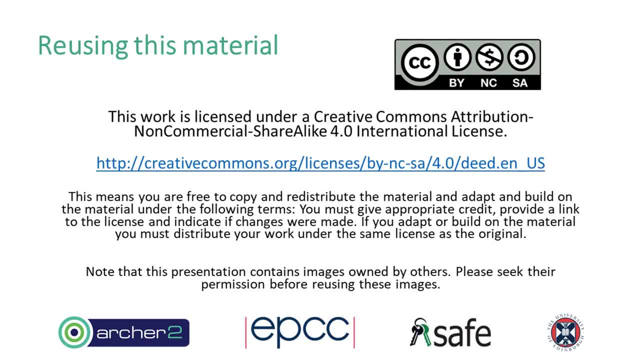 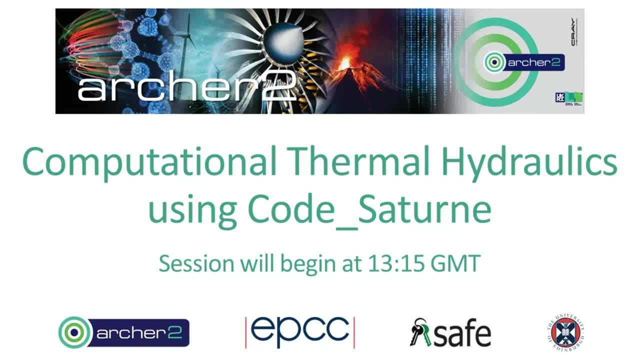 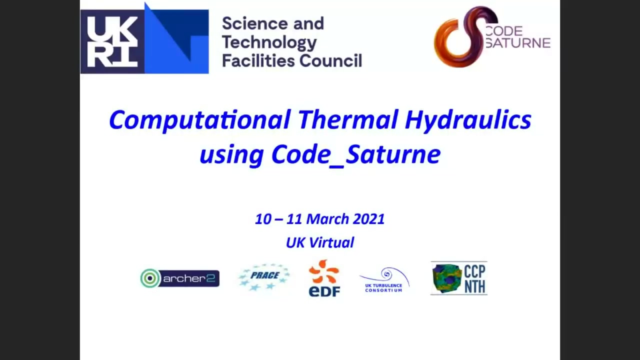 Okay, good afternoon all. So thank you for registering for the course and for attending it. So I'm going to give you a short introduction. So I'll move from these slides with the title and to a short welcome presentation. So here we are. So the course is called Computation. 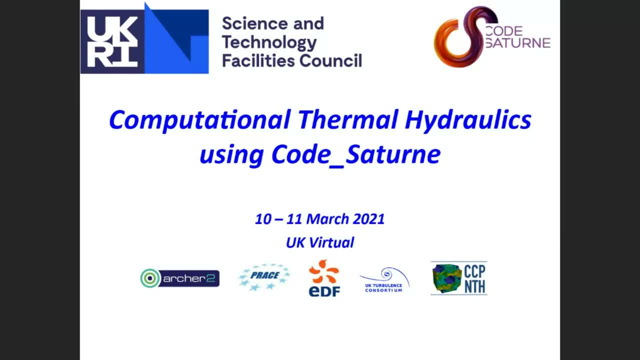 Thermal Hydraulics using CodeSaturn. So we are going to explain what the steps are to be able to run some simulation using CodeSaturn- So a part of the course is run on a virtual machine or a local machine- And some tutorials The last one from today is going to give you. 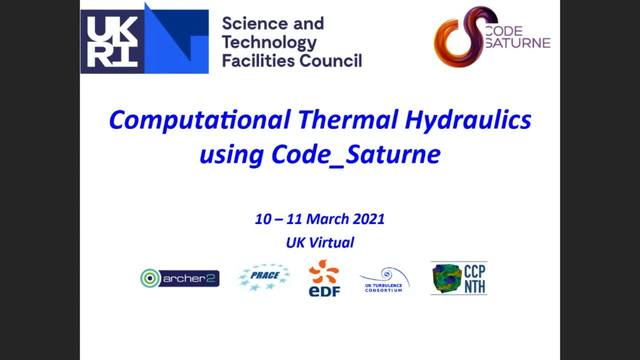 the chance to use ARCHER2, the UK national facility hosted by EPCC in Edinburgh, And you're going to run a simulation overnight and post-process the results tomorrow and then run another tutorial With more features of the course. So I'll first give you a very, very quick overview. 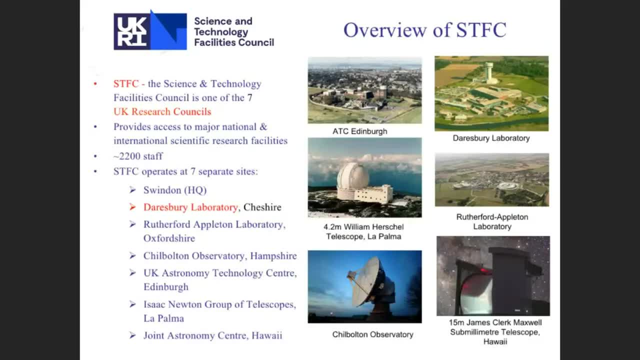 about what STFC is. We've got three tutors from STFC- Stefano Rolfo, Wei Wang and myself- And Juan Uribe is from EDF Energy, So he gave a short introduction to EDF and what he's doing, what they do and what they use CodeSaturn for. We also have the support from EPCC and 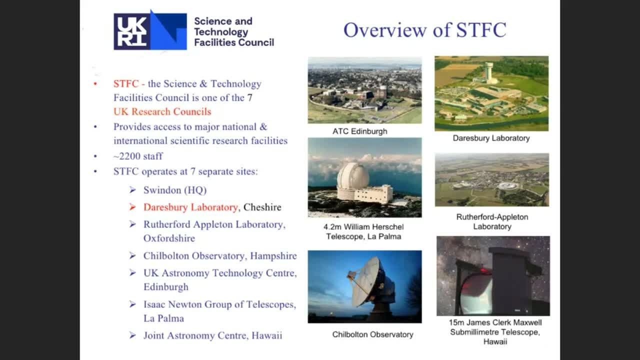 three persons, So Claire Barras, Juan Rodriguez Herrera and William Lucas, who is going to help us mainly for the part devoted to ARCHER2.. So STFC stands for the Science and Technology Facilities Council, So it's one of the councils of UKRI which has been set a couple of years. 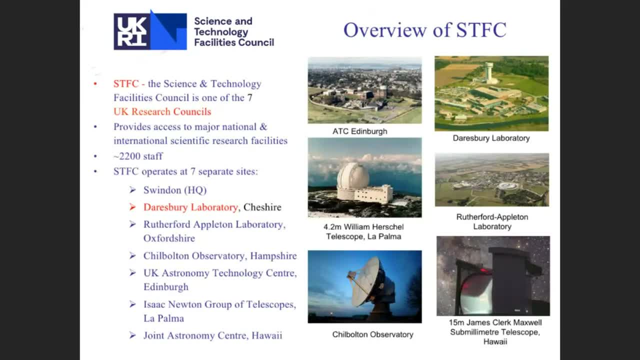 and so vegettaccess to the international scientific research facilities with about over 2,000 staff, And STFC operates seven separate sites. The three of them are all itezaccedu. Thank you, Prince, Great Thank you. Thank you. 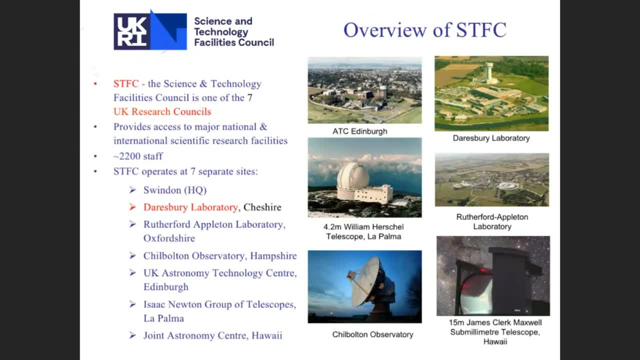 Thank you, way, Stefano and I are located at the D'Asbury laboratory, which is that's really being between Manchester and Liverpool, just to give you an idea, for people might not be familiar with the UK geography, and so we always also have other facilities like, and I know, a telescope in. 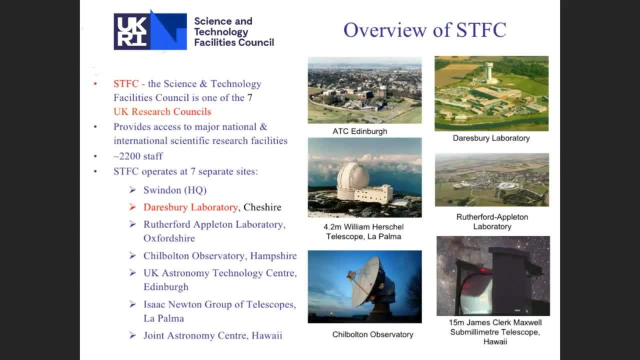 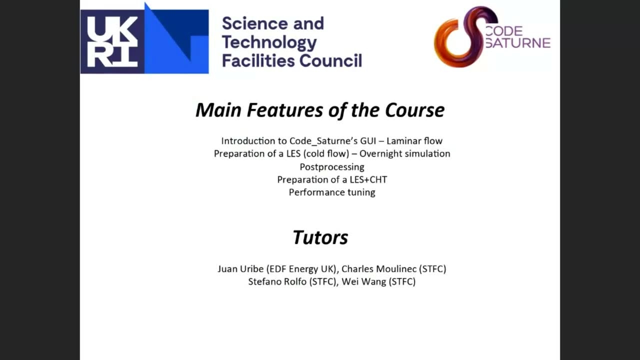 Hawaii, which is probably a little bit more fancy than D'Asbury. so, concerning the course itself, here are the the main features. so we are going to go step by step. you know, first working on the virtual machine or your local computers. you've got got such an installed on it, so the idea is: 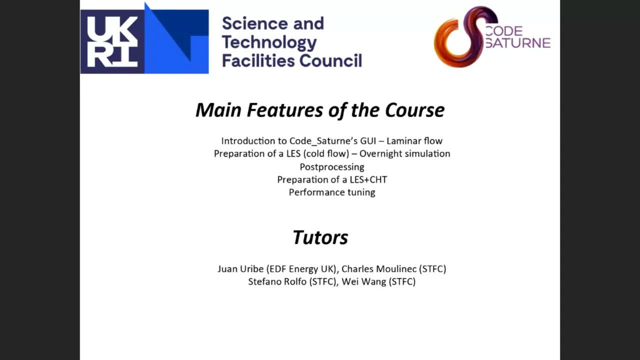 for you to get familiar to the graphical user interface. and we, for this course we are running, going to run the same test case in different working conditions. so the test case is about a flow in a bundle of tubes, so that kind of flow. you can find this type of configuration in heat exchanger exchangers for instance. so the first tutorial is: 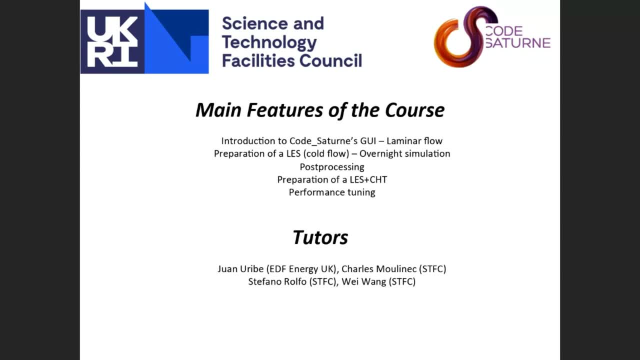 about laminar flow with different type of meshes. then later in the afternoon- this is actually the highlight of this course- is to run an advanced turbulence modeling simulation based on larger dissimulation, and so the this type of simulations are quite costly, but because of the power we get, having access to Archer 2, it's possible to. 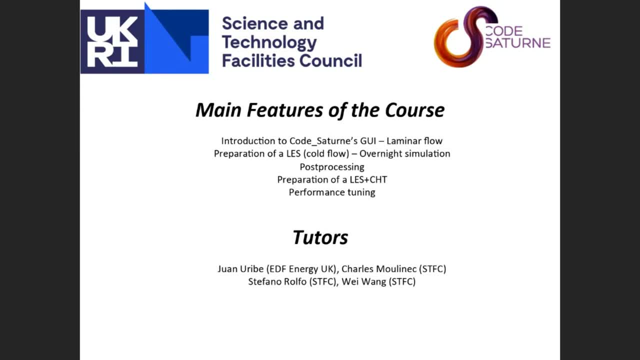 run an overnight simulation and and to to be able to capture most of the feature of the flow. so tomorrow there's going to be some post-processing session to analyze a bit the the results of the overnight simulation and then another feature of the code is going to be looked at which is based on internal coupling and more. 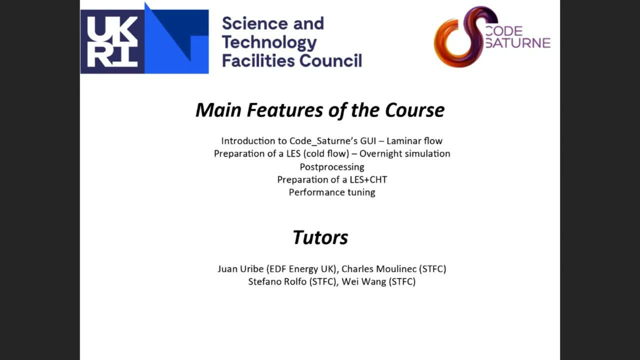 physics going to be added to the case with larger dissimulation and conjugate heat transfer. and finally, because we got access to a super computer, we are going to have a short tutorial about how to tune the code depending on the computer, depending on the configuration which is used, and so this is going to be the 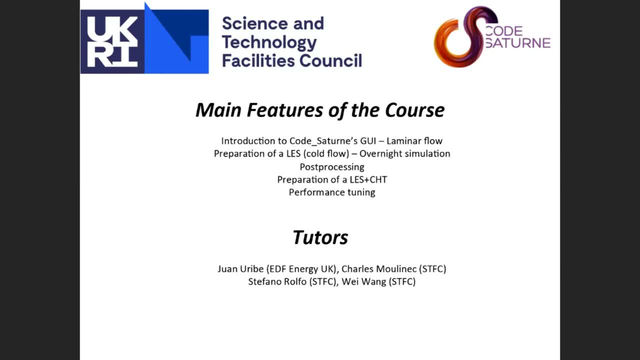 the last tutorial before the the end of the course, so I only mention here the tutors from uh who've got experience in a code Saturn, so that's one. or eBay myself, Stefano Rolfon, way one, and, as a I said before, I mean Claire Barras, William Lucas and Juan Rodriguez Herrera are 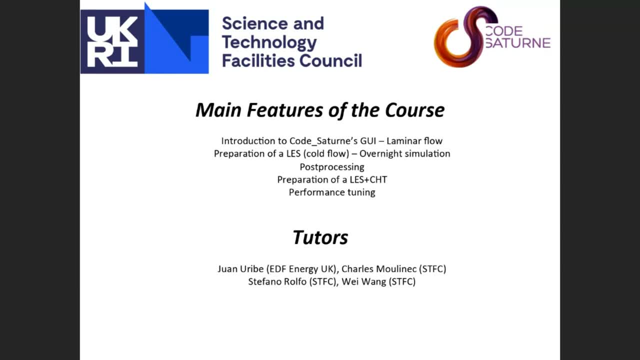 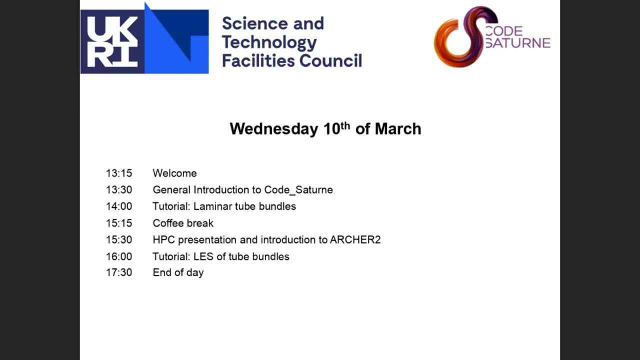 going to help us mainly for if we got problems setting up accounts or also to run on Archer 2. so here the the agenda of the course. so I mean, after this step, uh, Juan is going to give one way, is going to give a general introduction to code Saturn. then 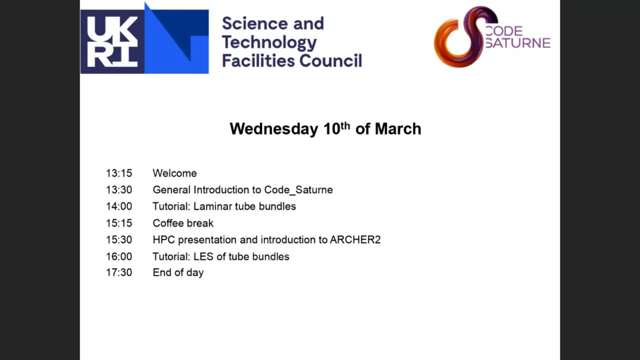 time for the first tutorial on the local or virtual machine, and after a coffee break I'll give a short presentation about HPC, for CFD mainly, and there's also a slide about describing how Archer 2 works. just to for a quick overview and then for the rest of the day you're going. 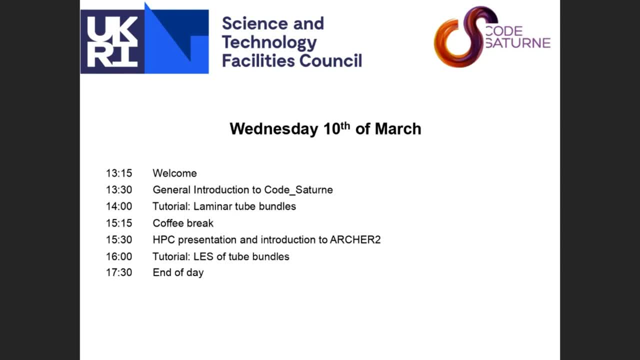 to work on the larger dissimulation of the set setup for a flow in a bunch of bundles. uh, hoping to submit a simulation overnight. so, through, thanks to praise, which is a partnership for Advanced Computing in Europe, and who's uh partially funding this. uh, this course, we've got access to 20 nodes of Archer 2, and each of the node being having 128. 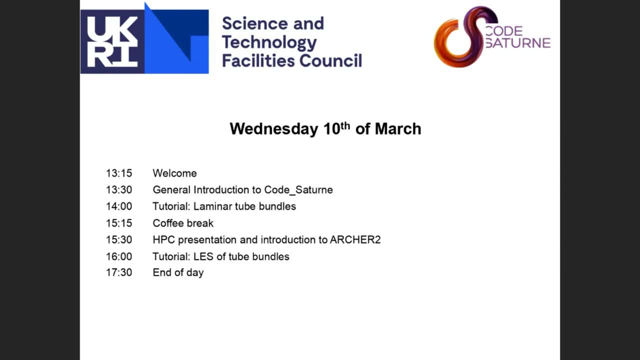 uh goals, so it's possible to run this uh relatively large overnight. so yeah, and tomorrow we post, process the results and to get access to most of the feature or to all the features of code Saturn, it's important to use user subroutines. so one way. 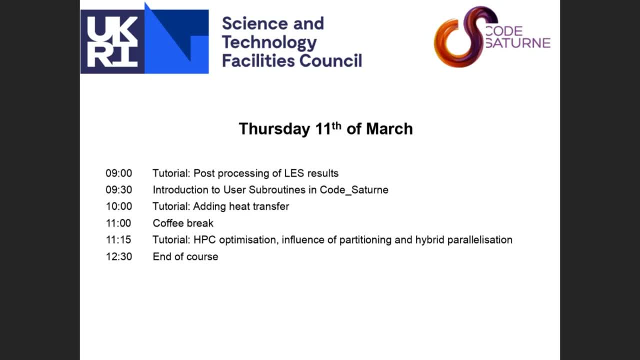 is going to introduce this, and then we will add uh conjugate hit살 to the largest simulation and show you other feature of the, of the software which is able to interpolate the solution to a different, to a mesh of a different size, and then to restart that from the simulation so which arose to to 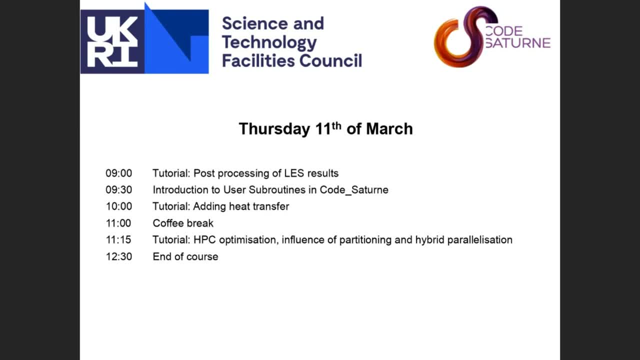 speed up some of the calculation and after the coffee break we we will talk more about HPC optimization and influence of the, the partitioning, to try to get the best of the machine we have access to. so I think I'm done here now. so have you got any questions at the moment? so the best is probably to raise. 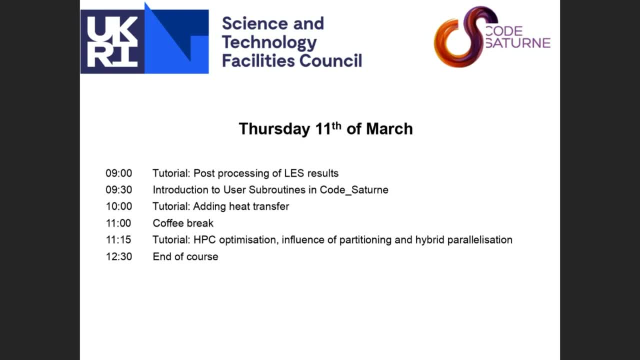 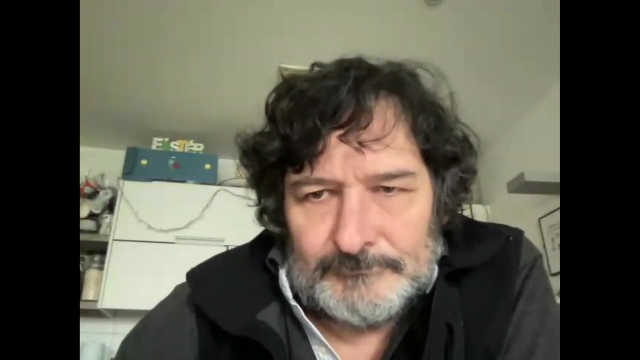 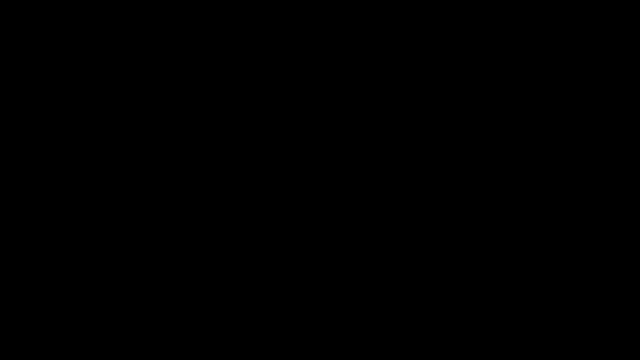 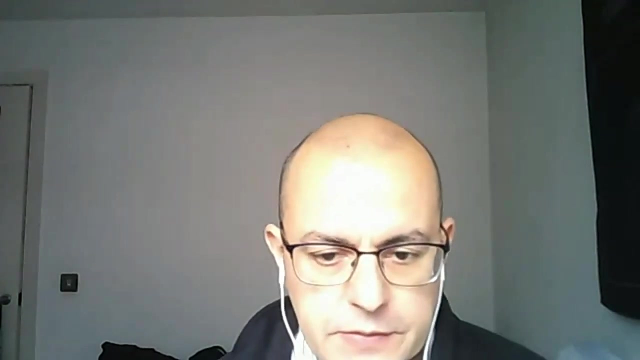 the hand if you want so. if not, we're about to start the course and I'm going to stop sharing the screen and and one is going to start the presentation on introducing code, such you. thank you, Charles. hello everybody. my name is Juan Uribe, as Charles said, and I work for EDF energy. I just sent a. 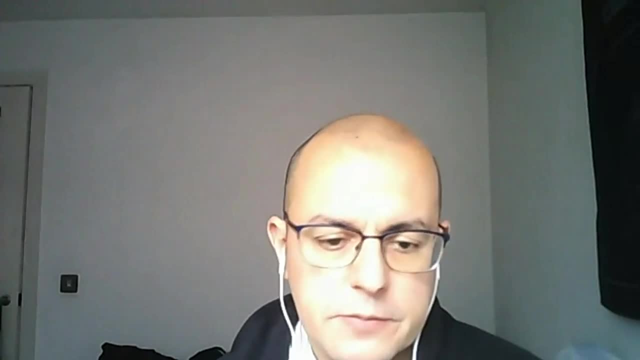 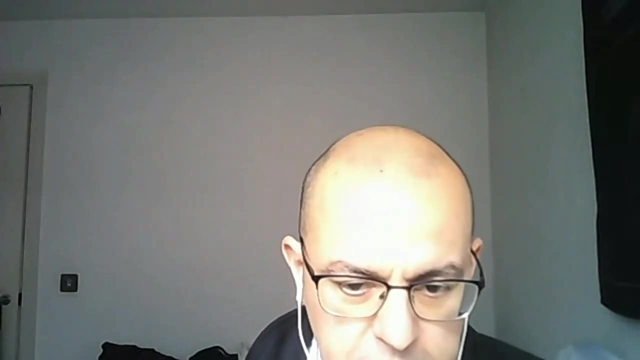 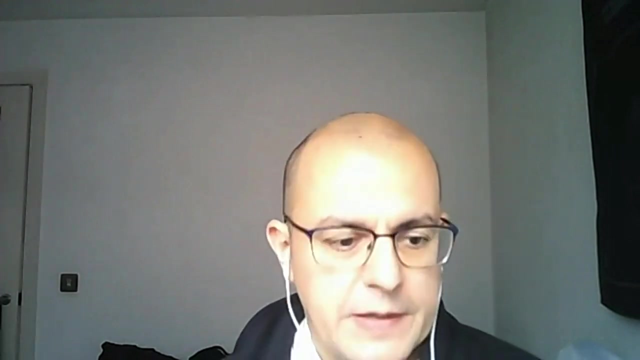 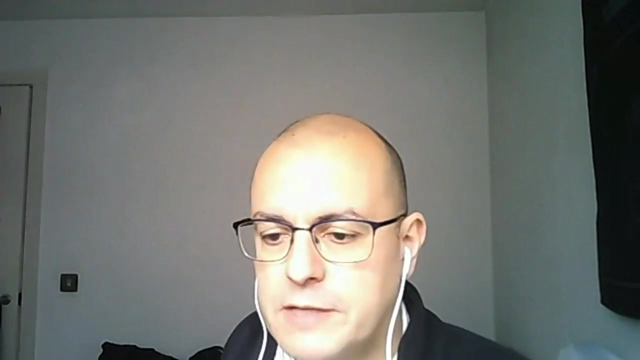 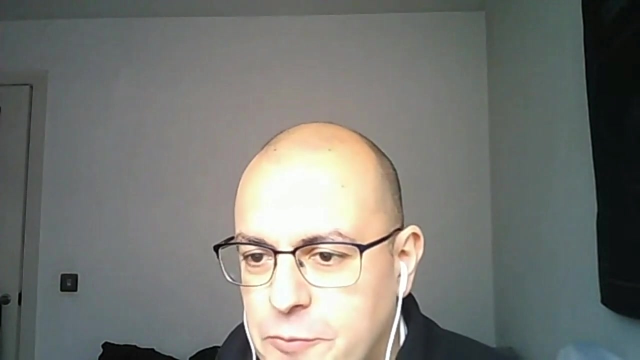 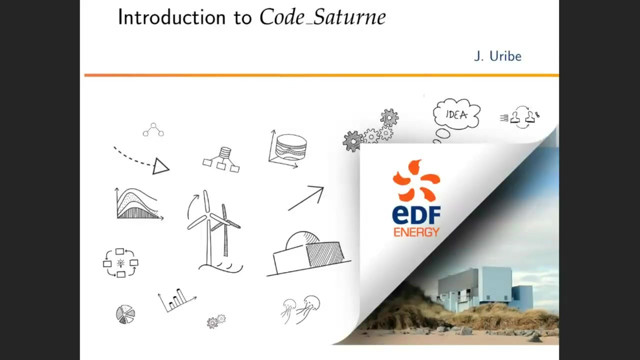 poll to make sure that you all have a working version of code Saturn before we start the course, and hopefully it seems like everybody has. yes, okay, good, good. so we're going to try this and see how it goes and I hope you can see this light. if you have any questions or if you have any problems, feel free to either put: 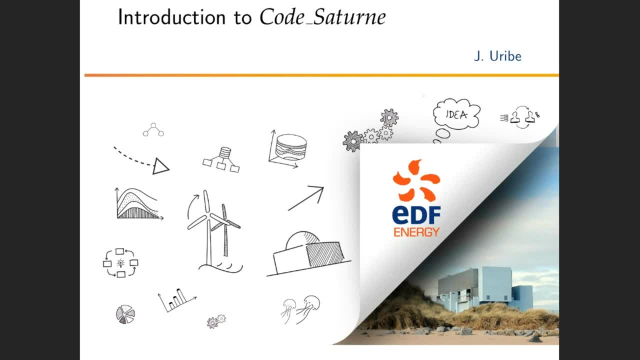 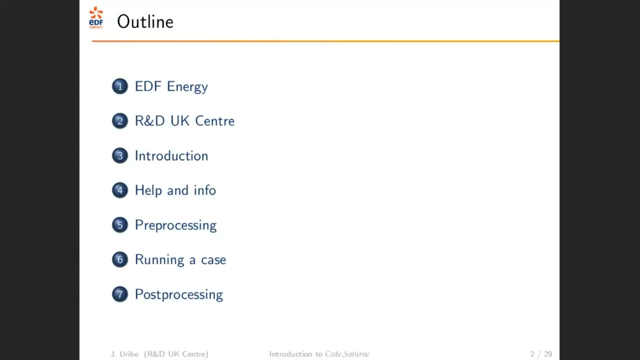 something in the chat or raise your hand and try to deal with that and, as I said, I work for EDF energy, so I'm going to just give you an overview of EDF first and then gonna introduce code Saturn, which is the software we're gonna use for this, for this course. give you the. 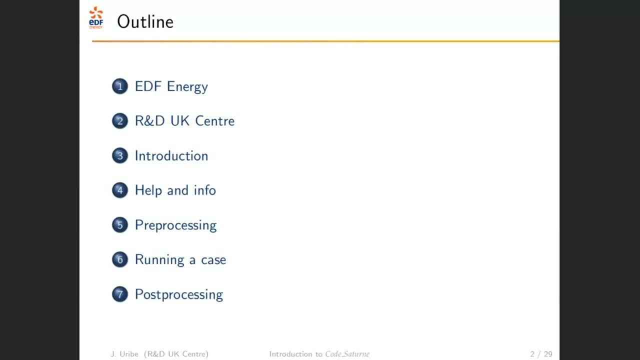 basic idea of how things work and and you're just basic steps for for running a very simple case, and then we'll go through the tutorials, which are designed for you to do it and on your own. so I'm not gonna do the tutorial with you. you we're just here to uh, we'll give you the material and the ideas that you follow the. 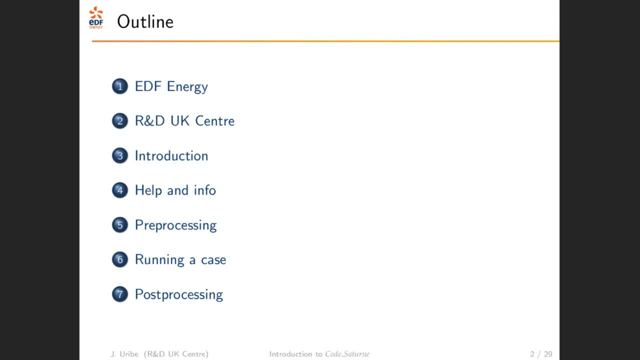 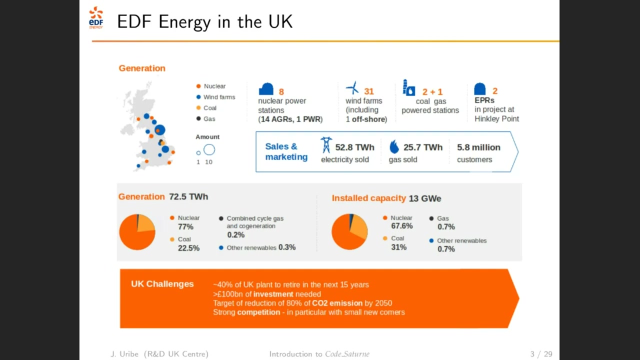 steps and the tutorials, and we're here to help you with any problems that you might have. um, so next slide. so edf energy is part of the edf group, which is a? uh electricity company. uh is a half owned by the french state. uh, edf energy is the. 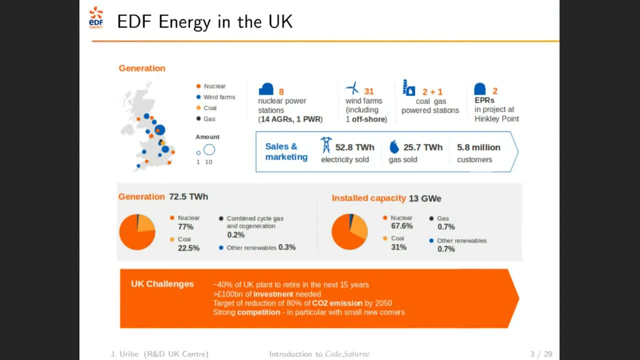 uk name for the company. we have um eight nuclear power stations at the moment. 14 of those are gas reactors and this one water reactor. we also have wind farms and we've just closed the coal stations that we had and we still have a gas station at the moment. 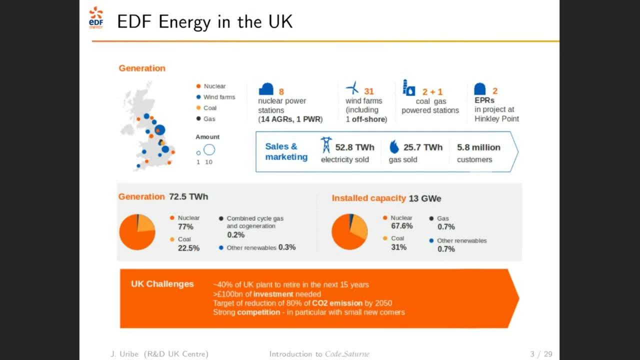 we're building, uh, two new reactors in hinckley point that should become online just as as the, as the old gas reactors are being switched off, and so we have. we have a series of problems in in in our business, uh, one of them obviously being used for energy transfer and fluid flow, and that's where we develop tools like uh. 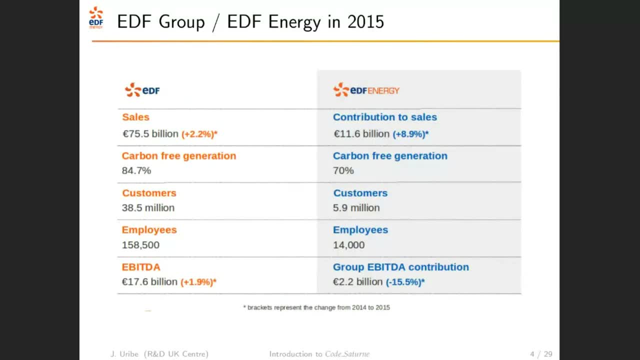 computational free dynamic codes, just uh, all of our problems. um, as i said before, we're part of the edf group, which is a much bigger entity than edf energy. here are some figures that are not really updated very recently, uh, but uh, we do have um. 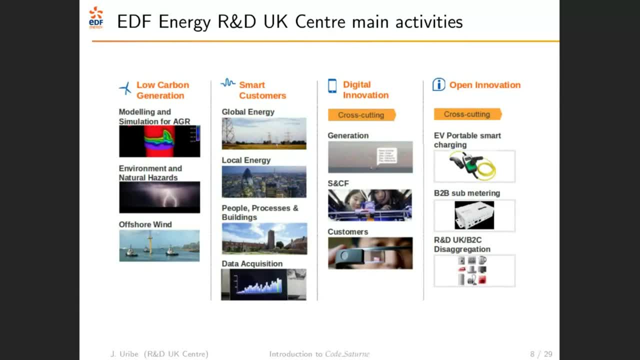 so um in the uk we have a research and development center which has four teams and part of the low current generation team which does modeling and simulation for our nuclear power plants. but we also have all sorts of uh research activities from the generation part and also from the customer side of the business. 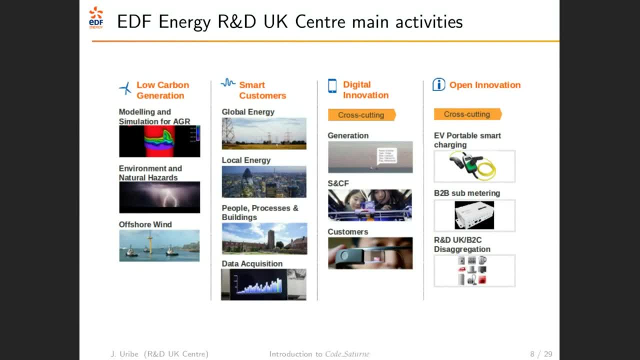 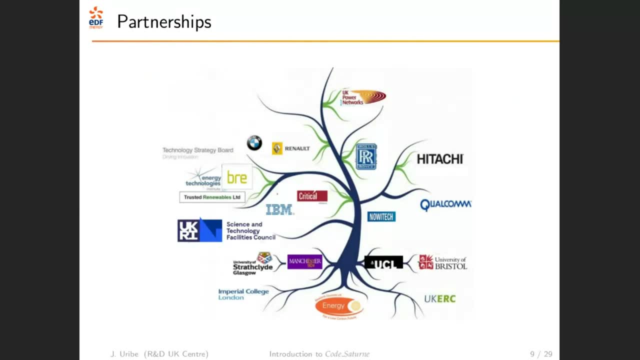 so things like grids and smart meters and things like that, and one of one of our main advantages of being here in the uk is that we have a very good set of partners. we work with very different universities and research centers and companies that share interests in in the same problems that we have, one of them being the science and 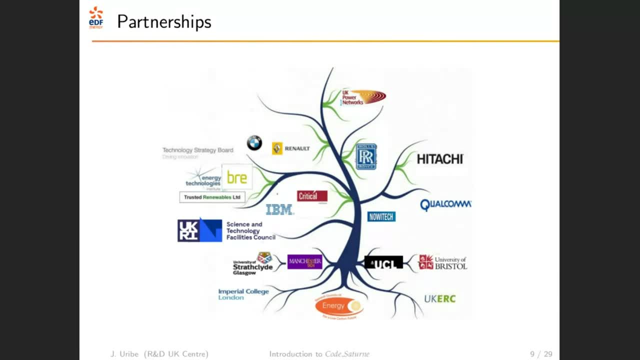 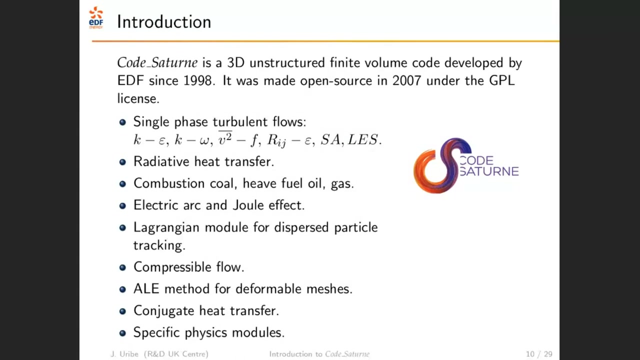 technology facilities council, where, when charles and stefano already work, so we have a very strong collaboration with them, and we also have a very strong collaboration with the university of manchester, where i am based, actually in a joint research center with them, and so, um, that's, that's a very quick overview of edf and the company. uh, as i said before, we have 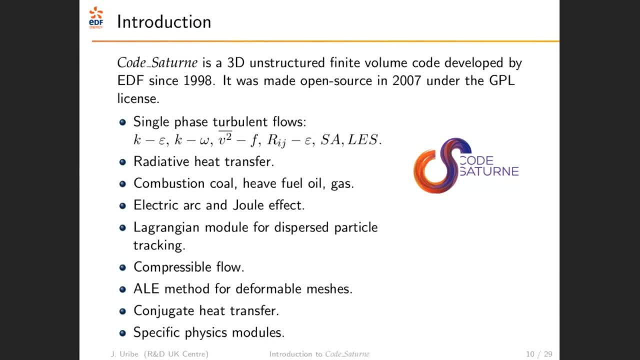 a series of tools and computational development, uh, to solve for the of the problems that we have with the patrick of the business costume is. one of them is a three-dimensional and constructive finite volume code for computational fluid dynamics. it's open source, as you probably know. 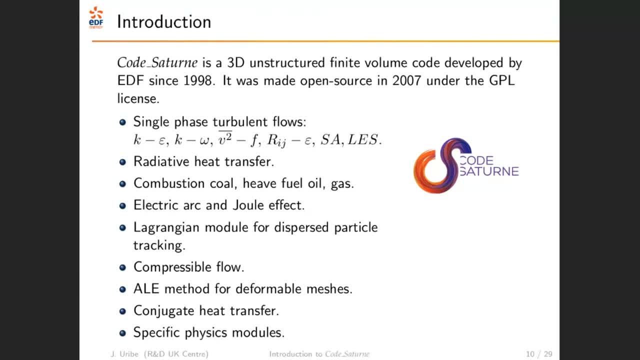 because you all seem to have it already working, so you can download it and use it, modify it and do anything you want with it. you can see all the source files and find out how everything is done in it. phase code has a very different types of turbulence models. It also has a series of modules. 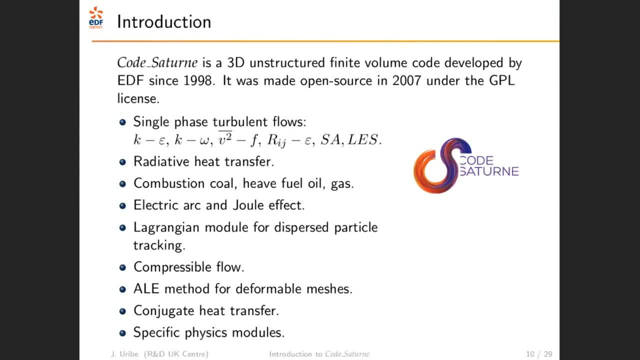 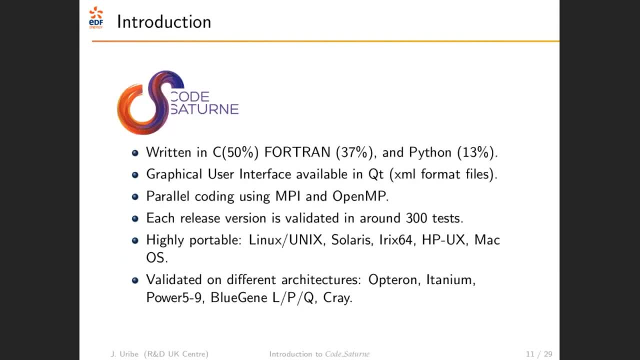 such as compressible combustions, electric arcs and conjugated transfer that we'll be using in later on in the course, And many other modules are being added as they require. The code is mainly written in C. Half of it is C, about 37% of it is Fortran and a little bit in Python. Originally the code was: 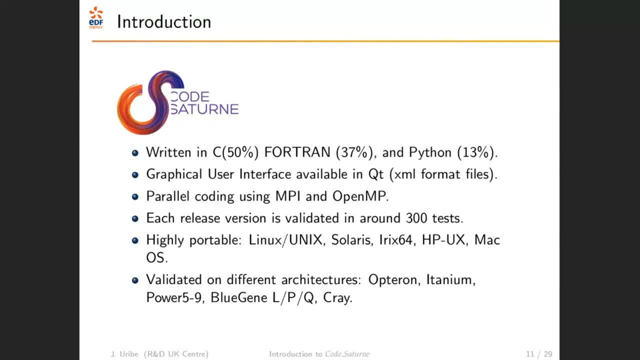 written all in Fortran and then it has been moving towards C very slowly in the past 20 years And we use Python mostly for the graphical interface and for the file manipulation. you will see that later in the tutorial. It has a graphical user interface. It uses Qt. 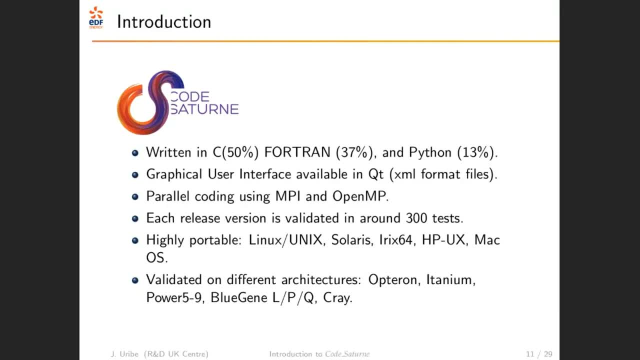 and uses an XML input file. We will go through that later. It's highly parallel. It uses APA and OpenMP as well, And one of the main advantages is that it's highly validated. As you can imagine, for the nuclear industry, we are required to be very strict in validation for the nuclear 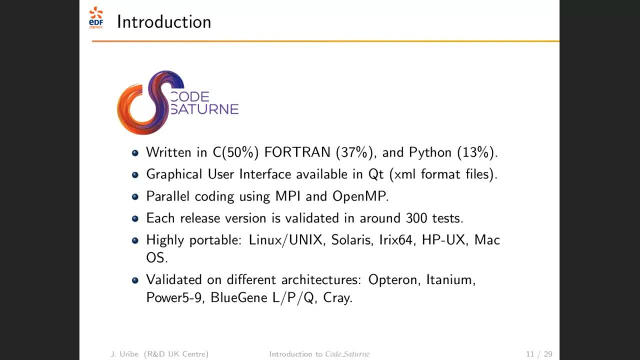 regulators, So they ask us to have a very strong validation verification suite, which is a, and it's run every time that something is changing the code. It's highly portable. You can pretty much install it almost anywhere, provided that you fulfill the prerequisites in any of these operating systems. 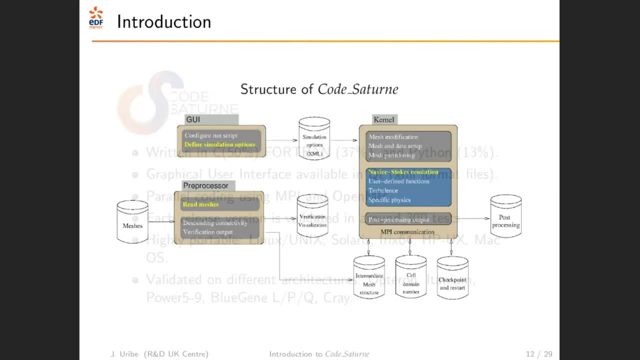 And we've tested it in many architectures, including the Cray system that you'll use later on today. We have here a description of the different parts of the code. We have a graphical interface which you will be using to create an input file, basically. 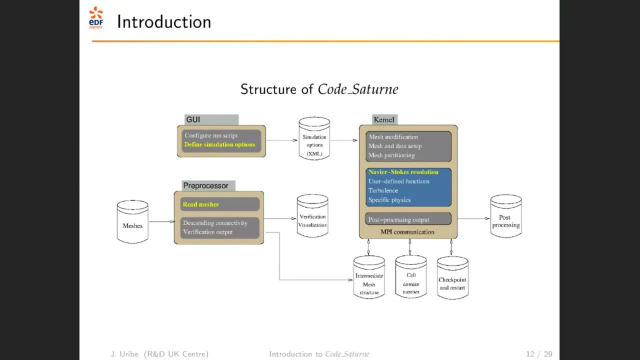 You have a preprocessor which will read a mesh. CodeSaturn doesn't have a mesh, a machine software, but it can read a very wide range of mesh formats. Once you have a supplier mesh to the code, it goes through the preprocessor. 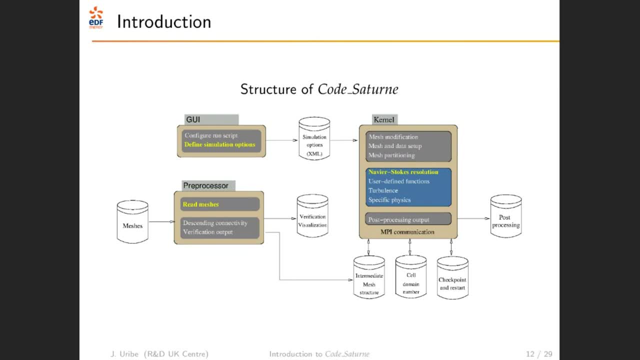 and create what is an intermediate mesh structure, That's, an internal file in which this mesh has been transformed into all the information that Saturn requires, like phase centers and normal vectors and connectivity and things like that that are not necessarily present in the mesh formats. 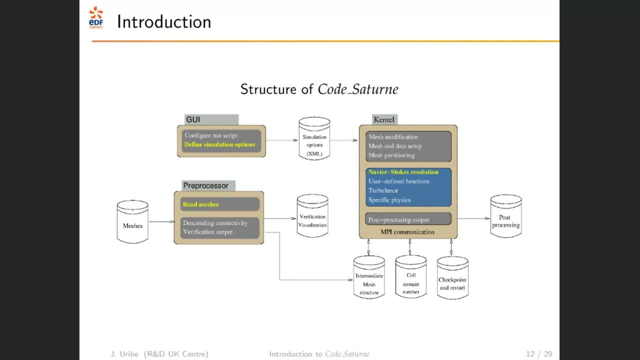 So once that translation is done, everything is passed to the kernel, which is basically when the bulk of the calculation takes place. It solves the equation that you are trying to solve And it creates an output. Concern doesn't have a post-processing utility either. It just relies on writing files that can. be read by other post-processing software. So once that translation is done, everything is passed to the kernel, which is basically when the bulk of the calculation takes place. It solves the equation that you are trying to solve. It doesn't have a post-processing utility either. It just relies on. 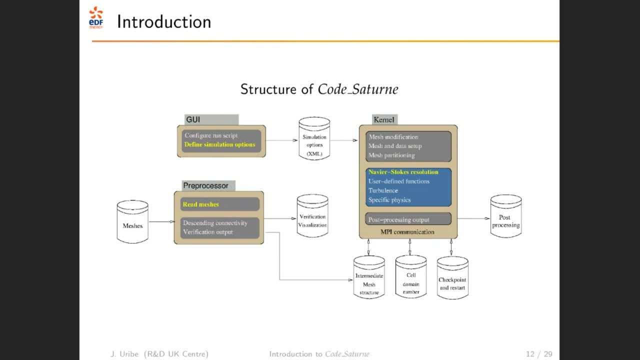 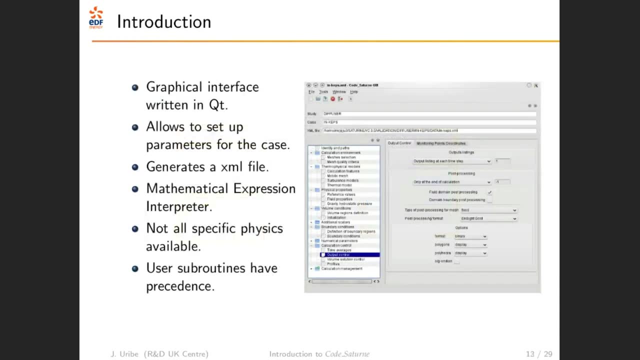 everything that you are trying to solve. It just relies on writing files that can be read by other post-processing software. We will be using ParallelView, which is also open source visualization software, So the graphical interface is a very simple thing really. It's supposed to guide you through the 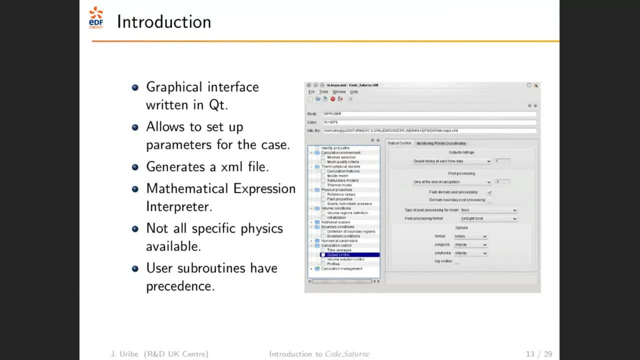 different pages. So the graphical interface is a very simple thing really. It's supposed to guide you through the different pages. So the graphical interface is a very simple thing really. It's supposed to guide you through the getting going lines, Or you can see in this picture on the left hand: 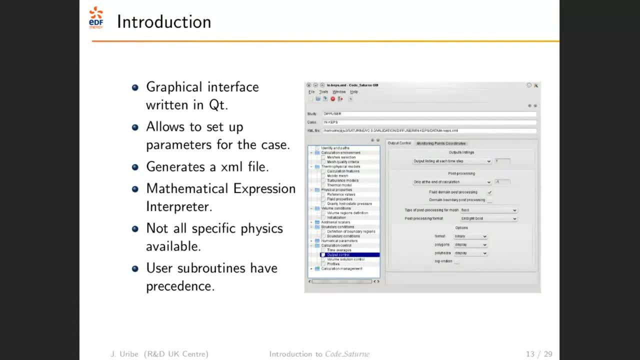 side. all of this titles refer to a page where you good going and select values or input values for the different things that you need to do during the setup. Anybody that is familiar with computational dynamics know that there is a lot of different options that you can choose. 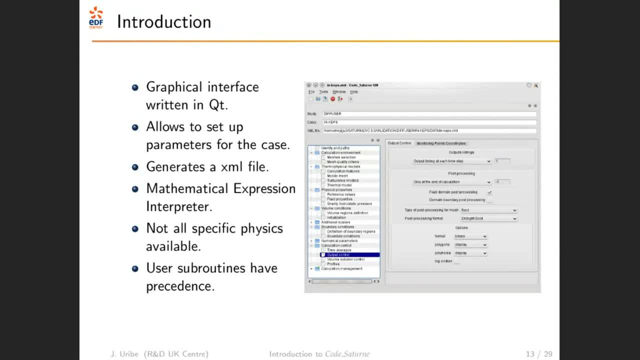 So in that sense it's not very different to any other computational free dynamic software. At the end, when you finish doing all of that, you will save the file, but it will be taken as an input for the calculation. It has a very basic mathematical expression. 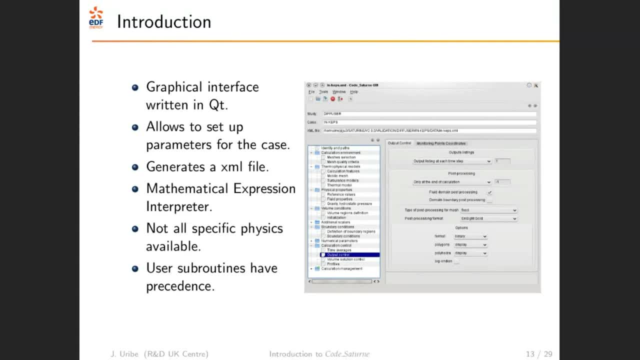 interpreter, which you can introduce formulas for things like density as function of temperature, for example, or some formulas for boundary conditions and things like that. Not everything is available on the graphical interface. There's a lot of things that are only accessible by subroutines. so for us working with the subroutines, the use of subroutines or 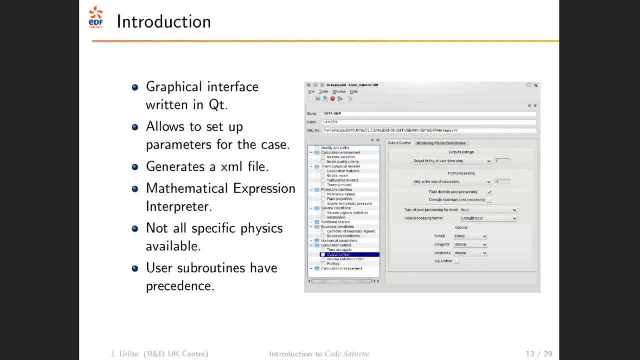 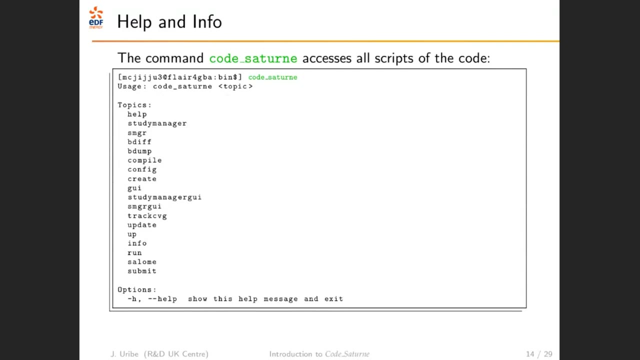 use functions is very common. This is a very normal thing to do and we'll go through those tomorrow. So there's a command called code Saturn that, once you start the software, you will have access to this command, and that's the one that pretty much allows you to do anything related to code Saturn. 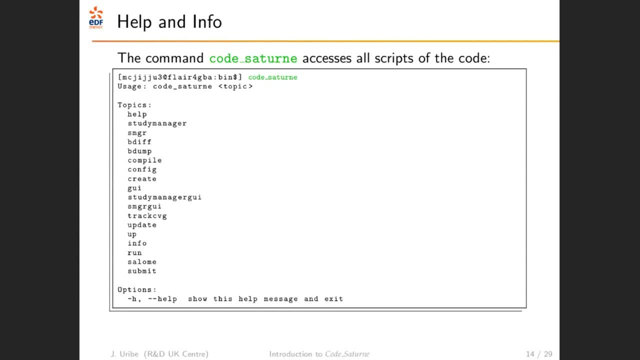 It can start the graphical interface, it can run the code, it can do the compilation, it can create your environment, your files, it can give you information about your installation and it also has what we call a study manager, which is what we use for the validation of. 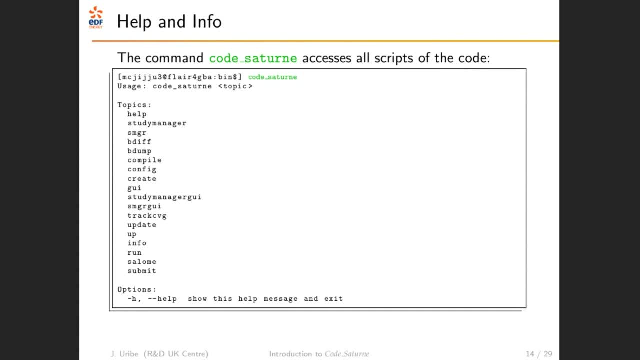 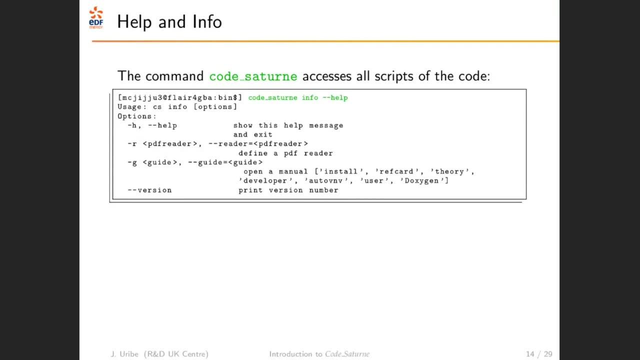 verification, which allows you to run a large set of phases almost automatically. The first thing that you need to know is how to get information and help, obviously, So if you type minus, minus, help for each of the comments in the previous slides, you get the help for that. 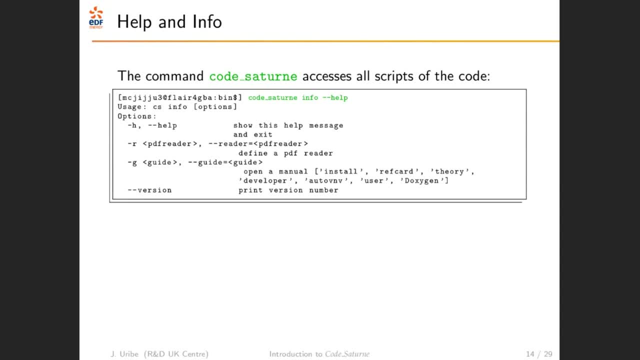 particular command. So in this case, in this example, if you type code Saturn, info minus, minus help, it will show you what options do you have for the information sub command, Which means that you can either select what type of guide you want or you can define a PDF reader. 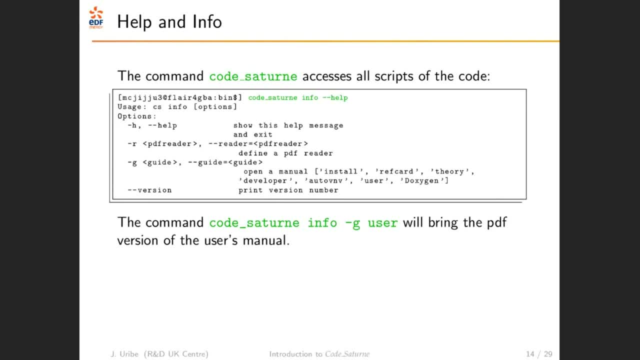 or you can just print the version number of the code that you're using. So, for example, code Saturn info minus g. user will bring the the user manual. You can have the user manual, the installation manual, the some developers guide and how to validation and verification as well. 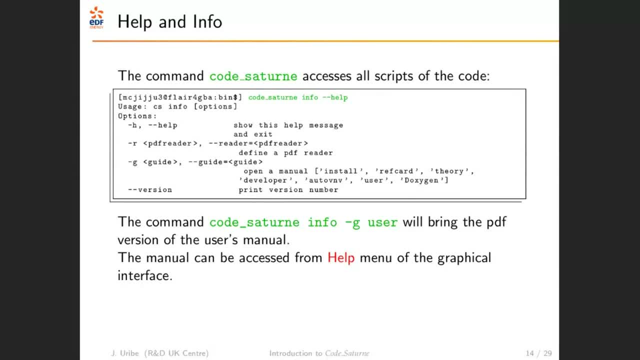 So there you have it. Hi, everyone, Don't think we can hear you. It has the morface. If this is stopped correctly, you will get the same pdf files as displayed here. There's an email support for all things related to CodeSaturn from EDF, but obviously the support is given without any warranty, as there's no. 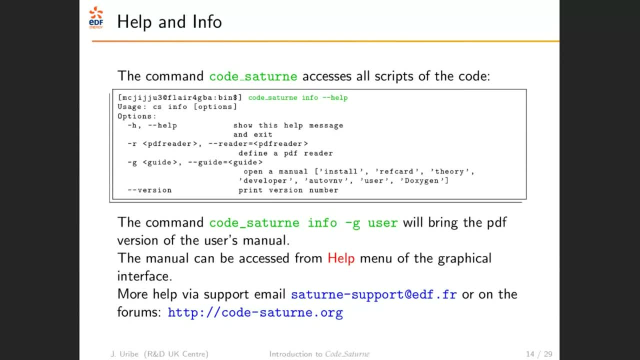 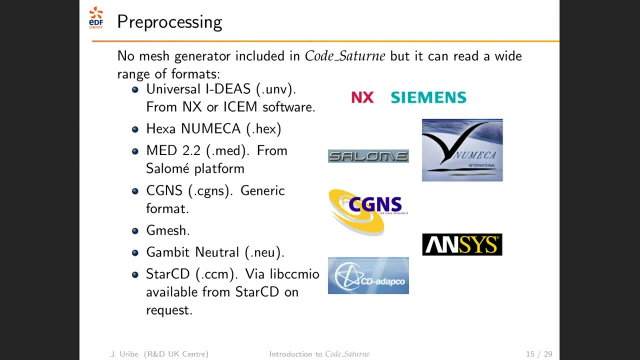 contractual agreement to do that. But there's a big forum in the web where you can find a lot of answers to most common problems, or you can contact the development team directly there and they'll give you the solution to whatever problem you may have. So I mentioned before, there's no mesh generator in CodeSaturn. 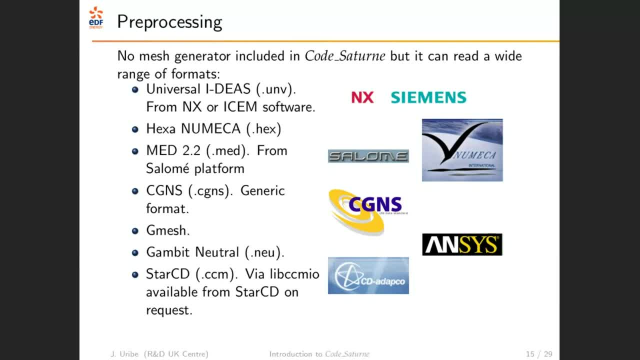 EDF has its own open source platform called Salome, which has a CAD and a mesh generator and a post-processing software. CodeSaturn can be installed within Salome, but that's an extra procedure that is not generally done. But there are also many other types of mesh files that we can read. Some of them are here: 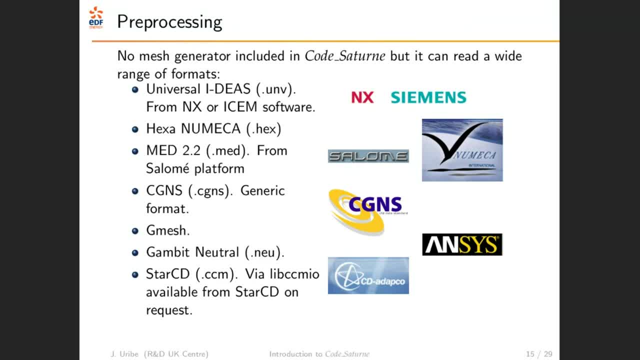 and we can read files from CGNS, for example, which is a very generic format that most of the mesh generator can export into. Mesh file is a particular format developed by EDF. as we are using this on the platform, We can also read CCM files, provided that you get a library from Siemens. 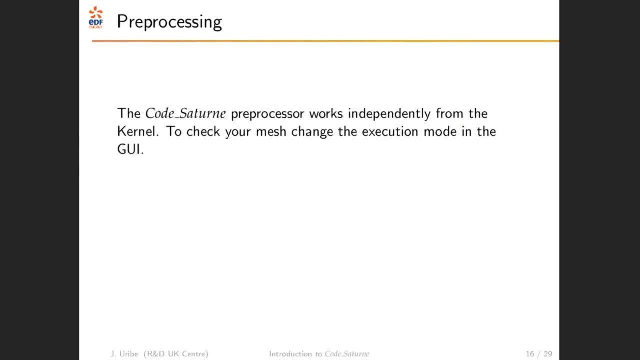 We can also read a lot of other files that are available on the platform. So, as I said before, when you have a mesh, there's a pre-processing stage that is done by the code and that is independent from the main kernel. You can run this separately without the needing to run. 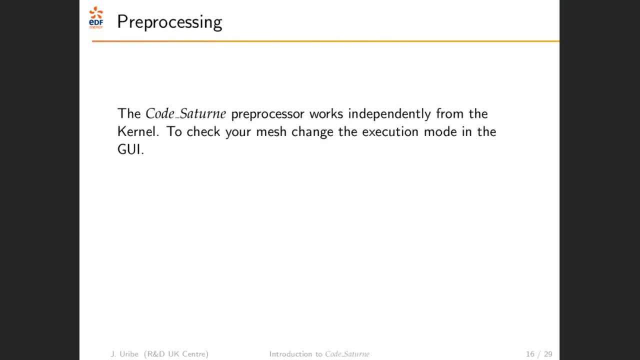 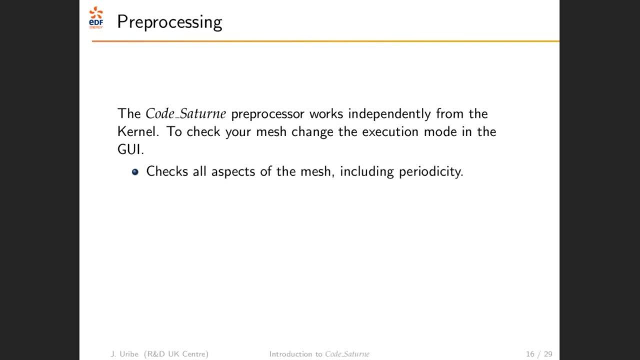 So you can just check your mesh before you start to run the whole code Going through your calculation. it will check that the mesh is valid. It will include the per-date boundaries if you set them up. It will show you what boundaries have been defined in the file, in the mesh file, And you can run a quality. 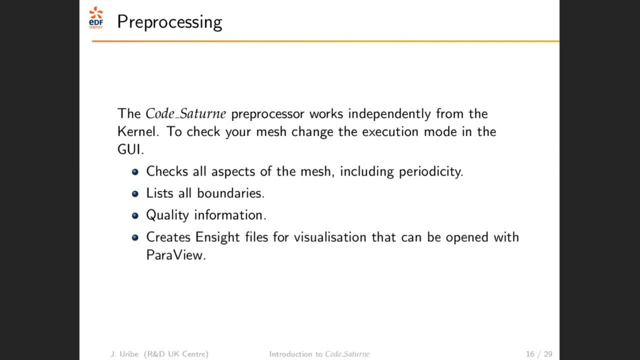 criteria and set up so that it will tell you the things like where the mesh highly distorted, or whether warp faces, or if there are any negative volumes, things like that, And then you can see all those results in ParallelView directly before starting your calculation. 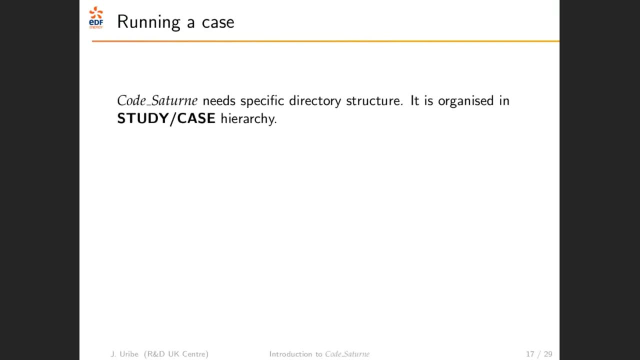 In terms of how to run a case. it's a bit more different than from other software And DieP detects by default a specific rule. forolan doesn't have the ability to cover the colors, the細pt and whatever responses it receives. 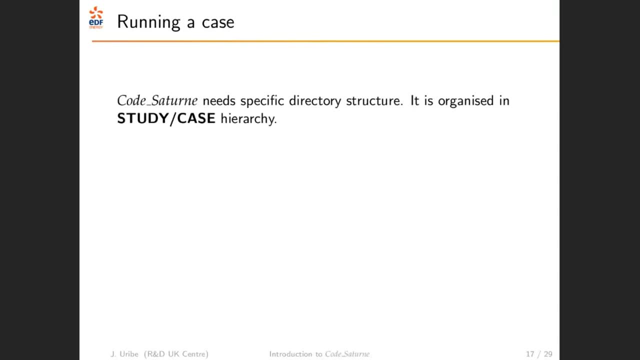 It expects to find by default a specific folder structure with the organization of the files and for the input files and the user subroutines. So we don't really, just because I was explaining you have different input files, is to use the code Saturn command to create this structure. 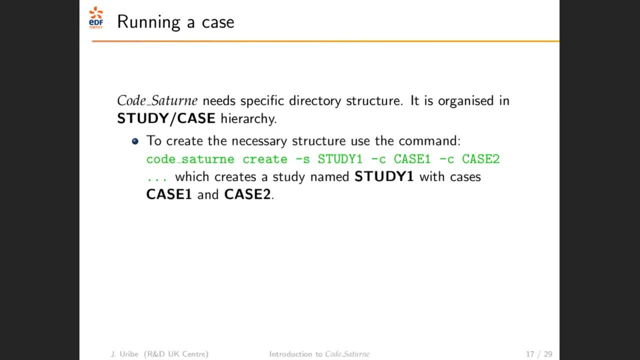 It's based on basically what we call an aesthetic case hierarchy, in which you have a folder which you can locate your study. say, for example, you're doing a pipe flow, then your study name would be pipe and inside each study you have different cases you can have. 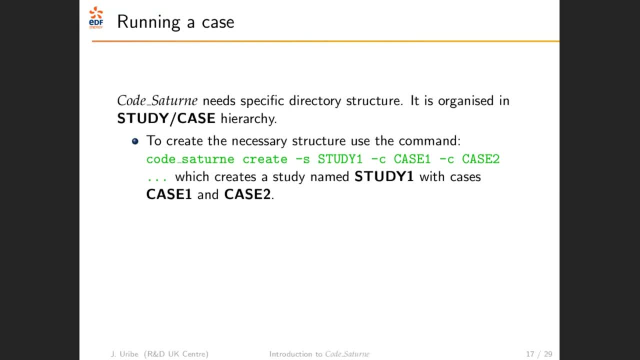 different boundary conditions, for example, or you can have different turbulence models or different meshes, so each one of those would be a different case. so to create a case you get, you can type this command: create code Saturn. create minus s will create a study and minus c will create a case. 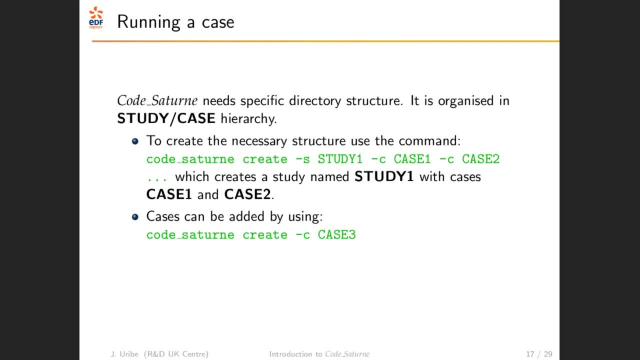 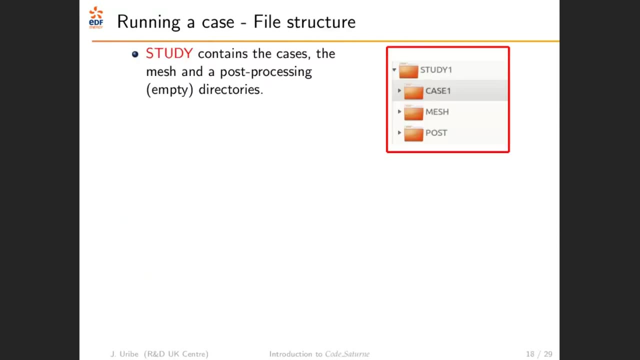 you can also create cases after you've created the study. you can also use minus c, create another case and it will just create a new folder. so it basically looks like this. so imagine that you have your your first study. in your first case, when you create this study, you have a mesh folder. when 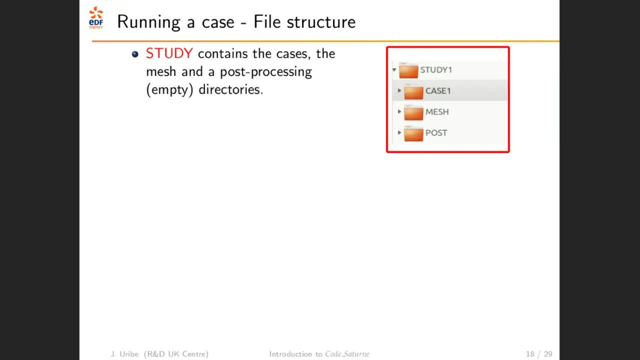 Saturn will look by default there to find any meshes that you have for the computation and it has a post-processing folder for you to do any, any scripts that you want to do for post-processing, for example. then the case file folder has will be created with this, this, this structure here that 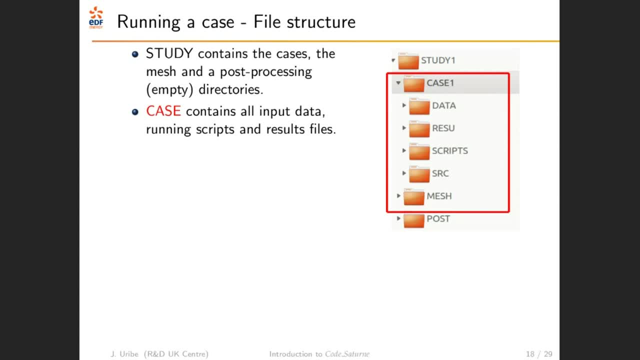 you see in the picture, you have data, result, scripts and SRC folders. the data folder has a script that will run the graphical interface that's the equivalent of typing code: Saturn GUI. it also has some reference files and where you can find keywords, things like thermal properties and databases and things like that. 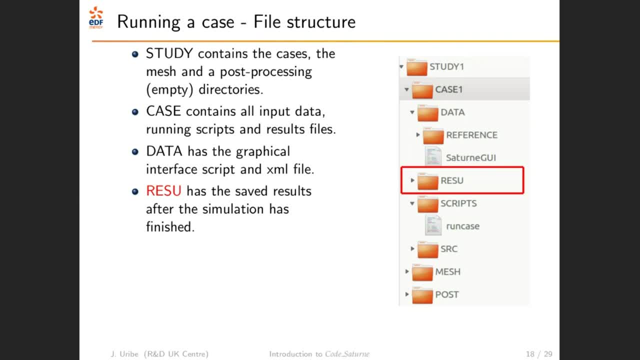 In the result file is where you're going to have the results after you've run a computation. So at the beginning it's an empty directory, but every time that you run any computation the results will be stored there by default, And the script directory has a file called run case, which is basically the equivalent. 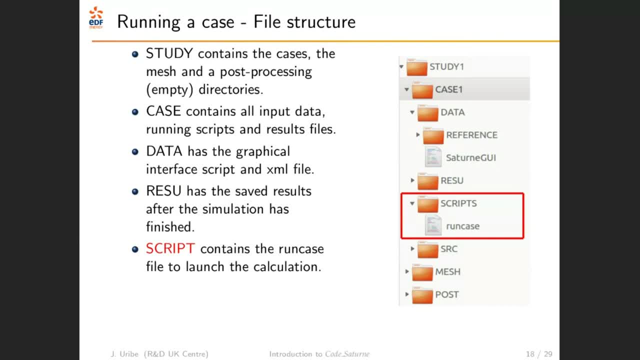 of clicking run on the graphical interface. We'll go through. why is that? later in the session when we go to the remote machine, You see, like that, this is an advantage. And finally, the src folder is where we're going to put all the subroutines that you want to modify. 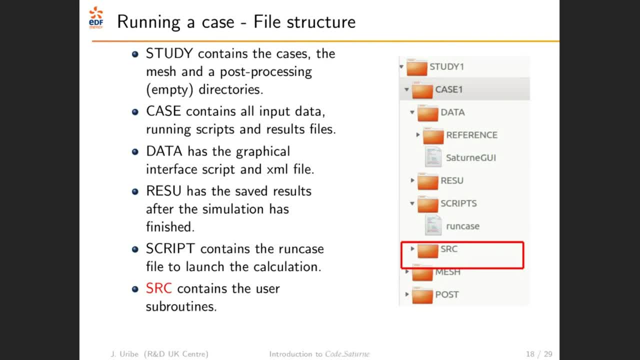 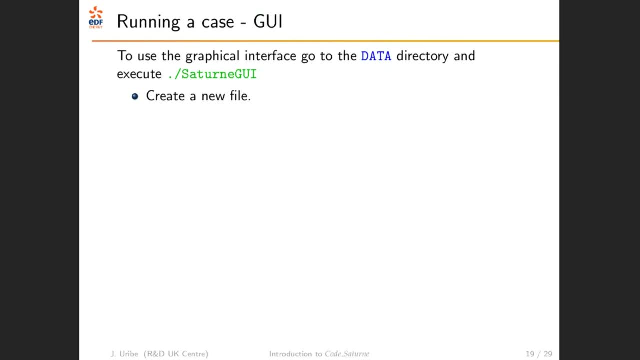 It has some examples for things that you can do with the subroutines. We'll go to that later as well. So the basic steps for running a case using the src folder. So the basic steps for running a case using the src folder. 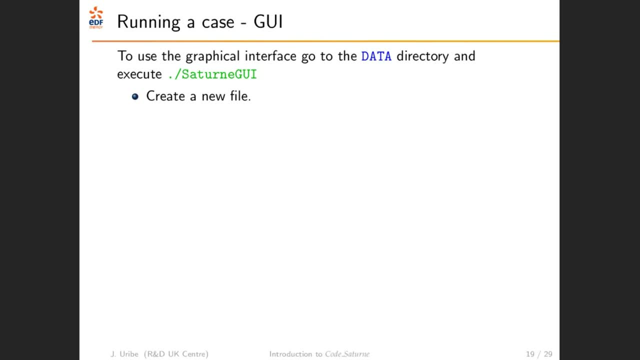 So the basic steps for running a case using the src folder. So the basic steps for running a case using the graphical interface is: first, after you've created this study case structure, you will go to the data directory and type chat gui. It will bring out the graphic interface which looks like: 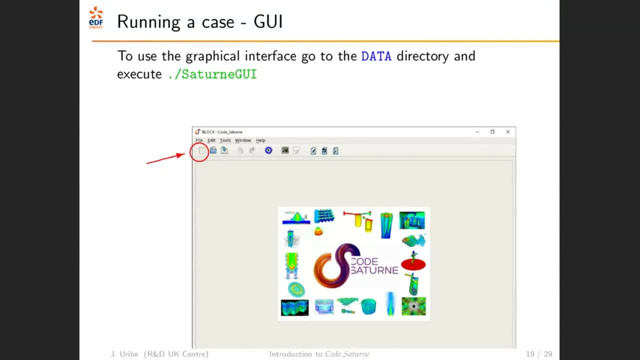 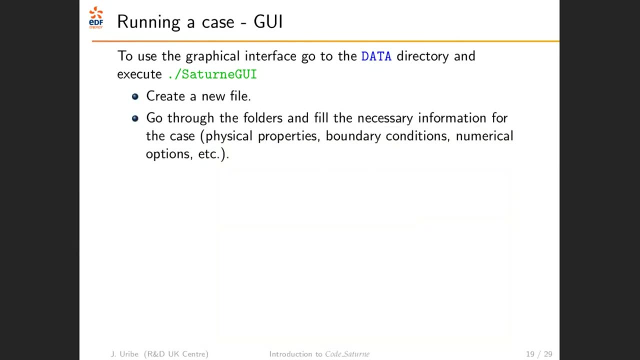 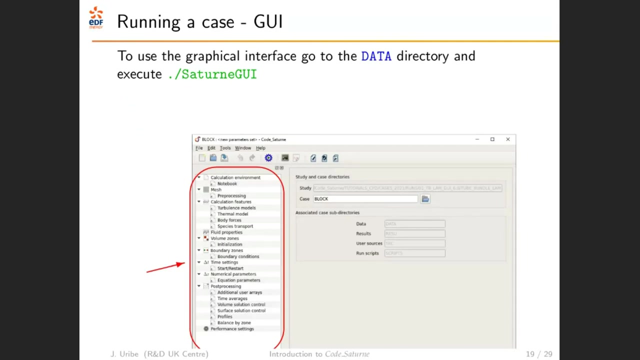 this. Then you just click on and have this logo at the beginning and an empty space. So when you create a new case, the new file button- it will give you a series of pages where you need to fill all the things that are required for a computation. So most of the things have a default value. 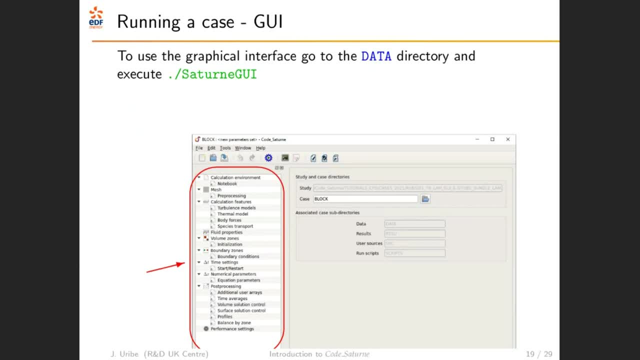 and it's up to the user to make sure that they are changed to whatever case is necessary. Obviously, the boundary conditions at the beginning are empty, So that's not. there's no default boundary conditions. You won't run until you put some boundary conditions and then some mesh file. 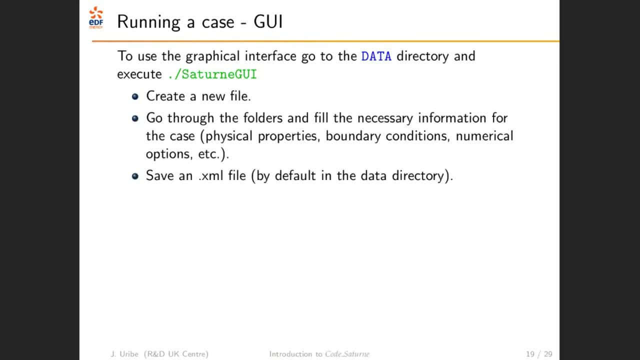 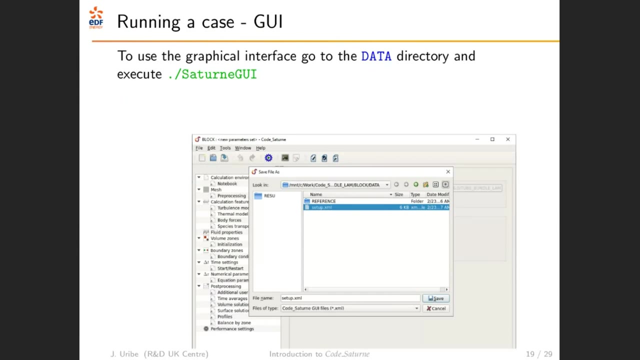 Most of the other pages have a default value. So once you go through all of those pages and you can save the file by default, if you just click save, it's gonna be called setupxml and it's gonna be saved in the inside. So this is the default file and you can save the file. 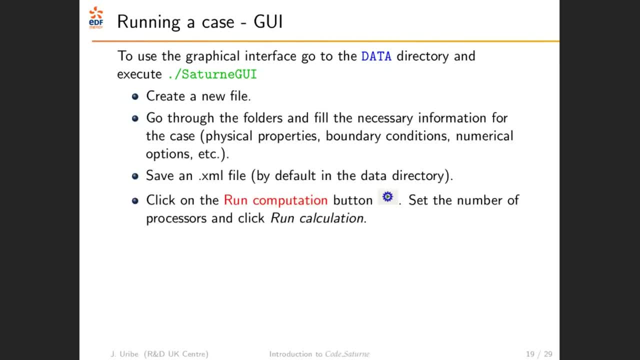 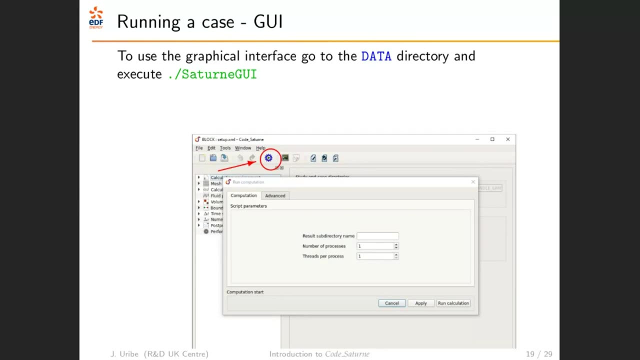 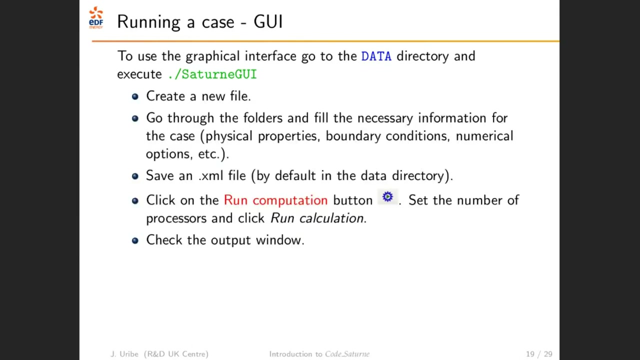 data and then you have this cogwheel play button, which is basically run. that would bring up this window in which you can set the number of processes that you want and the number of threads. if you have compiled this with OpenMP, so you can just click run calculation button and once you do that, there will be. 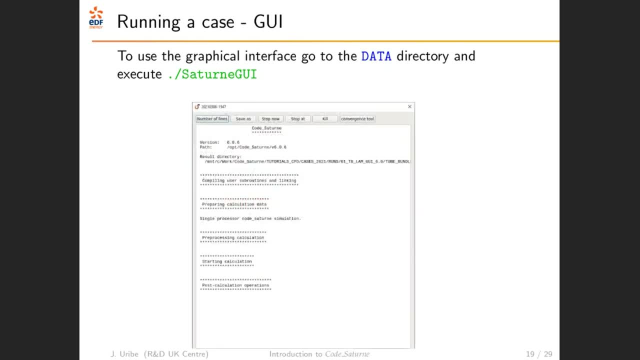 another new window that gives you some details about what's happening. so it will tell you which version of the code you're using and where is that version installed, and it will tell you what now your results are going to be, and then it will start printing things as the calculation goes along. so first step, if 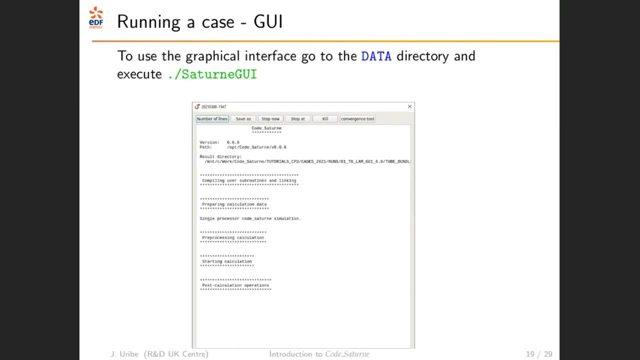 you have any subroutines, you would compile and think those subroutines. then it will copy all the necessary files, including the mesh and the input data. then it will call the preprocessor stage which would read the facts that the mess file and once all that is done you will start the calculation and then, at the 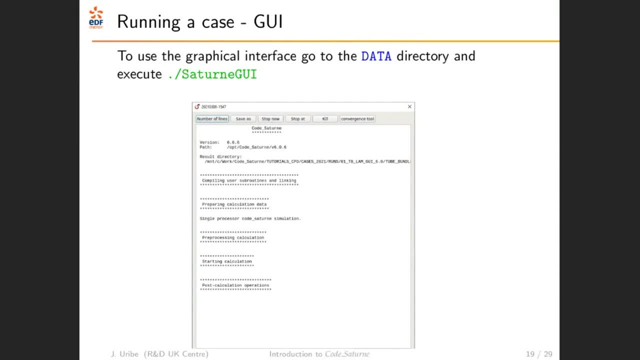 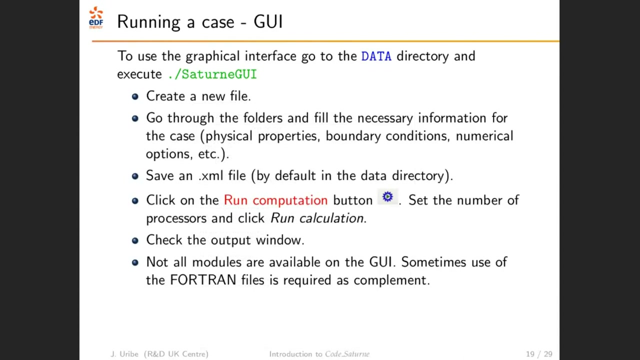 end you will just tell you that it's done some post calculation operations and finish, and you have some buttons at the top of this window that allows you to stop the calculation or kill it, and then also a convergence tool. as I said before, not all the modules are available on the graphical interface, so sometimes 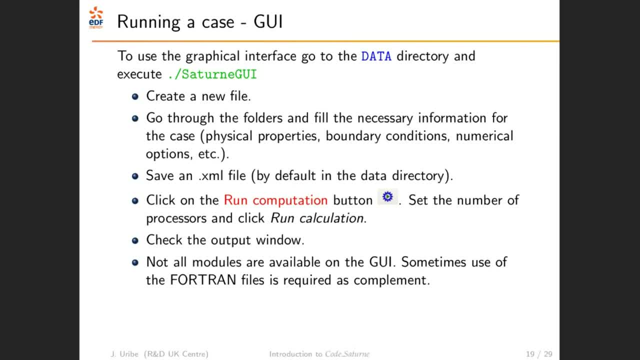 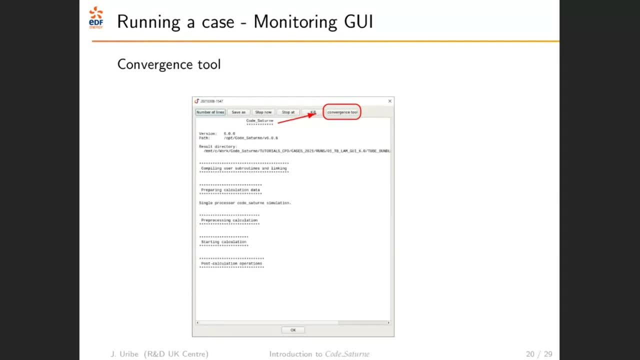 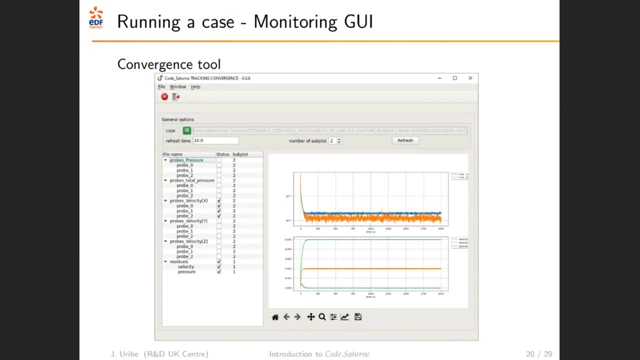 you need to use Fortran or C files for changing things that you may want to use. So the convergence tool, when you click here, it will show you, basically by default, it will show you a plot of the residuals of the equations that you're solving and if you 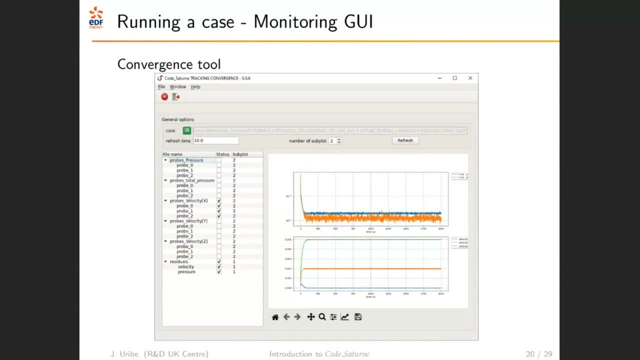 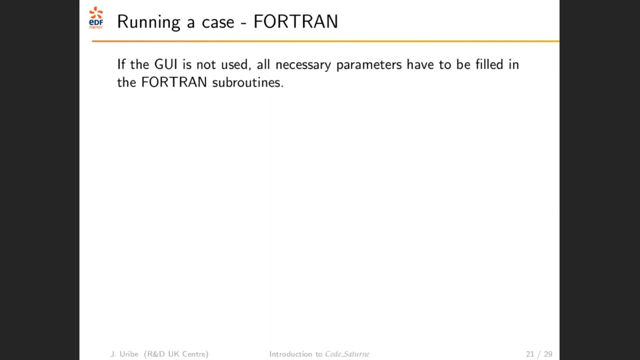 set up monitoring points. these are points that you select in the domain where you want to see the evolution of the variables. you can plot those too as the calculation goes along. So that's very convenient for knowing how things are behaving. So sometimes you need to use Fortran files or user subroutines. they could be also in. 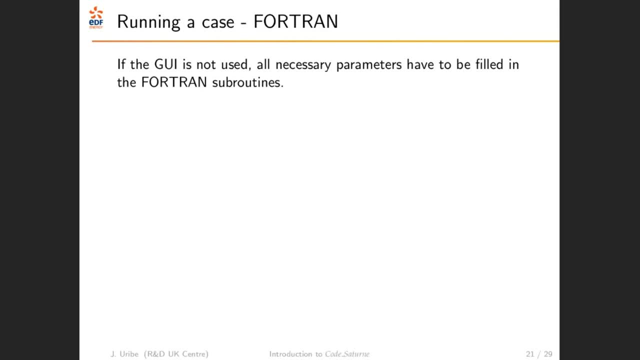 C as well, and in fact you don't need to use the graphical interface at all. you can run a complete calculation Only using the user subroutines. So obviously you need to be much more comfortable knowing the subroutines than the graphical. 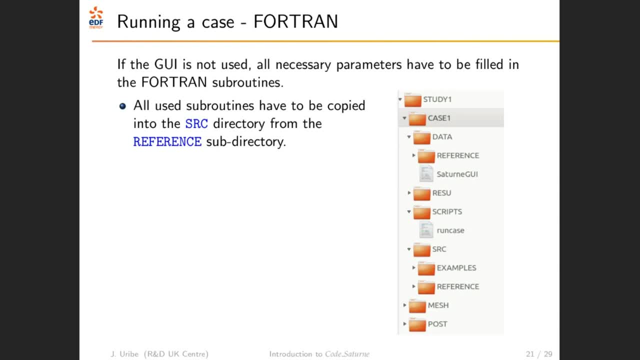 interface, but it is possible. If you want to do that, you can find in the SRC folder examples and reference files. So the reference file directory will have empty files And the examples will have the same files, but with some examples that you can use to. 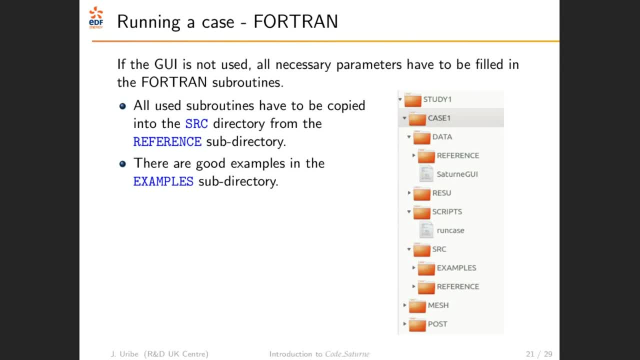 make inspiration, let's say, or copy-paste from there to whatever you want to do. You don't want to use the graphical interface. you need to have at least two different subroutines: the C is user parameters file and the C is user boundary conditions file. 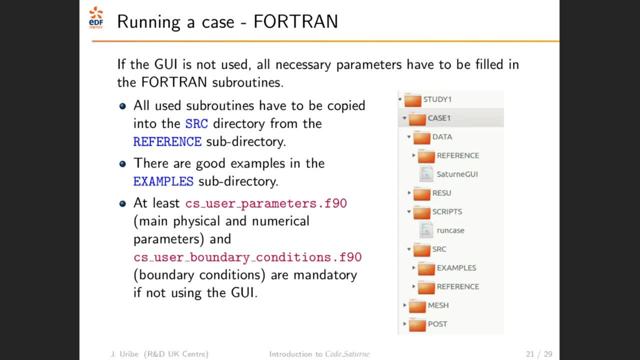 So that's very convenient, Thank you. So you need to. in your set C as user parameter files, you will define things like physical properties and numerical parameters like your time step and your number of time steps, and then your boundary conditions. you need to define the boundaries that will match the 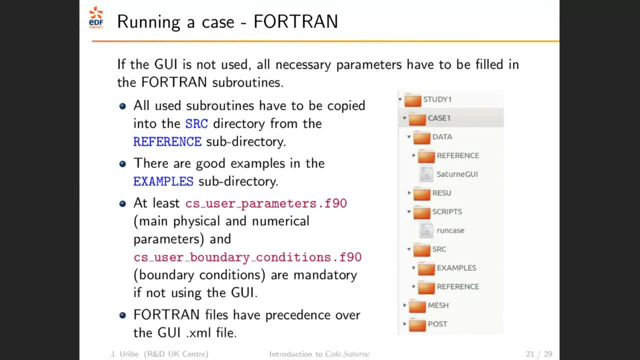 mesh that you're using for this case. Yeah, Thanks, Bye-bye. One thing that is important to know is that if you have the same value set up both in a subroutine and in a graphical interface, the value that you set up in a user subroutine will have precedence over the graphical interface. 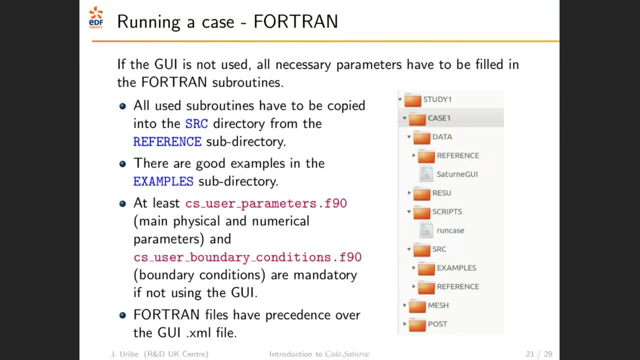 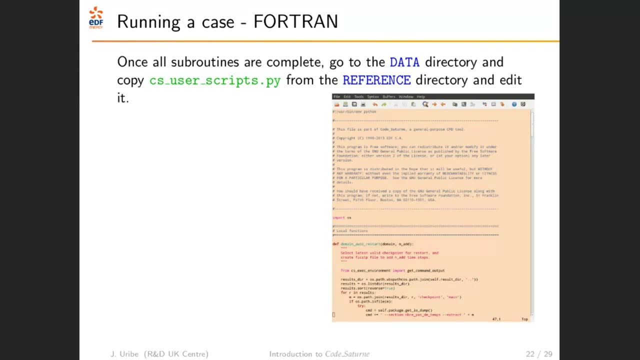 So if you have a value for the density in the graphical interface that is different from the one in the user subroutine, the one that you will be using will be the one in the user subroutine. So if you're not using graphical interface, you will also need to use a CSS user script. 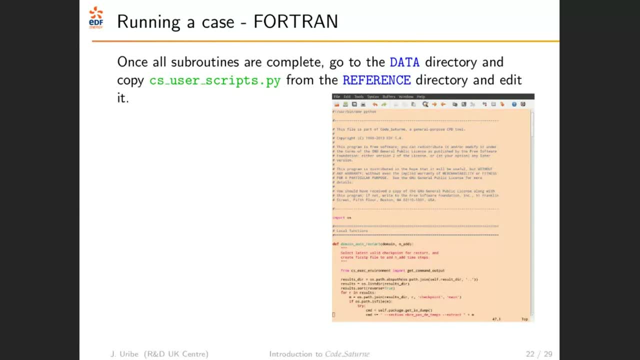 a Python file that will tell the code where to find the mesh file and where to do all the things that are optional, such as find a restart file Or do some sort of post-processing code, things like that, And that can be found in the data directory in the reference. 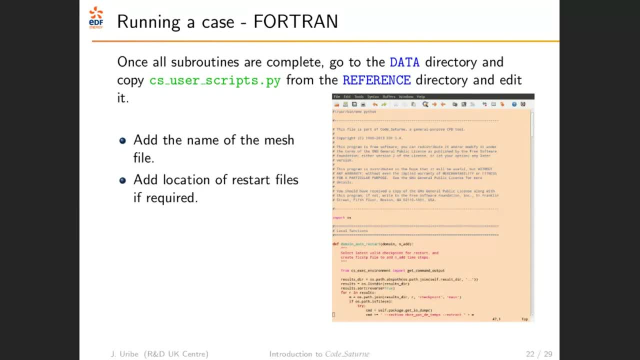 And we need it. if you don't use the graphical interface, The tutorials that we're going to do, we're not going to be using this, as we're going to create an XML file, even though we're going to have some subroutines later. 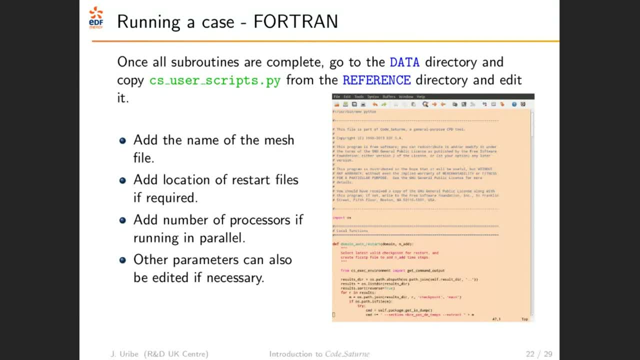 Once you have set up everything in your data directory and your subroutines directory, you can go to the scripts directory and run type: run case. As I said, this is the equivalent of clicking on the graphical interface, the run button. So if you don't have the graphical interface, that's how you start the case. 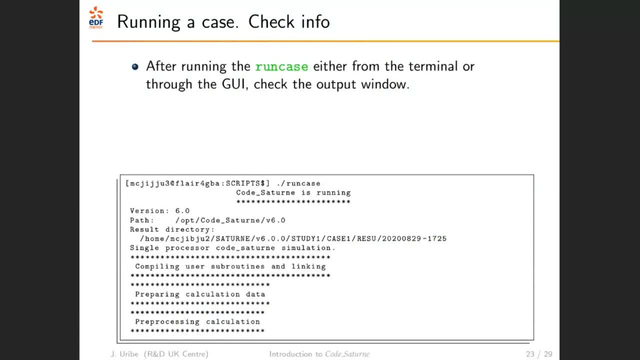 So what happens after you start running is the same thing that in your terminal. you will have the same stages that I showed you before on the graphical interface window. It will give you the location of the code, the location of your results, and it will show you at which stage of the calculation you are. 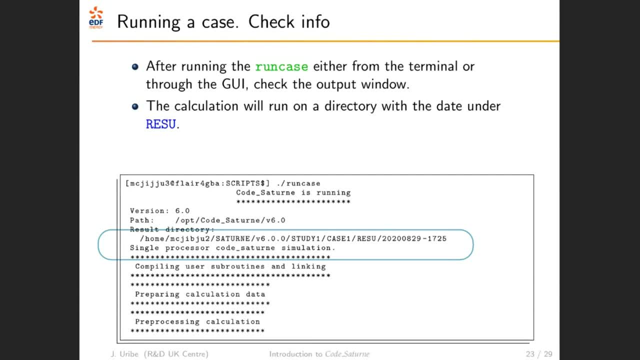 One thing that is particular for CodeSaturn is that the results file that every time that you run the calculation you will create a new directory So that line there is always going to change with the date and the time of your run, So it won't overwrite. 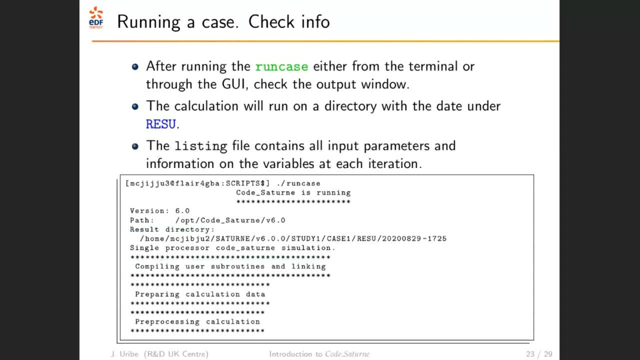 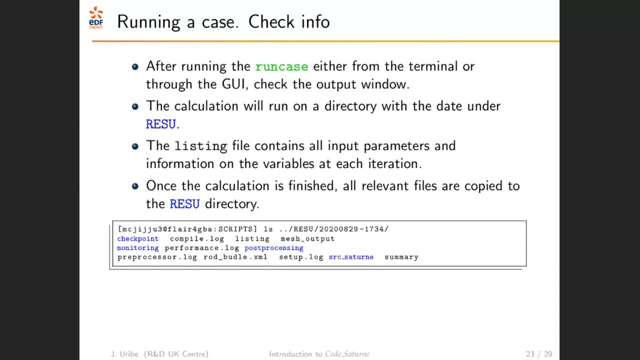 But that is the amount of files that you create that are quite significant when you start running several instances. Once you go to that results file, you see that you have various files in there. The listing file is one of the main files. There is a text file that contains a lot of information. 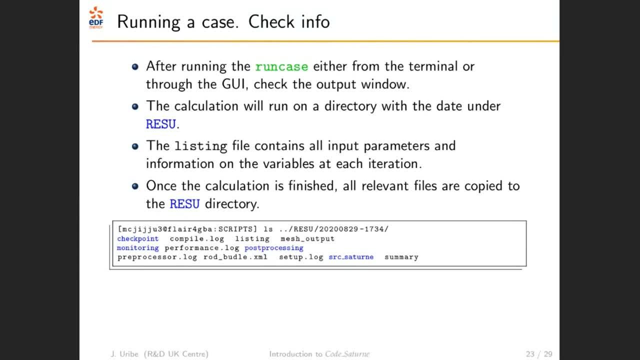 On the values that the code is obtaining through the solving of the equations at each iteration. So it gives you maximum and minimum. It gives you the number of iterations that it did for each variable, For example, what level of convergence was reached. It will tell you some things like if there are some clippings done, or things like that. 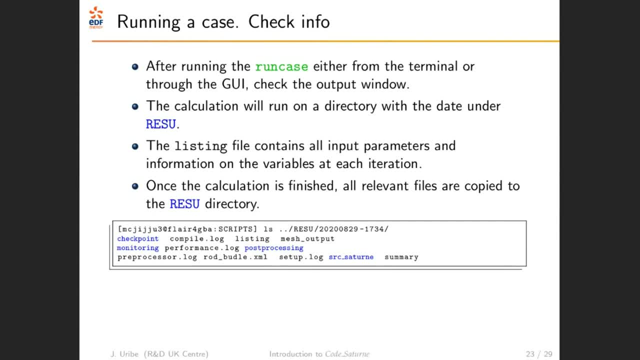 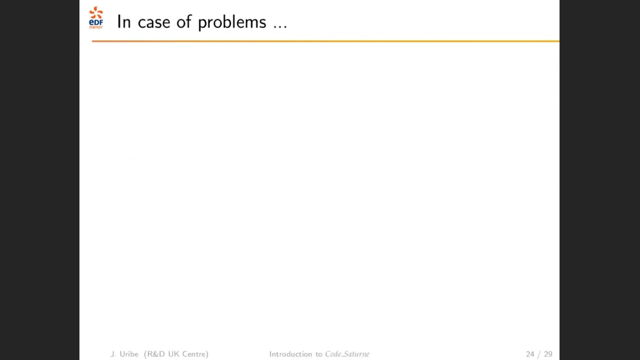 Okay, So your setup log will contain a lot of information about your case before it starts to run. So it will tell you things like what type of gradient calculation you've chosen for each variable and how many variables you have, etc. So you'll get also things like 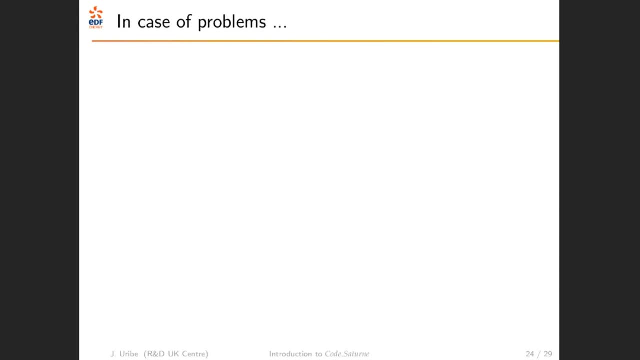 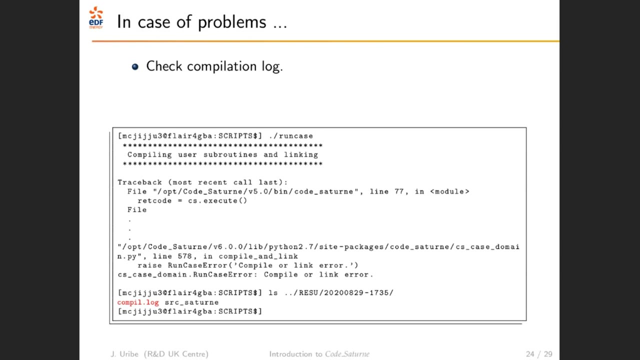 Your post-processing results to see the part of your files, etc. So one important thing is what to do when you have problems. First thing that can happen is that you have a compilation error, So you'll see a message. start to this when you have a compilation error. 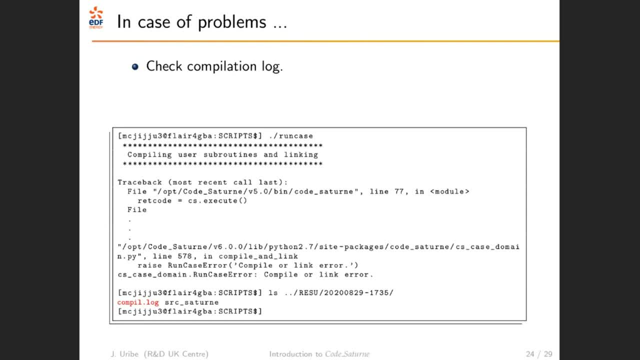 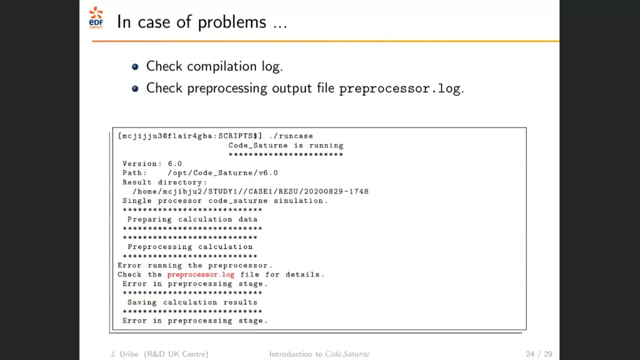 Compile or link error And you will see that. Tell you that What the error. if you look at the compiled log file, Then if the compilation goes right, then the next stage is the prepressing. You could have an error there as well. 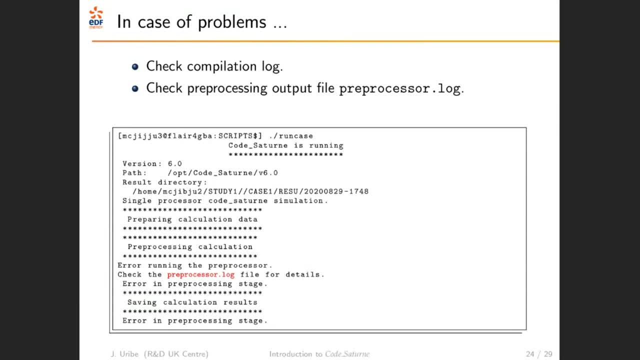 See, for example, if your mesh is found to have negative volumes or Your mesh file is corrupt or something like that, you will find it in this preprocessor log file, And if that goes all right, then your calculation could also have problems. 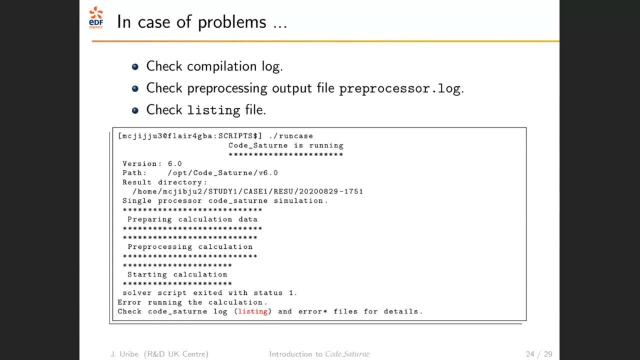 In that case you would check the listing file And in the error files it would tell you the things like, for example, if your equations are not converging or if your boundary conditions are wrong, or things that can happen, Or if something didn't work. it would appear there. 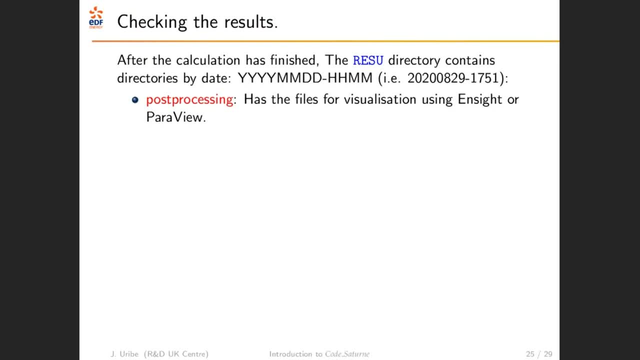 So, when everything goes all right, as I said before, your results would be in a directory that will have the date where it started, So you have the year, the month, the date, the hour and the minute, And inside you will have the processing folder, which is what you can use to see the results and create things like contours, vectors, floats or extract profiles, things like that. 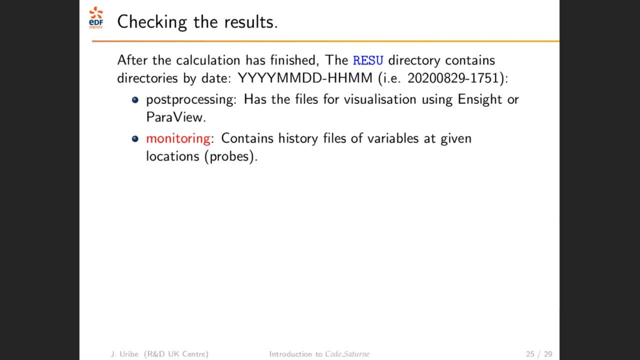 If you set up monitoring points, you will have a copy of those values in the monitoring points, sometimes called probes In Saturn language, And a checkpoint directory is quite important because that has all the values and all the cells for the last iteration stored. 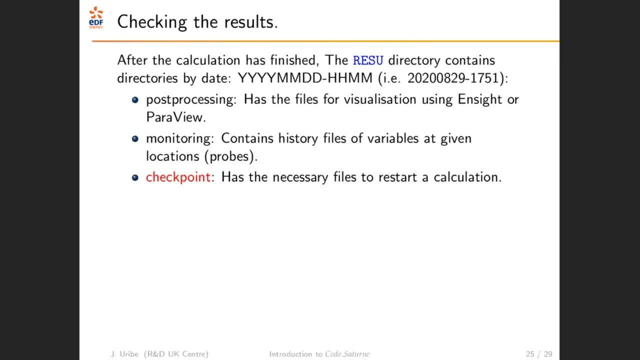 So you can read from there if you want, And that's a file that is only readable by Saturn, So it's a binary file. You will have a SRC folder And Where you have all the copies of all the subroutines that you use. 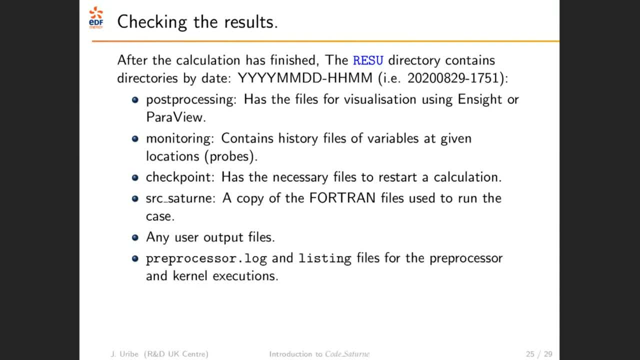 And you will also have a copy of any output that you define. So, for example, if you define files or you define data files at a certain location- And of course, you will have all the logs for the stages of the run, as I said before. 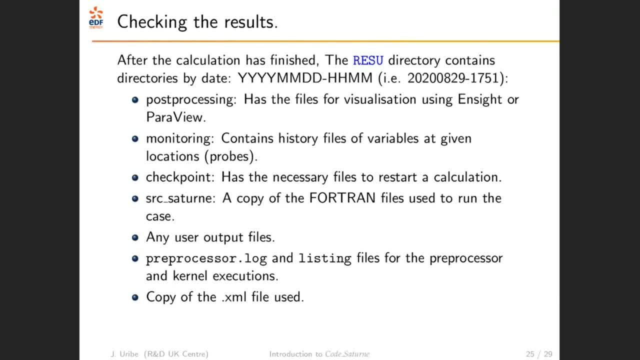 You will also save a copy of the XML file, Which is your input file, generated by the graphical interface. So, in summary, this file with the date, This folder with the date, will have basically a copy of all things that you used to run that case. 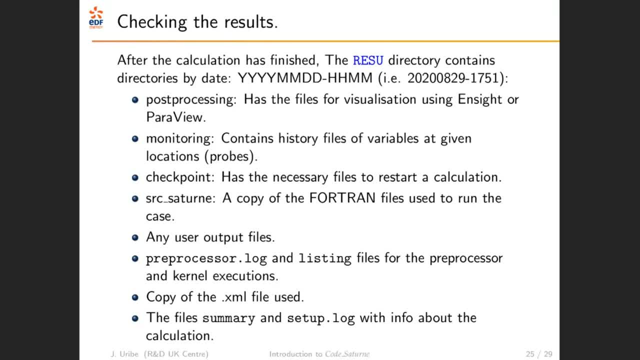 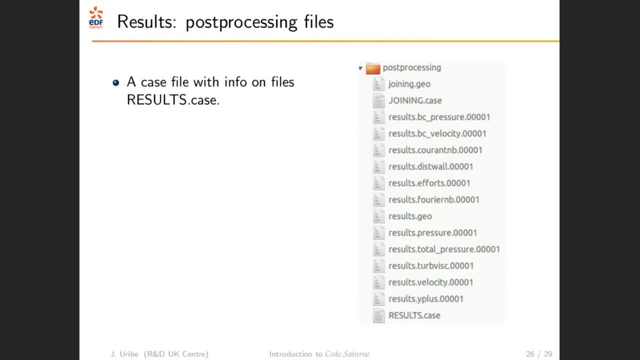 So you can rerun it again if you want. But all the information is there And Okay, Thank you, Bye, Bye. So The post-processing folder. So the post-processing folder will have a series of files. You will have a. 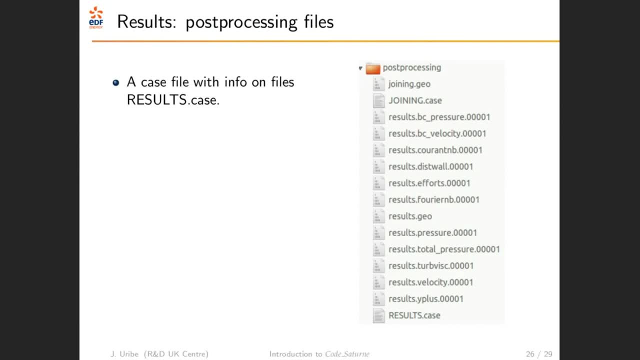 This by default in a format for InSight And inside, is a visualization software And it is not open source. There's a free version that is up to, I think, 2 millions cells And but if you want to do more things with that, you need to pay for that. but Paraview, which is an 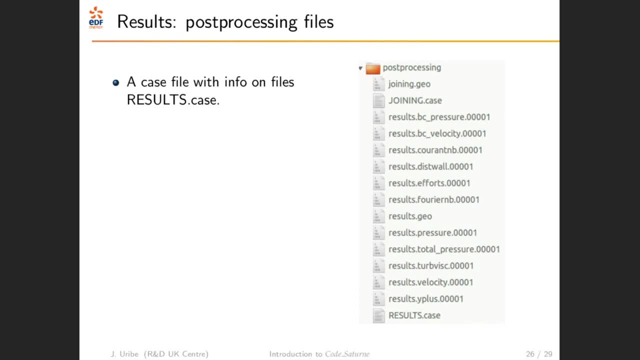 open source and free software can read these files directly, so that's why we haven't changed them. basically, the case file is the one that you would load in Paraview and that will tell the software what to read. what variables are there, how many time steps, what's the geometry? so all of this. 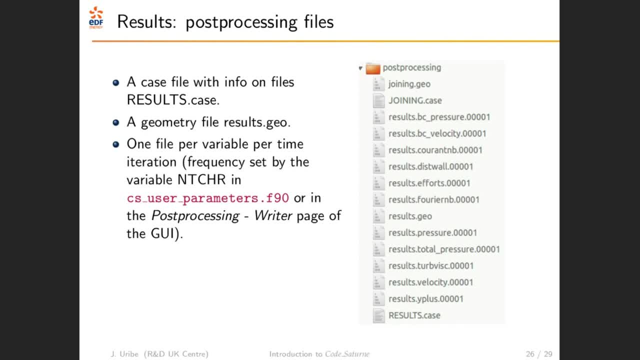 information is split on our serial file and you can change how often these these results are written. so by default you would only write it at the end of the calculation, but you can change that if you want to see, for example, some animations, or or if you want to save different stages of the simulation. 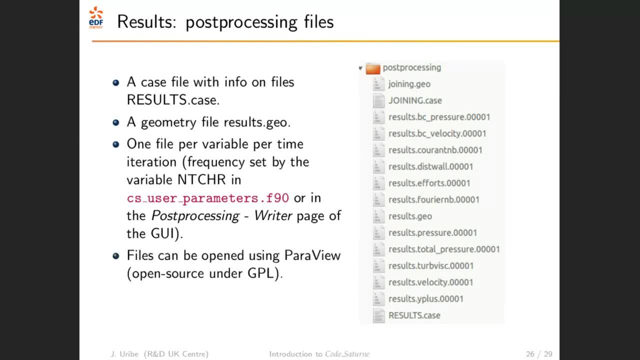 one important thing is that you can also create parts, and we call parts is subdomains, where you can select a smaller simulation. you can select a smaller simulation. you can also select a smaller simulation set of cells where you're interested in. so if your mesh is very big, your post-processing file. 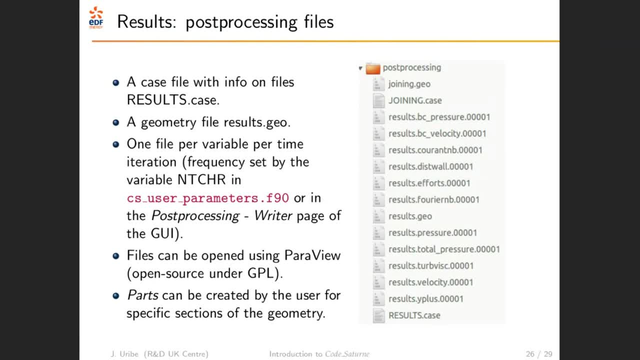 is going to be very big because it has all the geometry file, geometry information in there and sometimes you don't want to see the whole thing or you don't want to copy a very big file. you can create subsets of those parts of the geometry where you're interested and those subsets can. 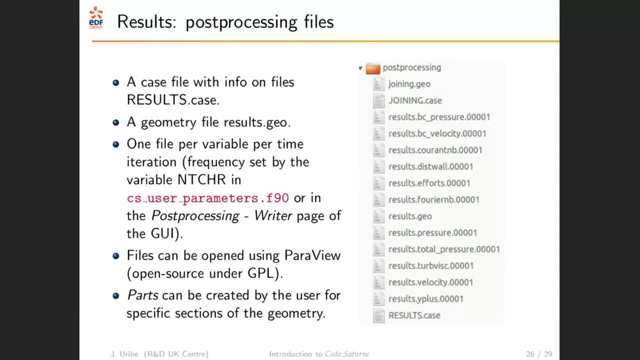 be either geometrically defined, say, for example, all the cells that are lower than x equals zero, for example- or they can be based on functions, so you can say all the cells that have a temperature larger than 20 degrees, for example, or things like that. so quite useful to when you have very 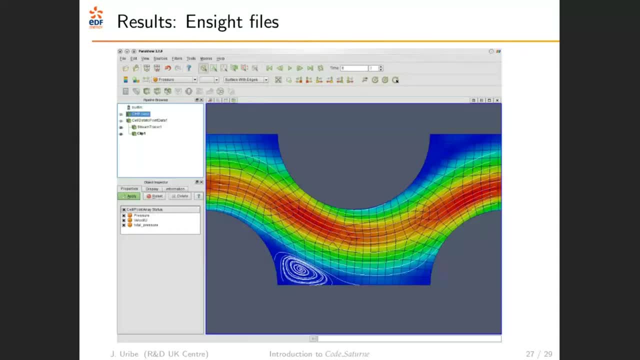 much cases and you don't want to see everything. this is an example of what you would see in para view. so in para view you will load your inside files and then you can do these things. you know: color the domain by any of the variables, create the streamlines, show the mesh or the mesh. 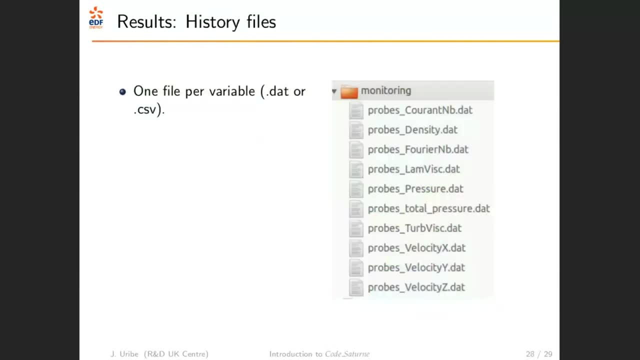 or anything like that. you also get a folder with the monitoring points. as i said before, you can define which variables you want to monitor. by default, when you create a monitoring point, you would assume that you want to monitor all the variables for that point, and then there's a file for each variable. 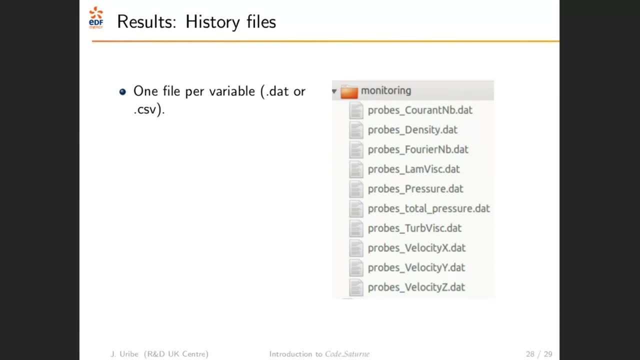 that file has a series of columns and each column is one, one point. so it could be a comma separated value or a space separated value. dot that file and it can. it will show you the variation of of that variable along the number of iterations or or time. 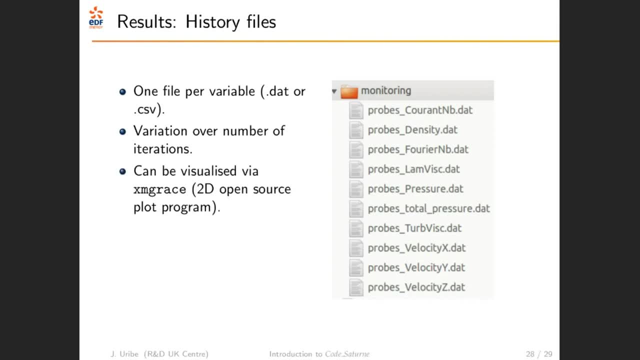 and you can select how often that is saved. so by default is every iteration, but you can do the retain iterations or everything and at the end it's just a text file so you can open that with new plot or x and grace or excel or any other program. 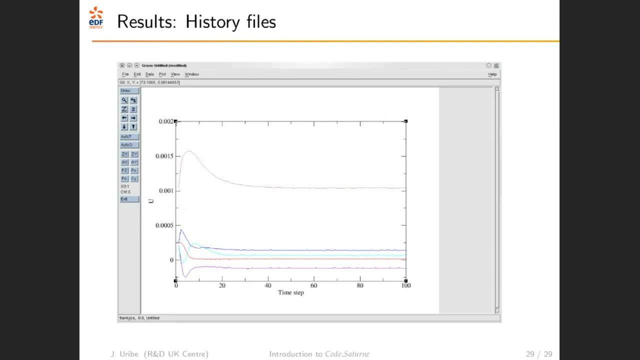 so that's an example of what you would see for any program, and i'd like to just about show you how it works for all of our programs. so that's the first tip that i just need to show you, but i want to say that it's very useful and if you're interested, you can come in. 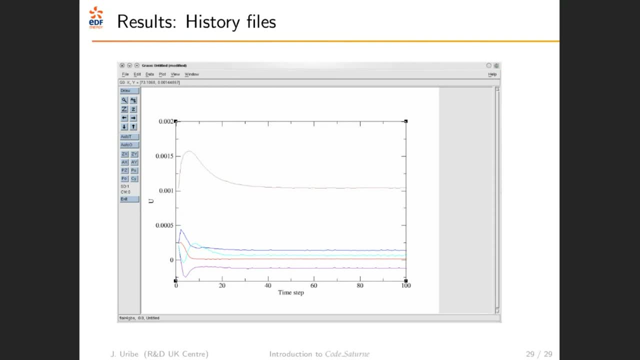 to the excel library and there's lots of information there so you can just go to friends or your other links and then have a look at the options i had at the beginning of the talk. you can search it in the chat and just check it so you can find all the options. 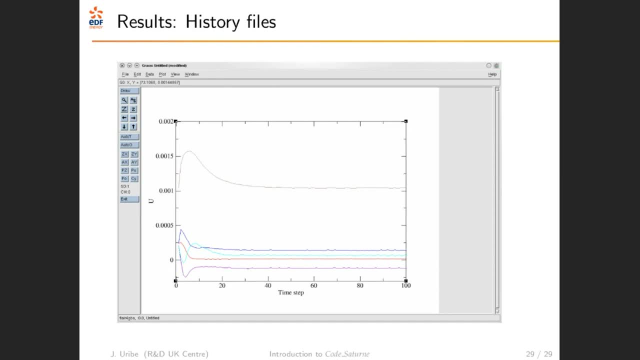 and you can see there's lots of other options, and once you click on, then the application three is the last one. so you can just click here and it will show you all the options, and then you can see the options also here as well. so, as i said earlier, this is an example of something that i really want to show you. 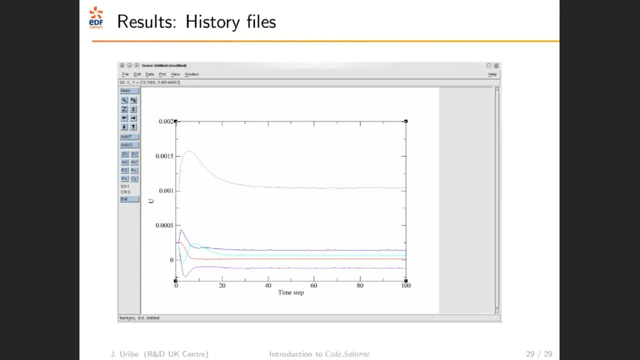 Well, I hope you could hear me okay and see the slides okay. So what we're going to do is go through the first tutorial and I'm going to show it here. You should have a copy of this with the files that I sent you. 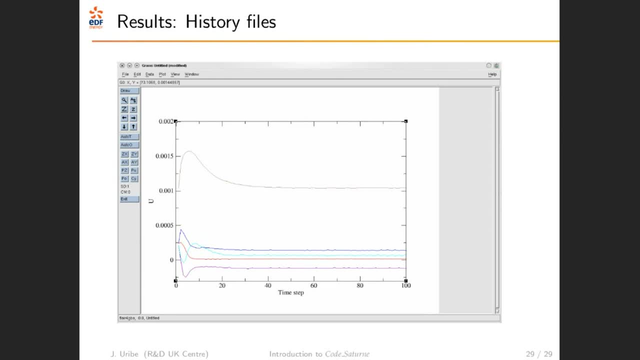 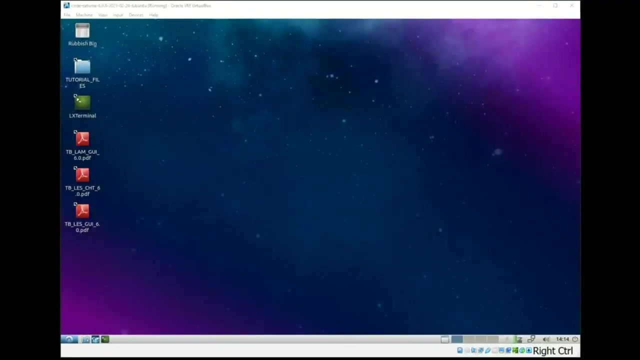 I'm going to share my My screen. Is anybody here using, Okay, Okay, Okay, Virtual machine that we sent for your own installation? Complete silence. Okay, If you have your own installation, download the tutorial files, zip file in which you can find a copy of these PDFs. 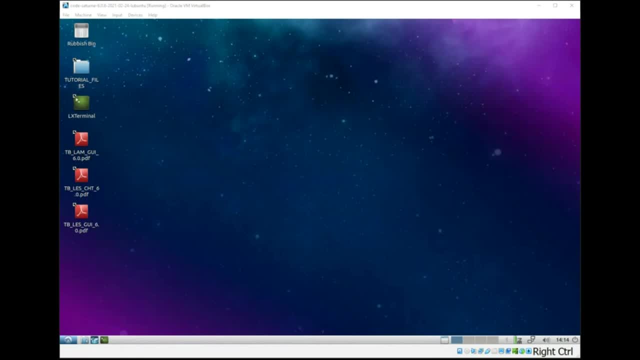 If you have the virtual machine, they are on your desktop And you can just start with the lamina one. Okay, Okay, Okay, Okay, Okay, Okay, Okay. If you have any problem using the virtual machine or starting CodeSaturn, please let us know. 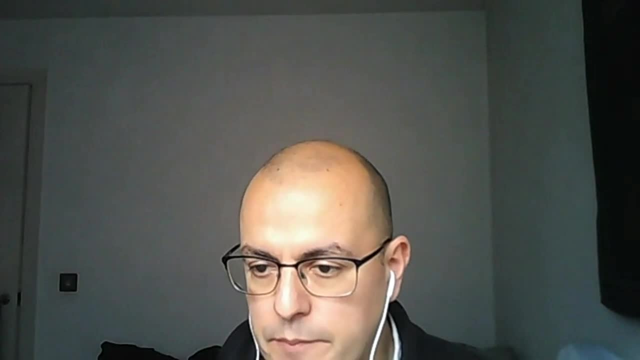 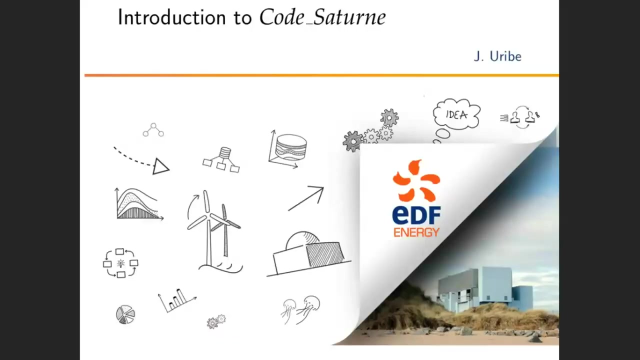 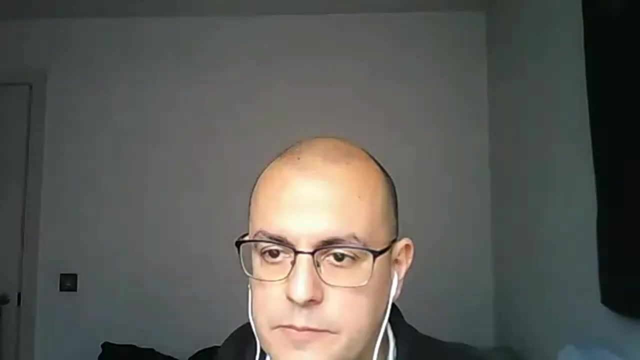 I'm going to put up the first tutorial here. I agree, Okay, Okay, Okay, Okay Okay. Thank you very much, and hands down this tutorial video. I really enjoyed it. If you have any Penny, please let me know the instructions. 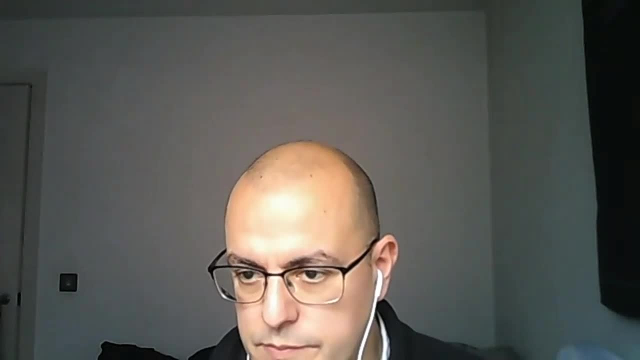 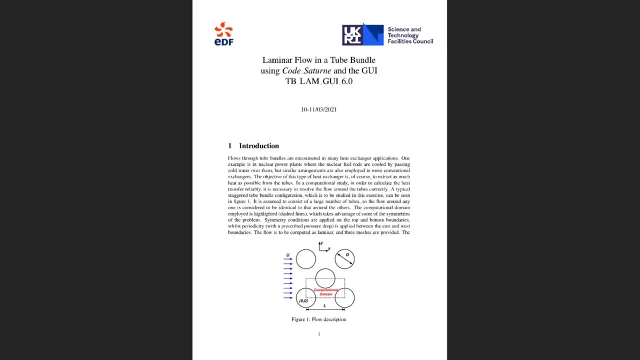 in the comments should you have it or not. Thank you, Thank you, Bye, Bye, Bye, Bye, Bye. All right, so this is the PDF that you should all have, and the idea now is that you go through this tutorial. it explains a very, very simple case to start with, and let's 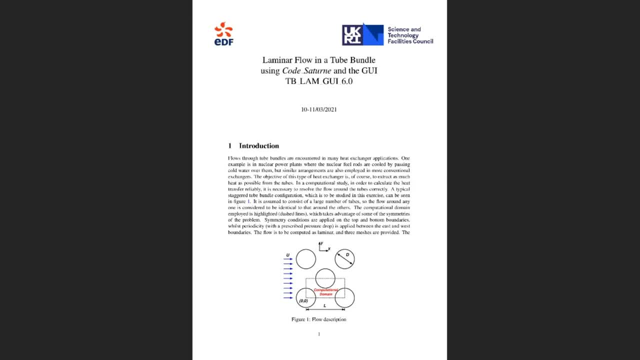 see if I can make this bigger here- which is, as Charles mentioned at the beginning, this is a tube bundle. so we start from the most basic domain, which is just what is dotted here in this picture, and we're going to just do a very simple laminar flow. 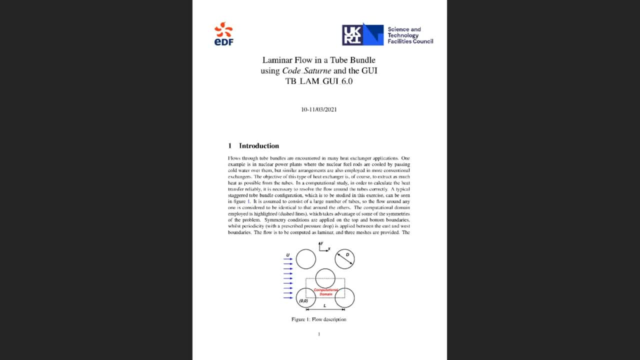 You can run it either on your PC or in the virtual machine. The measures that we are providing You are very, very small, so it's not going to be very heavy on your computing resources and it's going to run fairly fast. 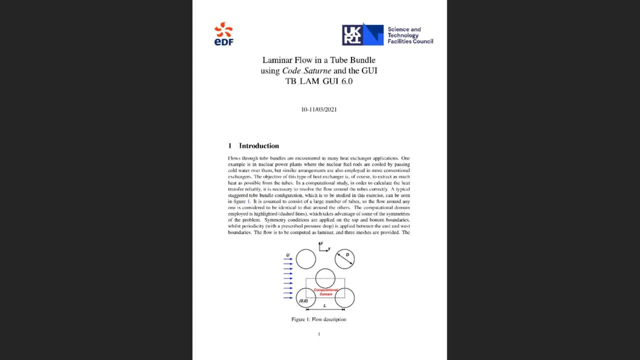 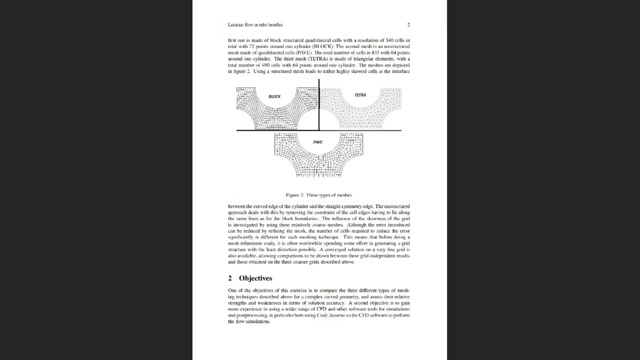 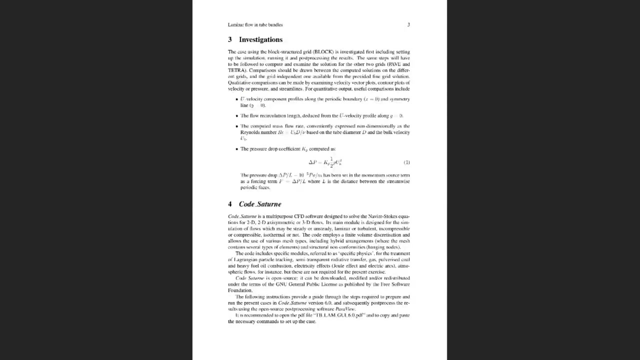 We only do a few iterations, so it's just for you to learn how to create a case and run it. So please feel free to go to the pages of your tutorial and try to run the same case with different measures. This is a step-by-step, so I should show you all the details using the Graph Interface, of course. 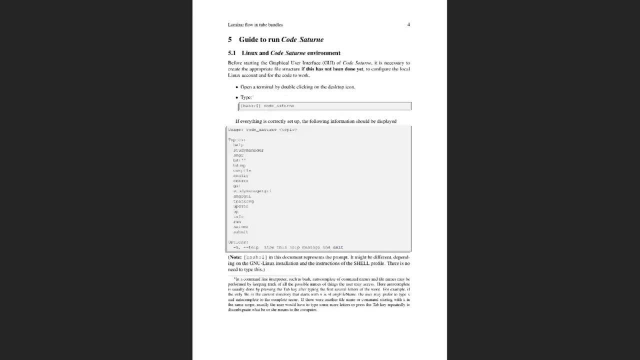 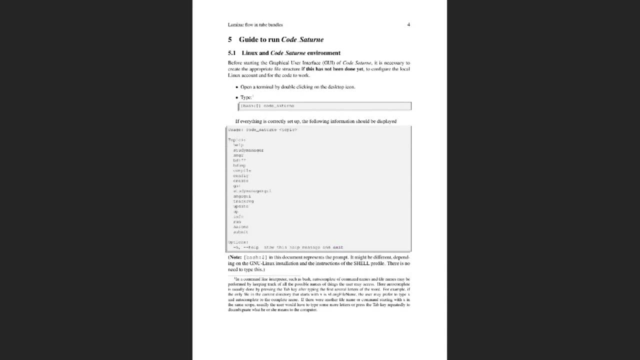 If you have any problems, feel free to ask. So this is the transcript of the tutorial. I will show you how to do this in the chat, or just raise your hand and talk. We're happy to hear you Some of these explanations. 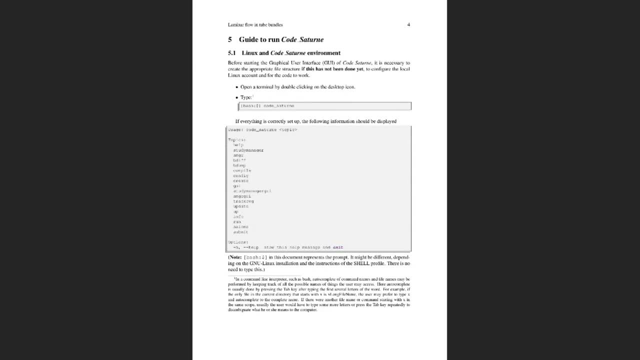 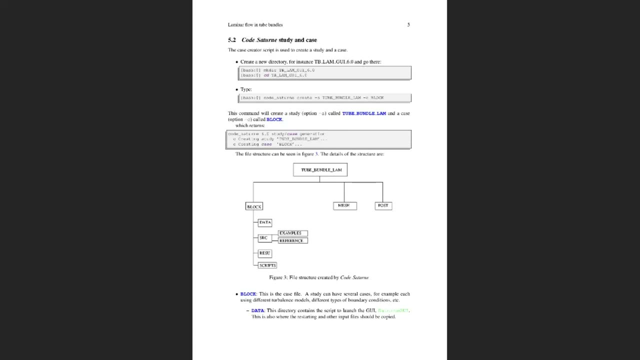 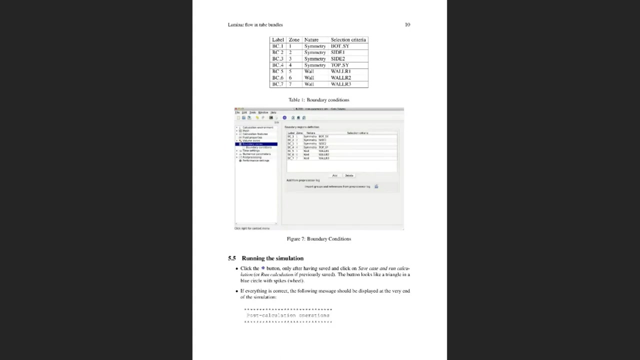 are already in the presentation that I gave before. You'll see that by the end of following these instructions, you should be able to run your first Saturn case. So we're here if you need us. Thank you, Okay. I think we are back to the break from the break. sorry, We are going to have a presentation. 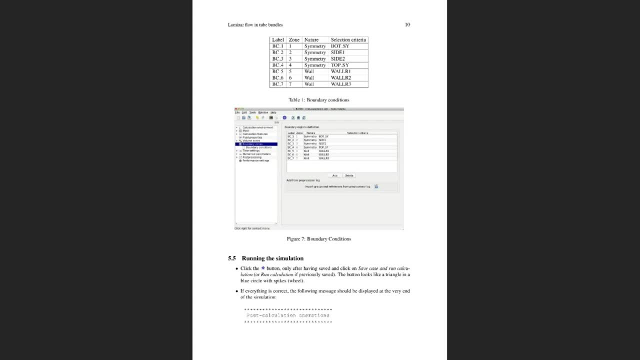 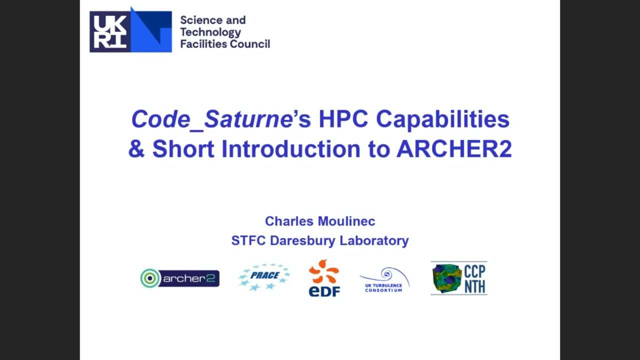 now about HPC and HPC for CFD, with how it is managed into CodeSaturn. So I'm going to load some files and share them with you. Okay, Okay, Can you see the slides? Yes, Yes, Okay, Thanks, Okay. So this presentation is for about half an hour or so. So this is to show the capability of CodeSaturn using many, many, many processors. 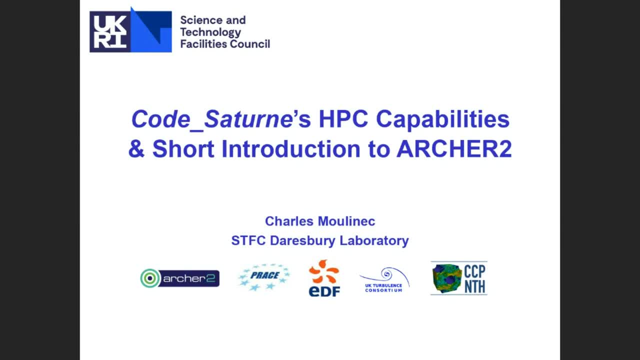 But you also to think that I mean, is the code that's been written for massively parallel machines that they also run. but it also run fine on just one processor without MPI, on just with a without a bear compiler. Okay, so sorry. So basically it's what happens is you have two processor and because they're all속ope ticket isiendo very, very far And there's there's special�unstance problem to any low-end computer That's very important in in industrially. So I think it's important to you know that people who can use multiple controllers, quite often You know multiple��. 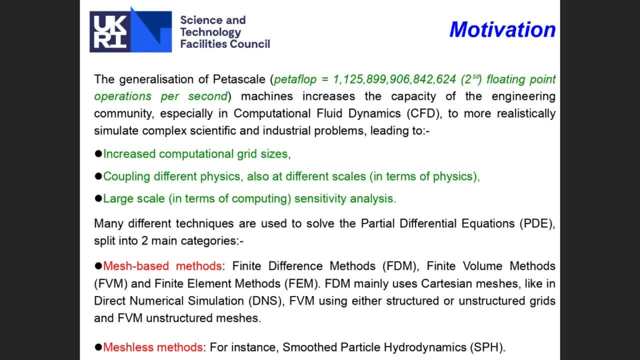 If you don't know, you may be able to do it any other way, But I think, my God, basically the motivation is this talk is that the current generation of machine operating at beta scale and exact scale should be ready by this, the end of this year or maybe next year. so if you see that peta scale, respond to about the 2. 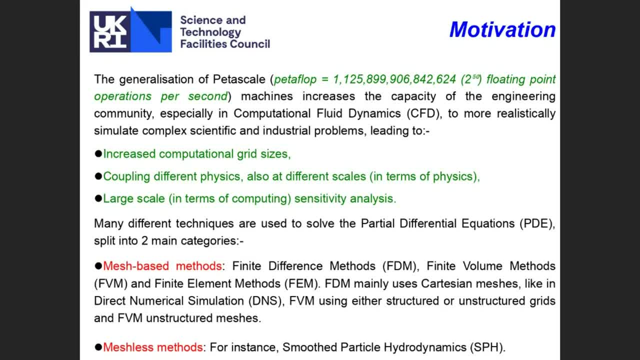 to the power, 50 floating point operation per second, so which is massive. so what do we do? when you are doing CFD and we've got access to a full machine like this? there are several options so it's possible to increase the size, the computational size of the of the current configuration, so you can also increase. 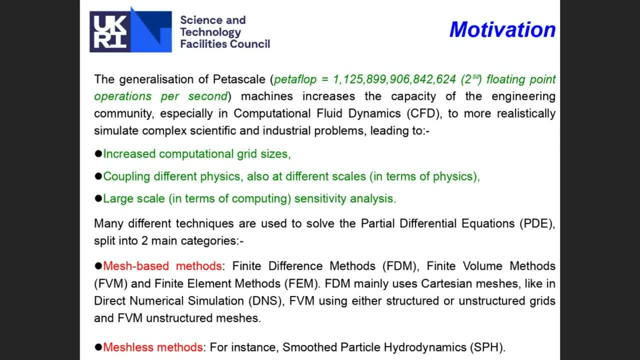 the- I mean the Reynolds number- make it more complex, adding more physics or also operating at different scales. but it is also possible to do some sensitive TVT analysis. so running parallel simulation actually don't communicate with each other, but at the end of the simulation you, you basically extract. 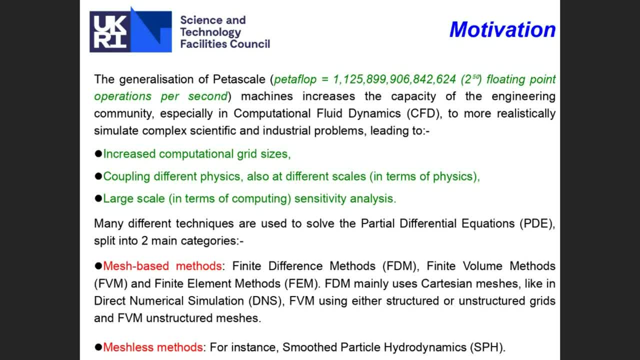 some feature through statistical analysis. so we we find that there- I mean they they are basically two different approaches, so either the mesh based methods or the meshless methods, but they've got a lot of different ways of doing it. so I think it's really important that we 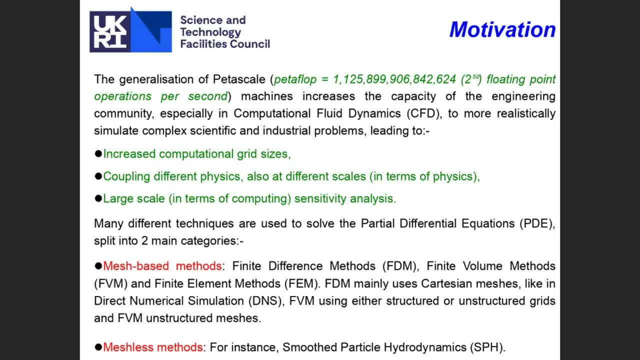 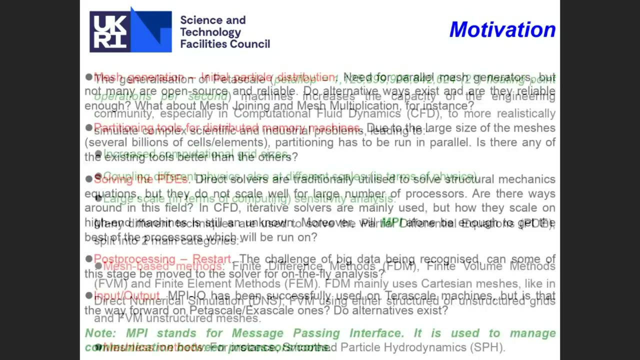 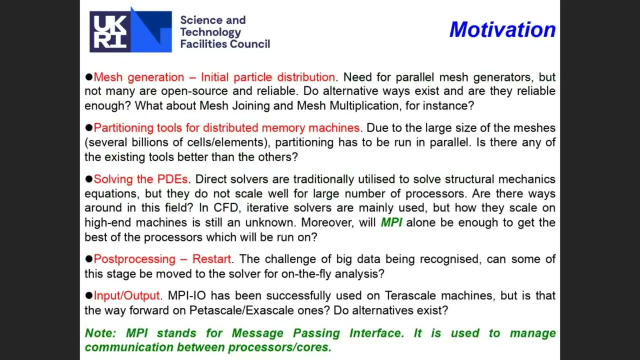 we've got a lot of common grounds so we try to identify some of them and we try to see what's done in code Saturn to to, to run at extremely large scale. so we are notified five different issues you could. you could hit running a CFD on. 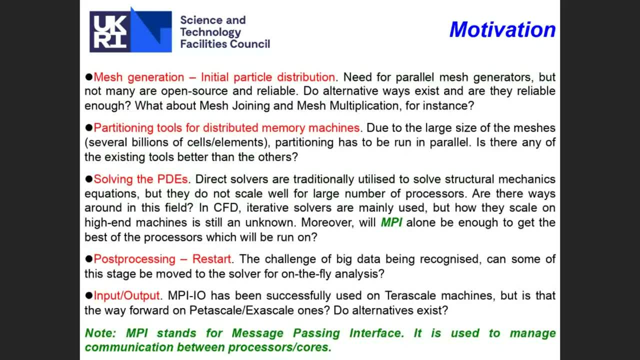 this large machine. so the problem, the first problem, is a mesh generation. so these trzy 나�squ Elsevier, usually emasculator, a serial, so they're a unit, a very fat node if you think that you want to generate the measure using billion of cells. so I mean there are. 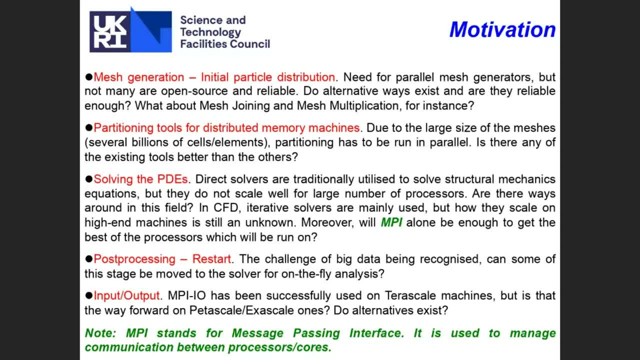 they ways around. so we're just going to see what can be done into the code for that. then, when you got your mesh, you need to distribute it across the, the Choruse or the nodes you've got access to. but you need two sono to form one engine online. if you got to thể. 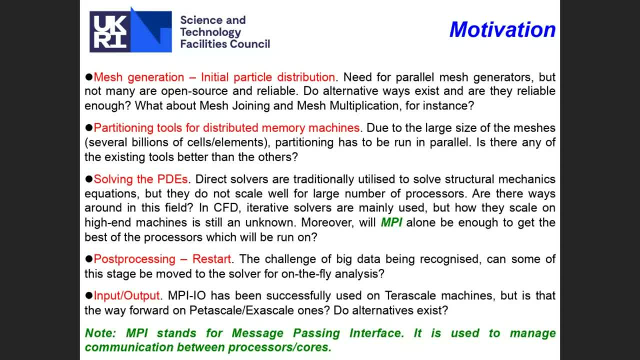 But you need to do it in an efficient way, especially if you need to repartition in the course of the simulation, Then solving the PDE is obviously key, And this is an aspect which has been, I mean, focused on and with a lot of improvement along. 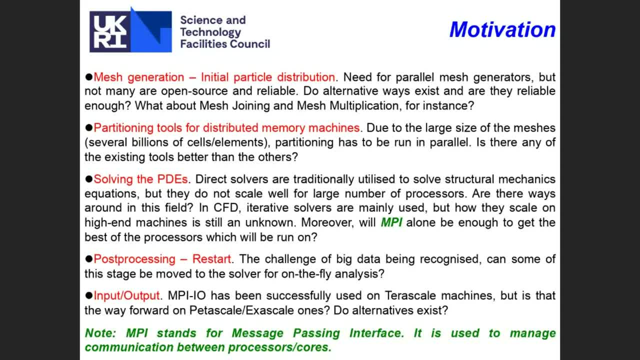 the years. Then obviously the big machine. they work with queuing systems, So the chance that you have to run only a chunk of your simulation, given the 12 or 24 hours you've got access to, is massive. So you need to have a process to down the disk and to read them very, very quickly. 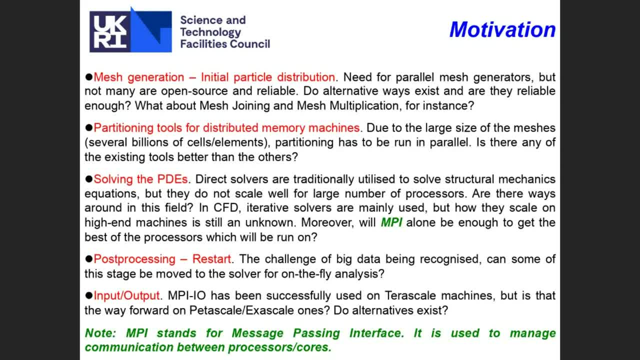 And we need to see if there are bottlenecks in there. And finally, the MPI-IO, which has been developed for quite a while Now and working well on terascale machine. is that suitable for petascale and now in? 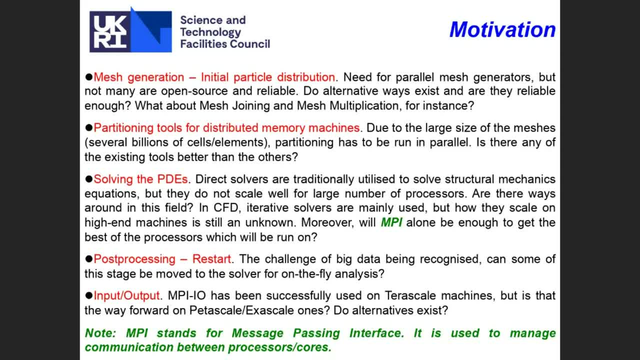 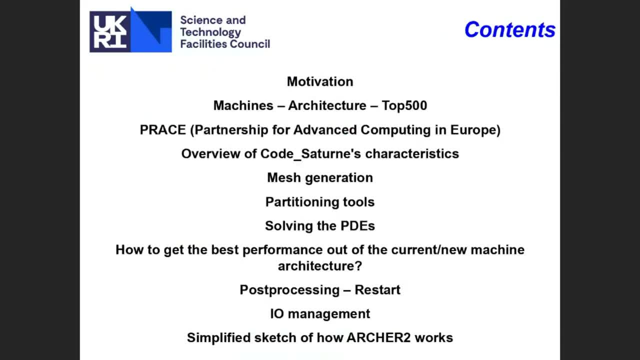 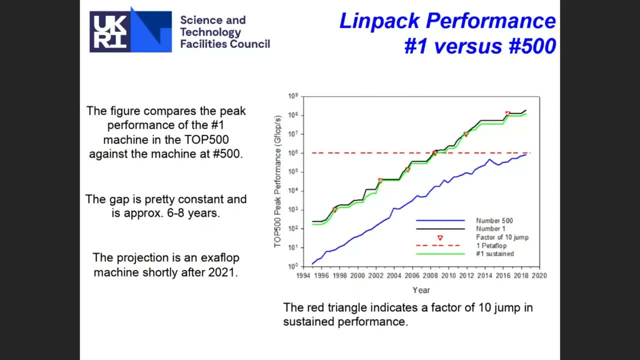 the future for exascale. So we don't know that yet for exascale, but we can have an idea about what happened at petascale. So this is a content of the talk. So I'll pass to what is called learning pack performance. 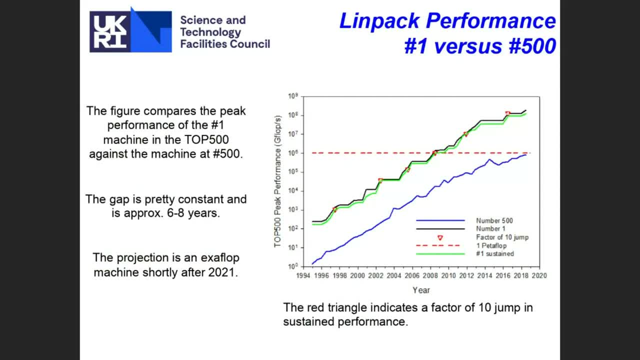 So some of you might know that there's a top 500. Listing the 500 public machines, the fastest ones in the world, And there's a suite of tests which is run to assess their performance. So there's the theoretical peak of the machine within built and then this lean pack suite. 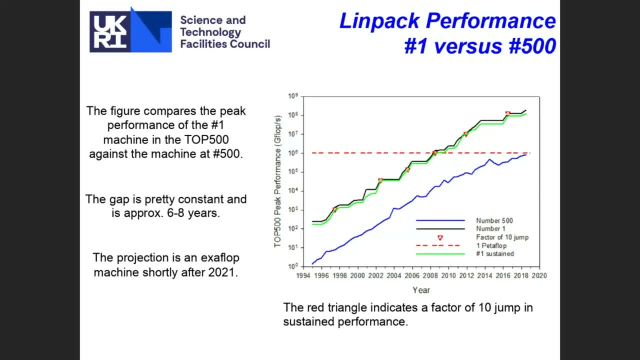 is run And they're designed to assess the actually the maximum peak that they really achieve. And so, if you look at this over the years, so let's go until 2019, but the slope is. I mean the same trend is observed for the fastest machine. 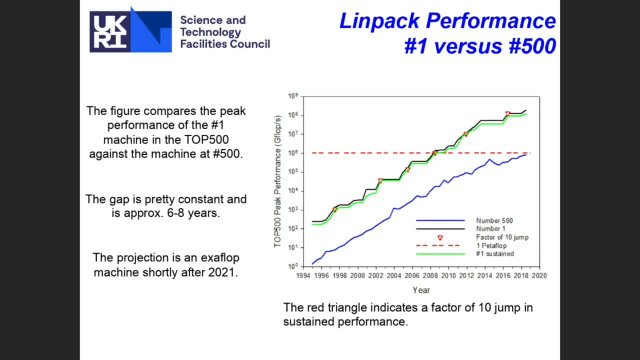 The basic events Also also for the, the source machine of the top 500, which actually almost reach petascale. so that means looking at this graph. that is very important to have a massively parallel code for cfd and to get the best of these machines. 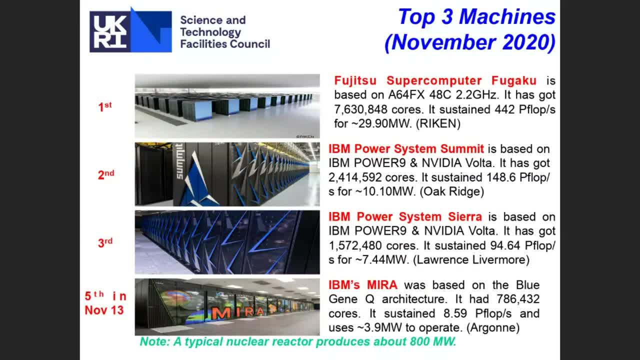 so the top uh, three machines in november 2020, the- i mean they're trying to go for exascale now, until a couple of years back was to add gpus to, to, to cpu, or several gpus or accelerators per node. but it happened that the fastest computer in the world doesn't use accelerators, but only. 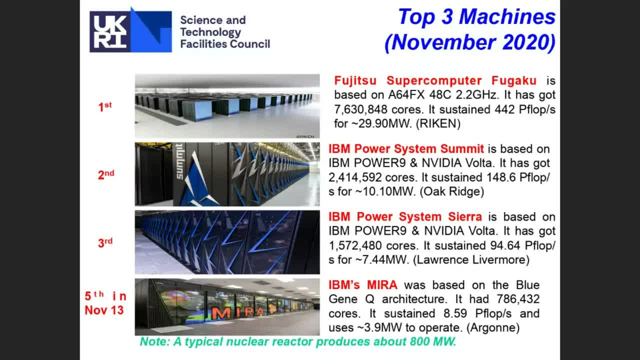 uh, cpus, based on arm processors, and. but the common trend of all these big machines- the three first machines uh- is the number of core you've got on this machine, so they're all over a million. and the the second and the third are two ibm power machines and they, they all. 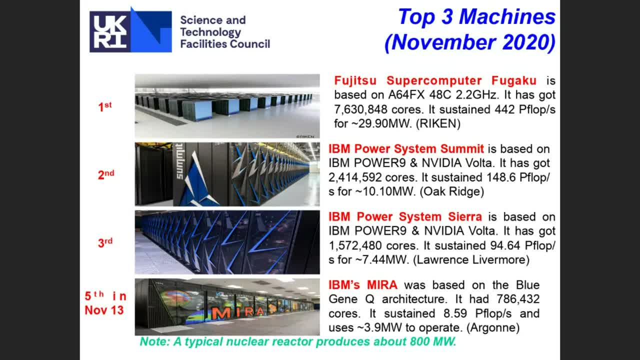 all have accelerators. summit's got six gpus per node and i suspect that sierra's got four only. but four is already a lot of gpus per node. and the last machine at the bottom is a an old type of machine called a blue gene and which is decommissioned now. but this is where we 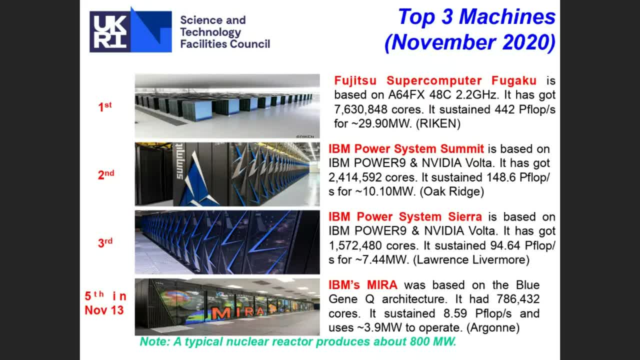 run the. the largest test cases or tests using code such as this machine has got 0.7 million cores, so the, the there's a requirement to build this machine. basically, it's possible to run an exact scale machine to to build an exact scale machine at the moment, but one of the requirement is to. 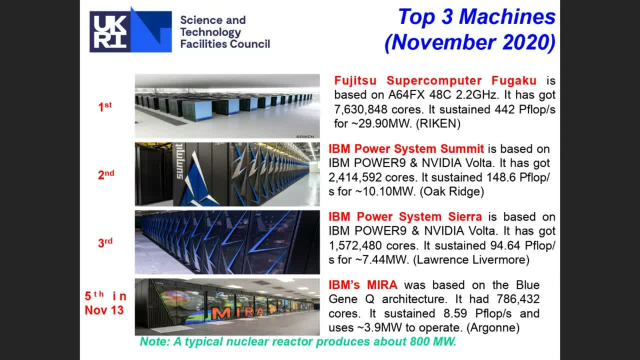 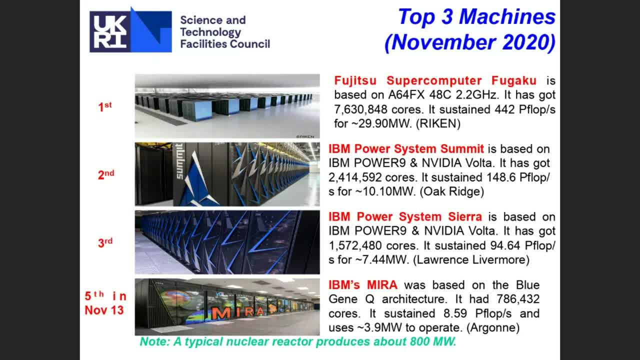 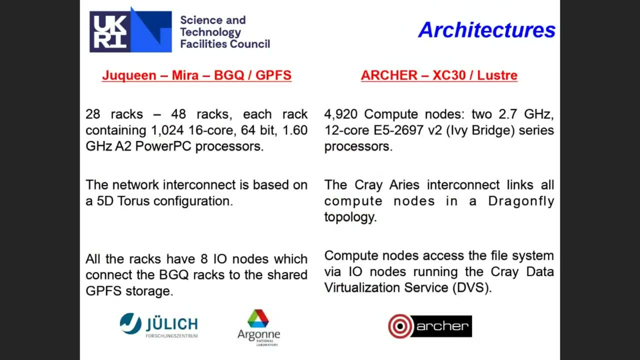 nuclear reactor. so that's, that's quite a lot. and the fugaku supercomputer goes up to 30 megawatts, is in japan, by the way. so here the attack texture which been tested. so, uh, on the left hand side you've got the blue jeans. so this where assets for the, the larger simulation, been run on this. 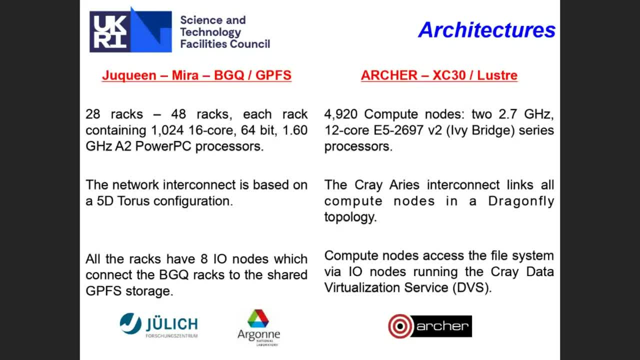 but the, the exита Resident turn and anywhere in the assed biggest Pascal-based stalin inputemic report is, you know, been published eight months ago and the, the extensive tests been carried out on the, on the, on Archer which it has the commission, and some tests now are ongoing on Archer 2, so the new, the new. 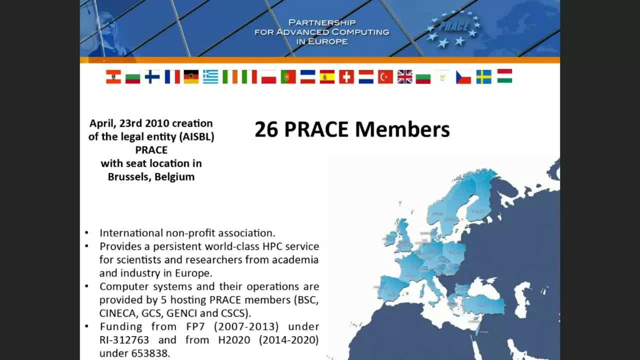 machine. so the this, uh, these both are craze, but with different types of of processors, praise has helped to develop some, some, some part of the code, and he's also the praise that sponsored this course, so it's a. it has a a good most of the european members. 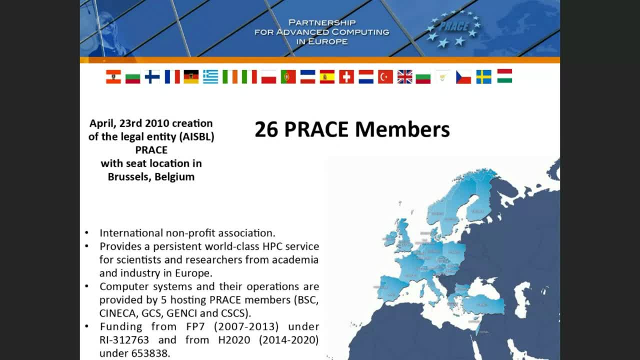 and so it's a international non-profit association and it it runs since uh 2010, but actually it started in uh 20 in 20 in 2007, 2008 already. so adasbury would be involved in in in a benchmark suite where code saturn is. so there's basically a suite of software. 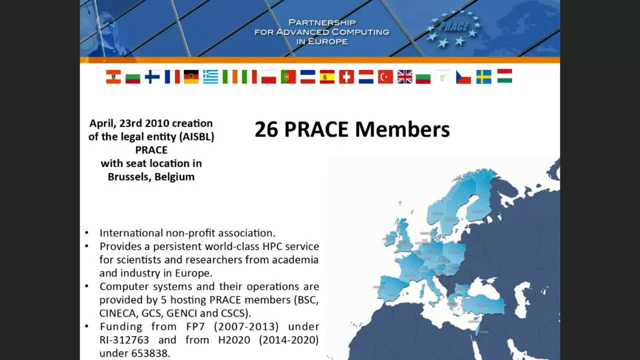 that people can download to test their their new computer or or the content performance of their computer and their clusters, new clusters. so in this suite of software you've got 14 software, and section is one of them and there are only two. of them are dedicated to the mechanical engineering and the second one being alia, which is developed by 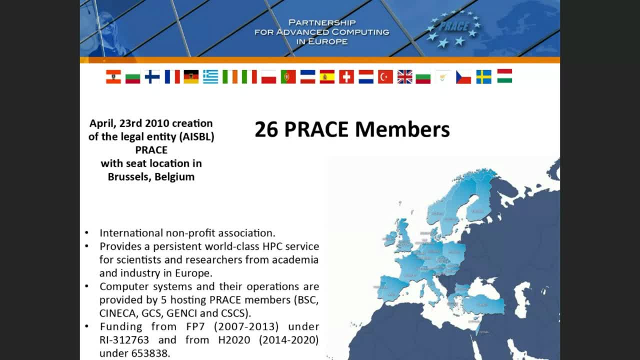 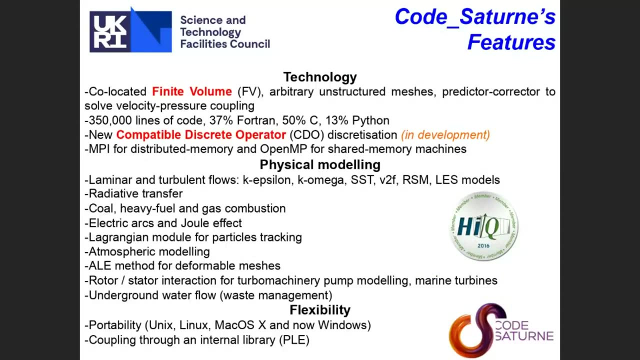 barcelona super computing center. so- and that was me- we are actively involved in in maintaining the presence of consumption in this benchmark suite. so, concerning the feature of saturn juan already showed that. so before. so what's important for this talk is that the um it's a mixture of, the code is a mixture of. 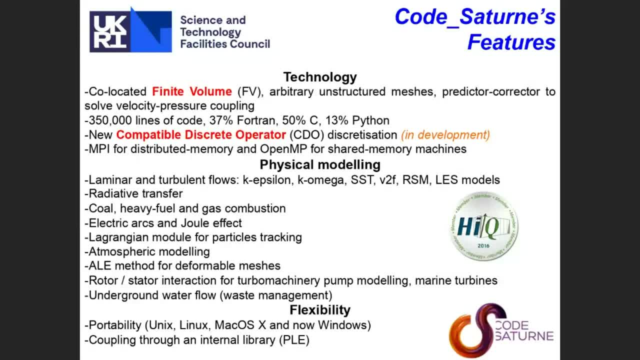 c and fortran with some pattern to manage the simulation. so, concerning the, the physical money, it's, it's it always expects to get to more realistic physics and it's driven because the edf on its own has uh to um to able to simulate a lot of uh. 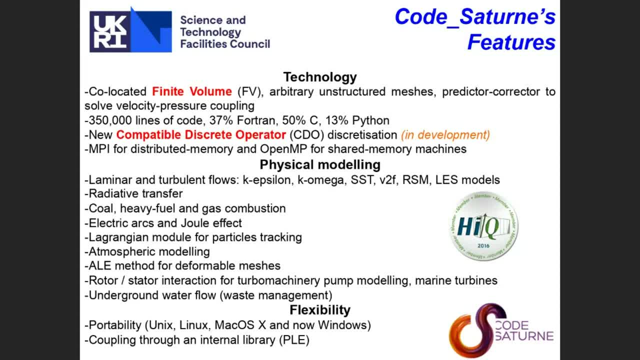 a lot of part of the power plant and is a is uh driven towards the parallel um implementation because in the future they expect to be able to simulate a full nuclear reactor. so you can imagine that i mean you, you. you need a billion or hundreds of billion of cells just to run one simulation. 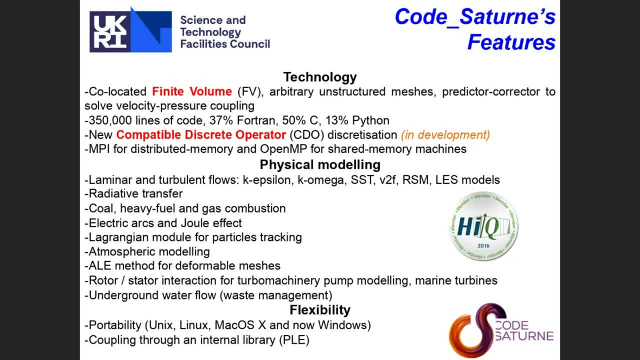 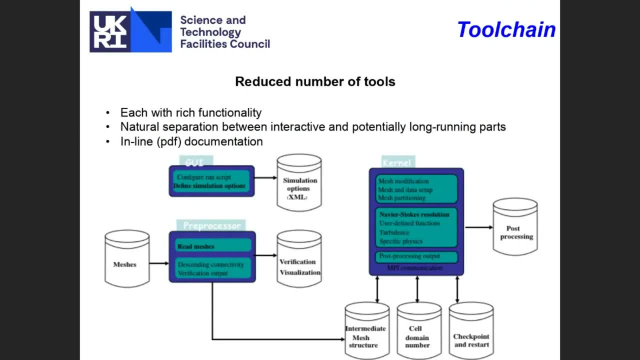 with uh, with advanced benefits modeling. so the tool chain that i have here is very similar to the one that one show this morning. so you have to think that on the left hand side, so just under the gui, all this part is a serial and and the kernel, which is on the right hand side, all these parts is 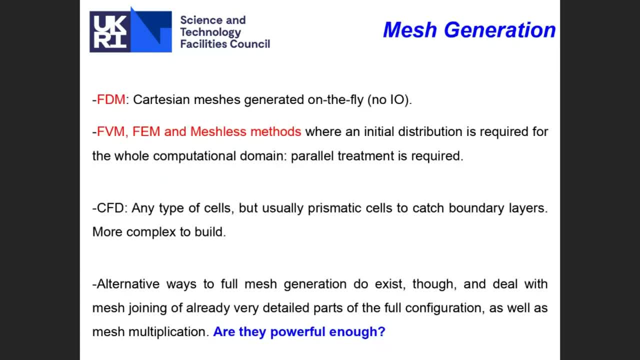 massively parallel. so now, if we go to mesh generation, is that if you would use a technique called finite difference modeling, the meshes can be generated on the fly, because the the complexity comes from the are solved, but not from this generation. in these cases, When you go to finite volume, which 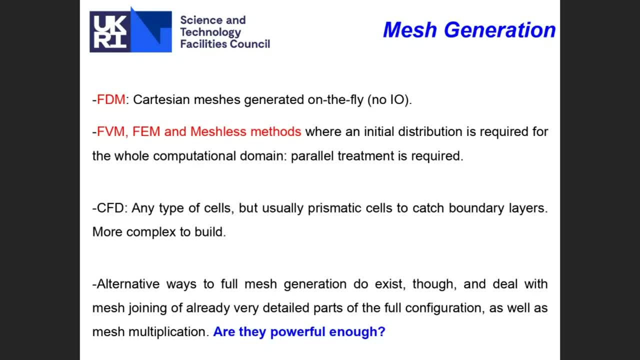 is the case of- and you've got cells or elements, we've got, I've got any type of shapes. you get very, very complex in terms of structure, very complex meshes, And we are thinking now in this case, going towards a billion and a billion cells. 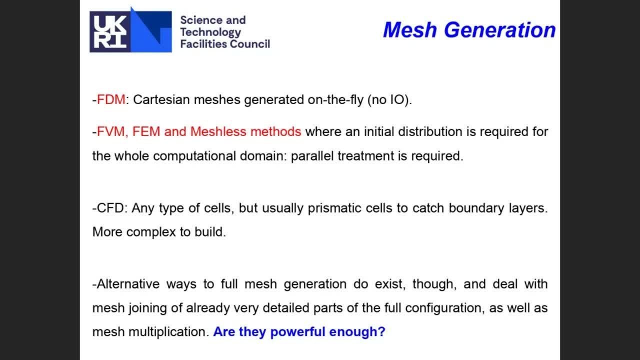 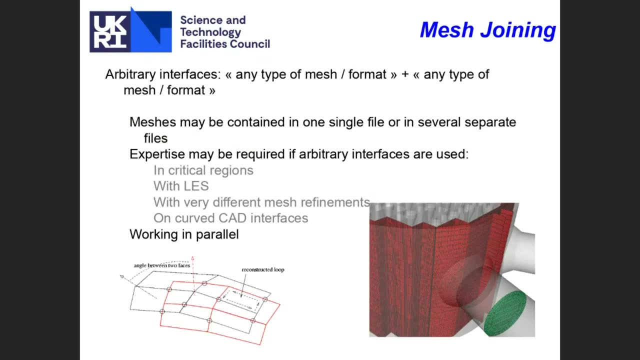 So it's impossible to do that on a serial machine because the memory is not available And on top of that it would take too much time. So there are ways around. So one way around is to build several parts of the mesh independently and to load them into the code. 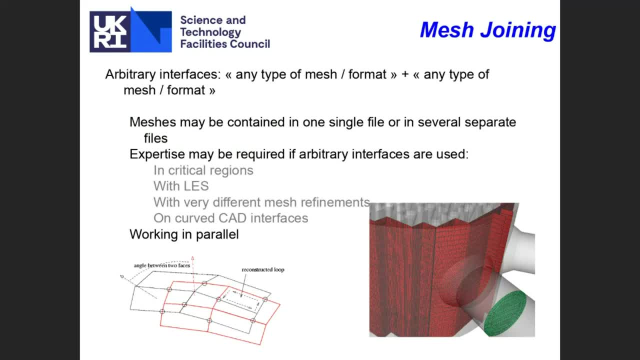 and to glue them on the fly. So it's called mesh transfer, It's called mesh joining in. so this is used extensively. It was actually used to build the periodic boundary condition you had to build in the first tutorial, So this is the same technique. 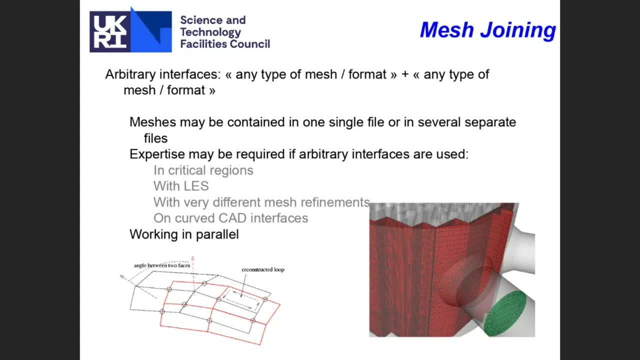 So basically, it's possible to glue conformal meshes but also no conformal meshes, which is described in the book In the bottom left in the plot, when you can see an overlap of two different meshes, and extra faces are built there so that the interface actually 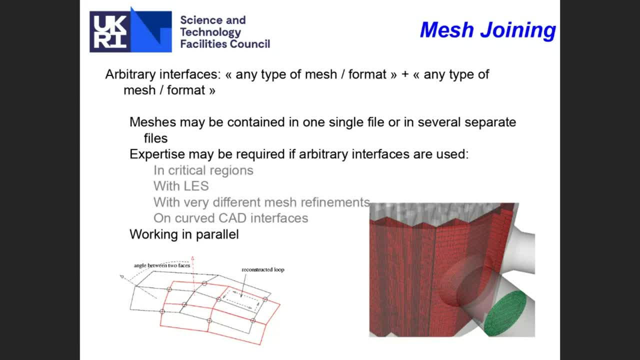 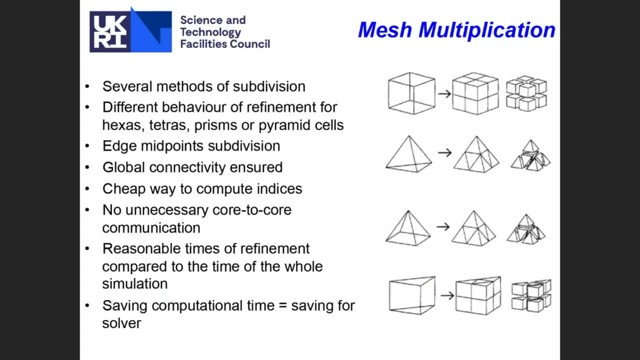 becomes a fluid interface and not a binary interface. So this is done on the fly and fully parallel. So the other technique to generate massive meshes is to start from meshes that we can manage. So meshes we can manage can go up to, let's say, 25 to 40 million. 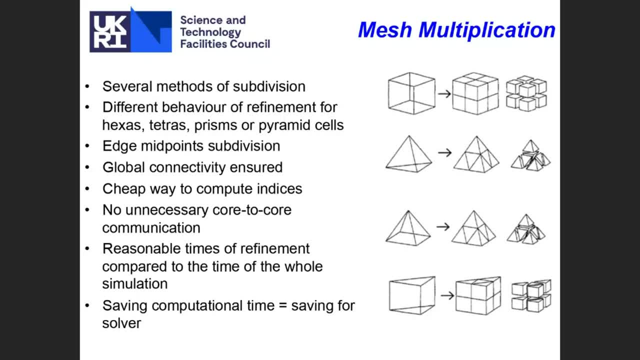 and really up to 100 million with a massive stretch. And then the idea is to use a technique called mesh multiplication, So you would refine globally all the cells of the mesh and then you can get a very big mass. So a cube would be split in eight cubes, a pyramid in 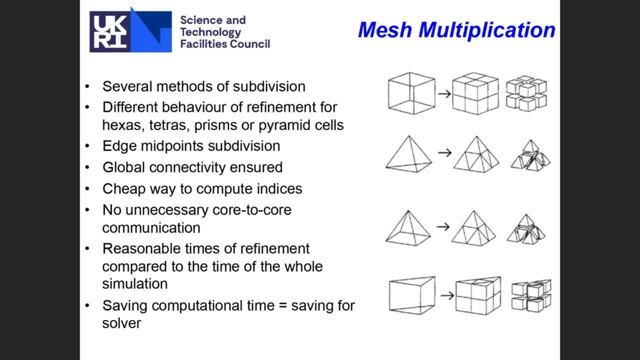 I think, 12 small pyramids, a tetrahedral in eight tetras and a prism again in eight, And this is done on the fly. This can be done locally by processor and is extremely fast, And by doing so you actually multiply. 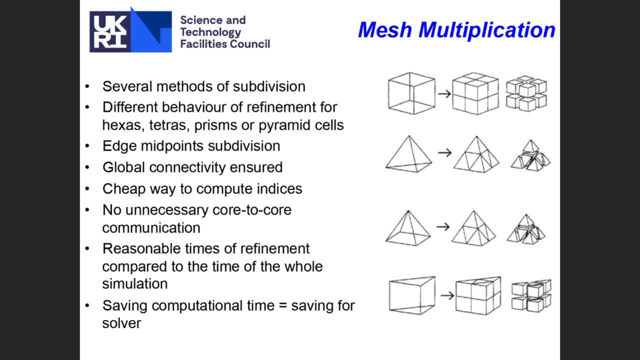 You multiply the size of your existing mesh by eight, once and 64, and so forth, And you can generate massive meshes doing so, And you keep everything in the memory. You don't have to dump that on the disk, So you save a lot of time in terms of IOs. 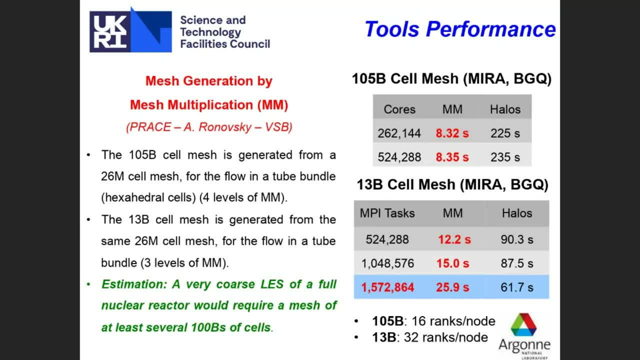 So in terms of performance, so the has been run to date using code, has got 105 billion cells, So the simulation will run on a mirror in Argonne in the US. It was a machine run by the Department of Energy over there And remember the machine had got up on 7 million cores. 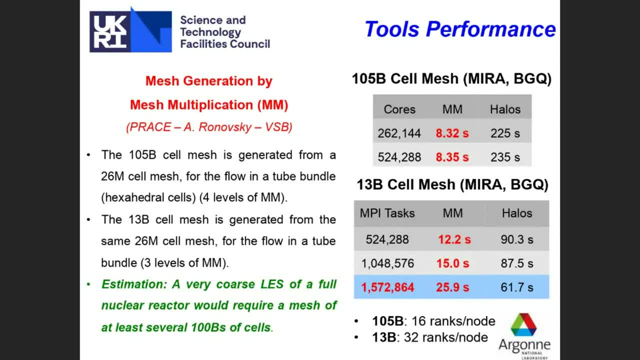 So for the mesh generation we run up to 1 third and 2 thirds of the machine And it only takes- It was taken, It was taking- eight seconds to run four levels of refinement there. So it's extremely fast If you imagine comparing to copying a file across. 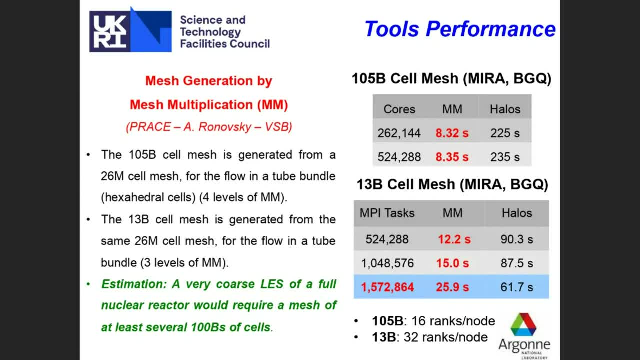 which is nearly impossible- and then reading and writing on the disks- I mean the timing a little bit later to show the size. This is extremely fast And it's only one Correspond to one time steps in terms of simulation, Which is nothing. 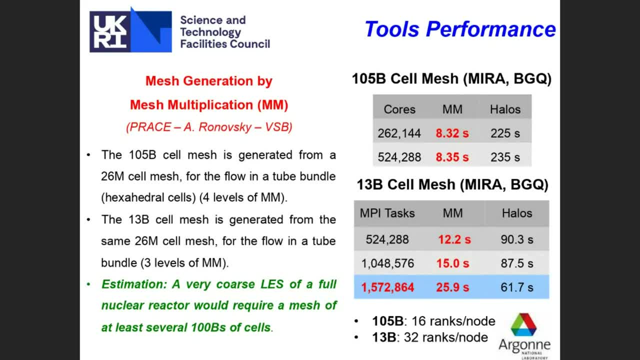 So then, for 13 billion cell mesh, we got timing, Actually. I mean, we've been tested up to the full machine, Half of the full, Yeah, Yeah, the full machine, but using some hyper-threading, And so that as well, is quite fast. 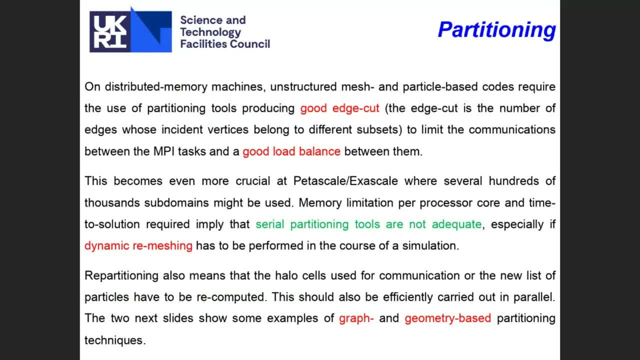 So now that we got the mesh, We need to distribute this over the process. So there are two main techniques. There are very intuitive one, which is geometry base. So you, I mean, I'll explain a little bit later how it works. 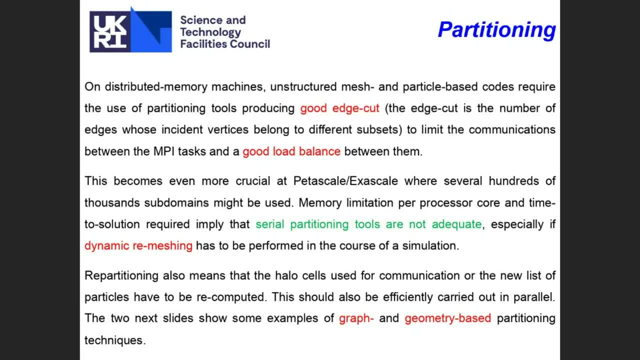 And the second one is a graph based. So you basically extract the graph of the mesh And what you want to do is that you want to actually distribute evenly the load per processor, But you want also to reduce the communication between processors, Because this communication can also really really damage. 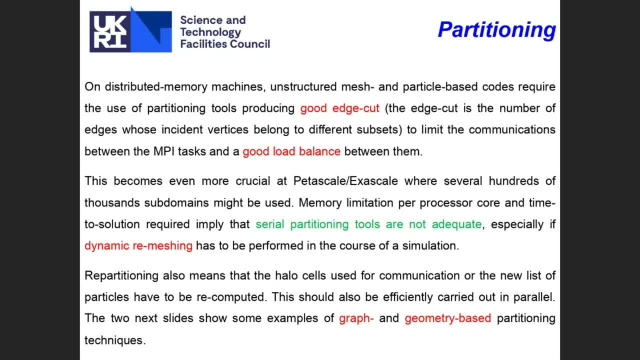 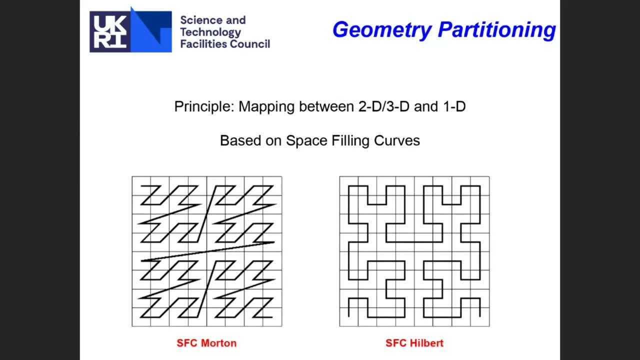 the performance of the simulation. So, going further, one of the geometry partitioning technique used is based on space filling curves, So here you could see 2D examples. So, starting from two squares, what you want? you want the mapping between the 2D of the corresponding 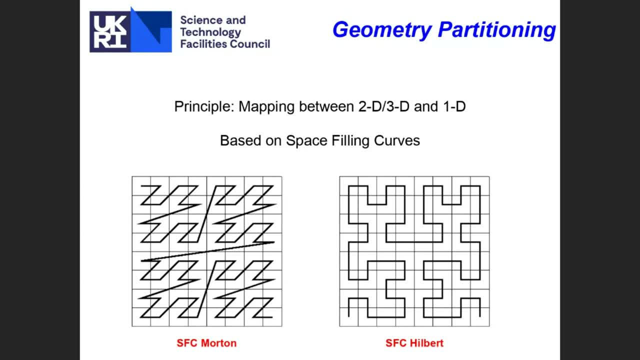 to the squares into 1D. So basically this line- Morton and Hilbert- a 1D line is just a very long array And if you have 16 processors, you just, you know, just have to do it. 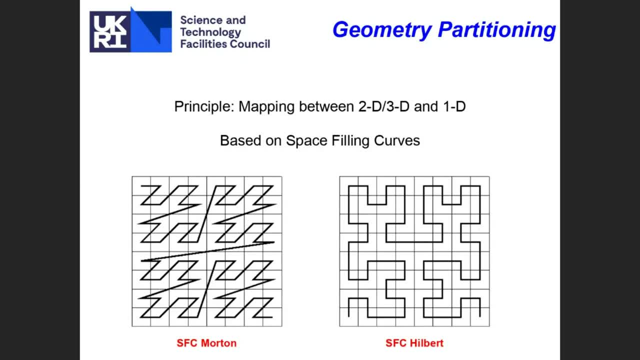 you just chop, equally or evenly, this line and each processor is going to run a chunk of this, of these arrays. so tomorrow we're going to test different these two approaches for the, for the tube model test case, and you could, you would be able to compare the timings and what usually affects the timings: the. 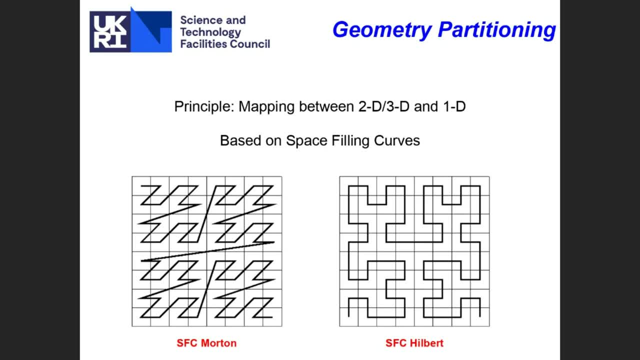 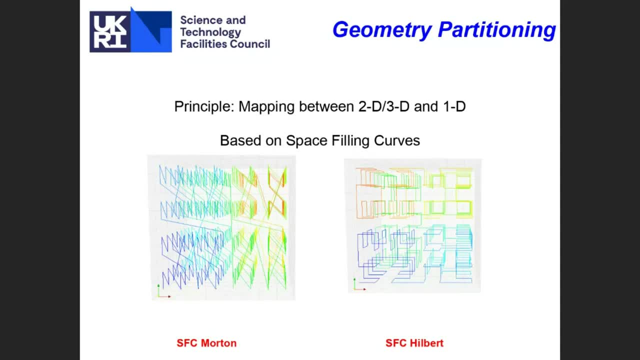 communication between processors. so this is for the geometry partitioning. in real life it looks a little bit like this: the colors correspond to the index of the processors, so it goes from blue, which is zero, I guess, to red, which is a maximum number of processors, and you can see the, the Morton shape, which is called also Z. 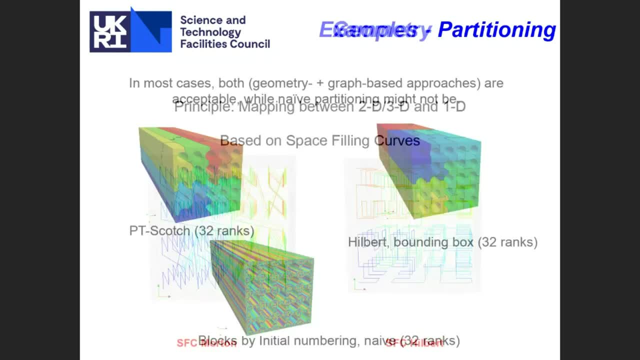 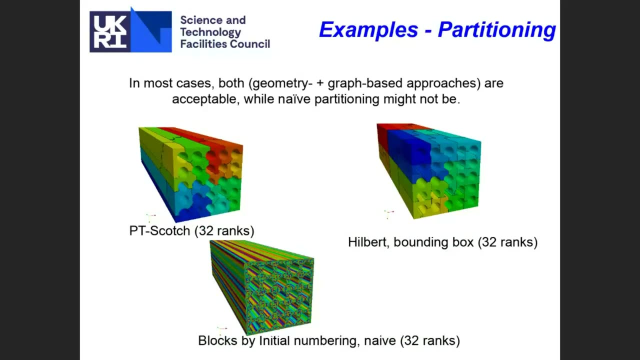 shape and the Hilbert shape on the right hand side. so now I don't detail here the given any more detail about the graph based approaches, but you can see that on the left hand side, the top left hand side, pittyscotch, which is a solver library which allows to partition using a graph. 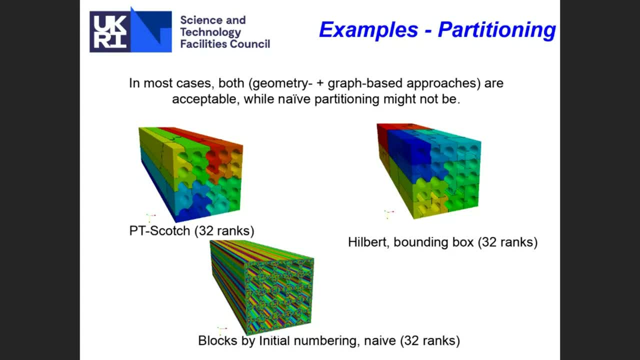 graph based techniques. so you can see the example on 32 ranks or MPI task, of course, and and the example compared to for Hilbert. so you can you can see that the shape of the subdomains are a little bit different, but now, if you use what is, 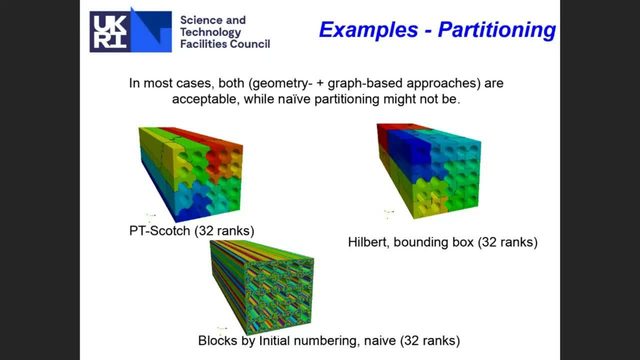 called a naive numbering. without any of this treatment you end up at the bottom of the slide with with all the color all over the places. so basically all the all the red on the at the bottom correspond to what is run on one processor. so you can imagine it looks like. I mean in that situation all the processors are going to talk to each other. 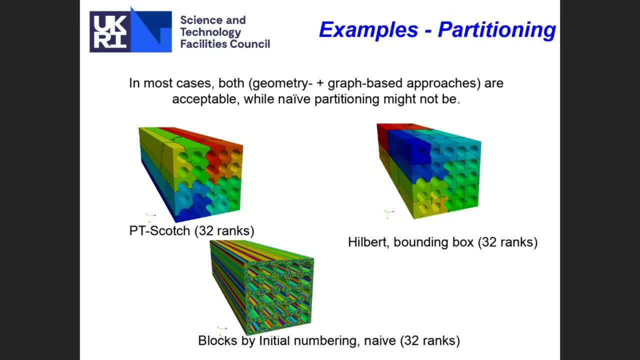 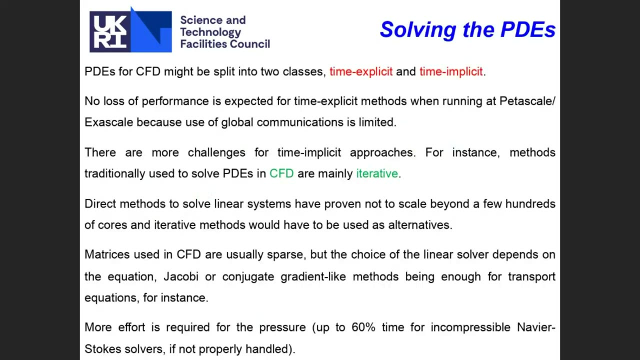 so this is going to very, very slow down the simulation. so the two first techniques on the top I mean, are to be chosen if you want to get good performance out of the machine on the code. so now, if we go to solving the pdes, is that they? I mean, in CFD you got two classes, mainly that, the 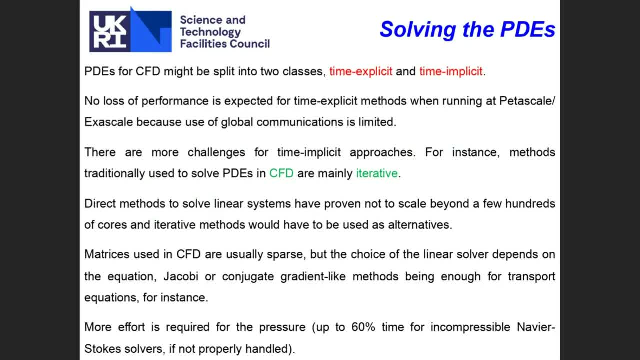 the time explicit and the time implicit. so there shouldn't be any problem to run a time explicit simulation at the exact scale and basically to get good performance out of it. because the, the, the data, I mean the- when you, when you compute the kernel, the data are very localized when you go. 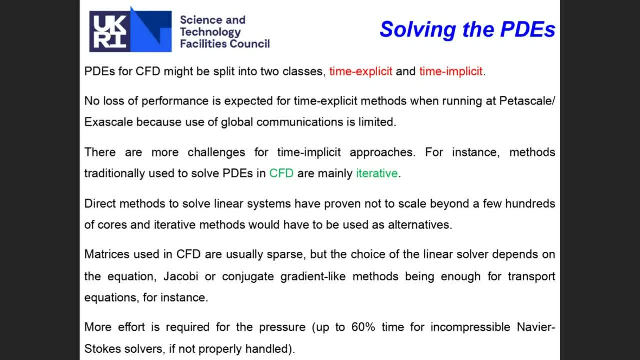 into the time, implicit. you end up solving matrices and then, in the case of the matrices are very, very sparse. so you, you don't get much out of the performance of the machine and you depend a lot on global communication. so, in Saturn, a few years back, about sixty percent of the time where we spent in 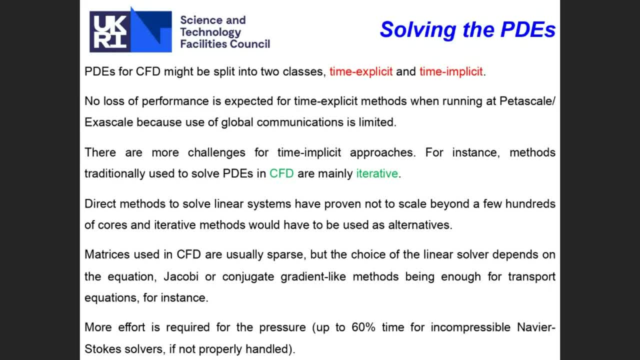 in a computing the process and in the same way in other other systems. we spent a lot of time in the computing the process and in the same way in other other systems. we spent a lot of time in the the pressure now I mean because there have been a lot of improvements. 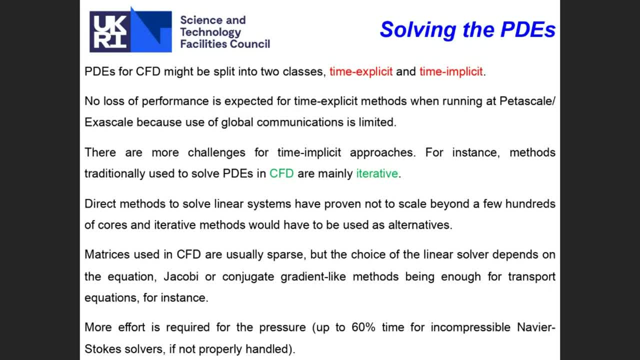 developing the multi, multi grid methods. this is probably down to two to thirty percent, and the velocity is a bit more costly now because it's it's all computed implicit. so you've got a block matrix with UVW there and another part which is quite costly in solving the. the equation correspond to what is called 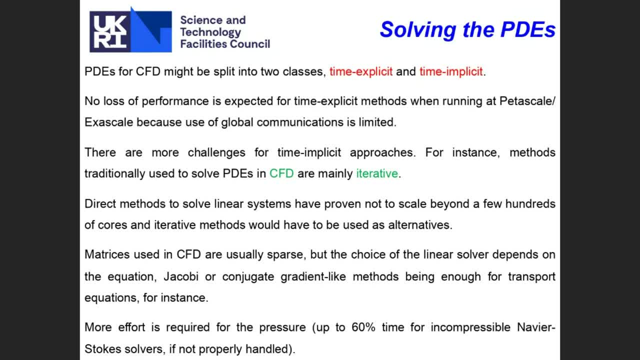 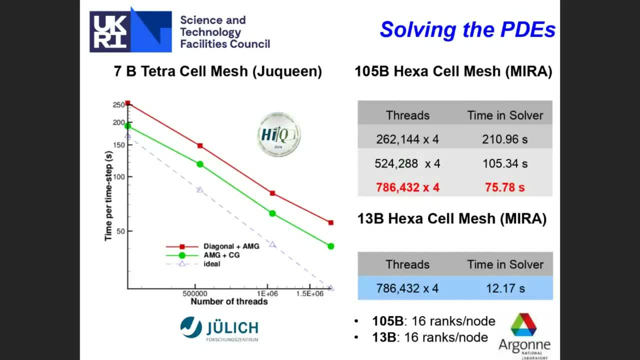 gradient reconstruction when you go up cells which are very skewed in the mesh. so but if we tested the, the code on different machine in this case they are blue jeans and they, they've been tested up to the full machine. and they are blue jeans and they, they've been tested up to the full. 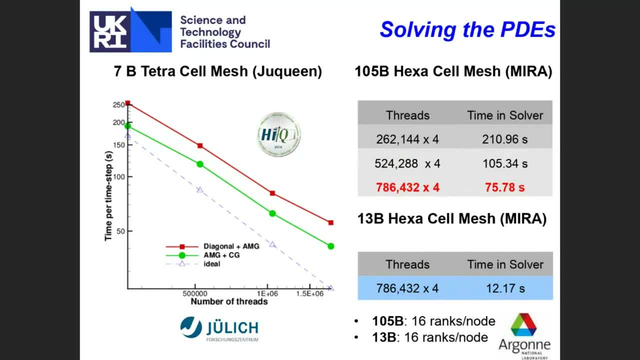 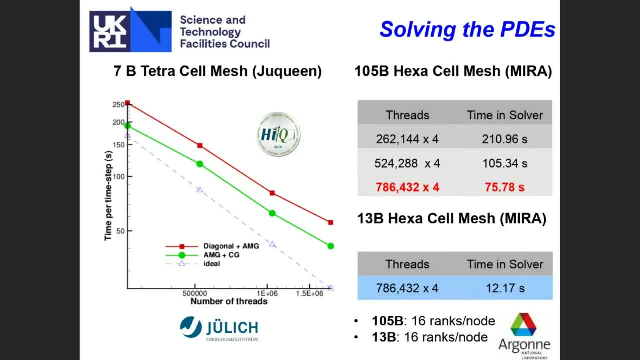 left-hand side. that shows the time to left-hand side. that shows the time to solution which a and the dashed line solution which a and the dashed line solution which a and the dashed line correspond to the ideal time to solution. correspond to the ideal time to solution. correspond to the ideal time to solution. and you can see that the slope is nearly, and you can see that the slope is nearly, and you can see that the slope is nearly the same and you get a very good speed. the same and you get a very good speed. 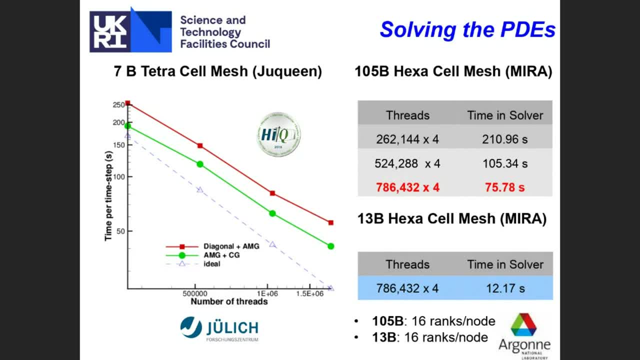 the same and you get a very good speed up now if you look at the largest mesh up now. if you look at the largest mesh up now, if you look at the largest mesh with 105 billion cells, you also got a. with 105 billion cells, you also got a. 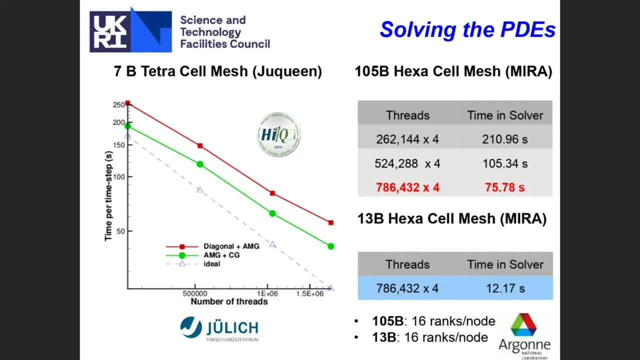 with 105 billion cells. you also got a very good speed up in a solver. you know very good speed up in a solver. you know very good speed up in a solver. you know the time, the time span in the solver i. the time the time span in the solver i. 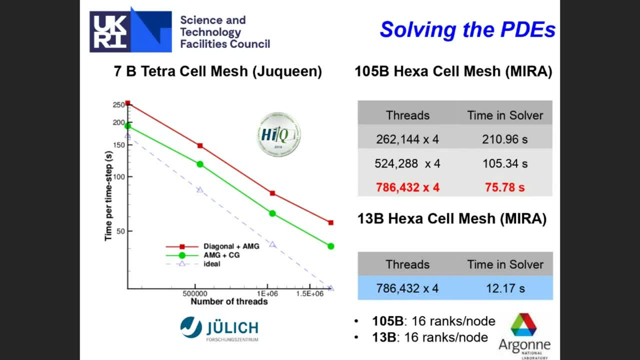 the time, the time span in the solver, i mean if you go from mean, if you go from mean, if you go from the the the first line 20, 60 000. the, the, the first line 20, 60 000. the, the, the first line 20 60 000, multiplied by four to five twenty four. 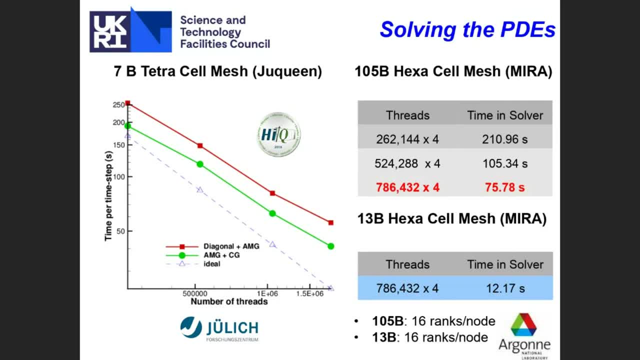 multiplied by four to five. twenty four multiplied by four to five. twenty four multiplied by four, you got a speed up of multiplied by four. you got a speed up of multiplied by four. you got a speed up of two and i and from the the first column, two and i and from the the first column. 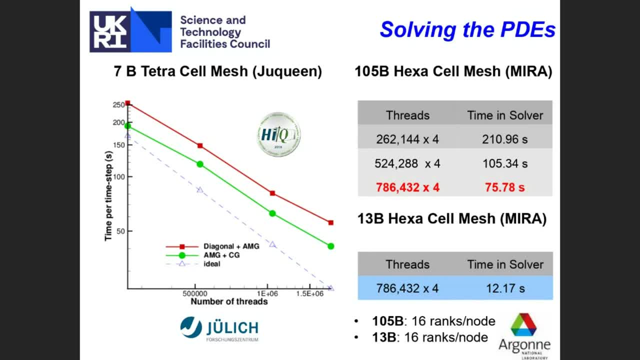 two and i, and from the the first column to the third one, you got to speed up to the third one, you got to speed up to the third one, you got to speed up about, uh, 1.9 tears. no, yeah, 2.2.90. so 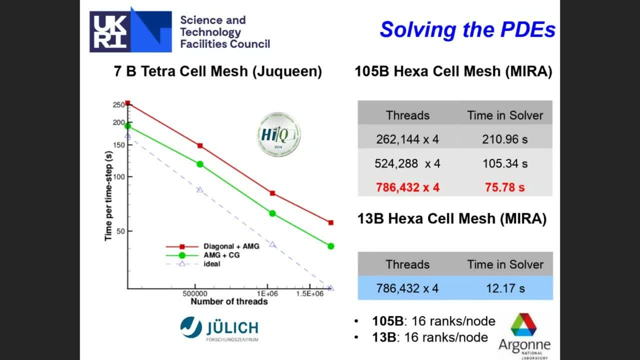 about uh 1.9 tears? no, yeah, 2.2.90. so about uh 1.9 tears? no, yeah, 2.2.90. so almost three, which is to be expected. so almost three, which is to be expected. so almost three, which is to be expected. so the, the, the, the solver scales, very, very. 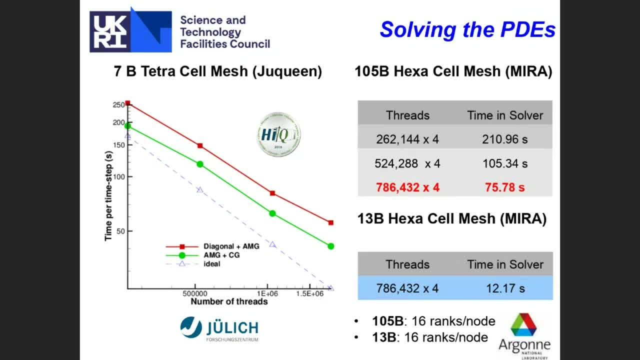 the, the the solver scales, very, very, the, the the solver scales very, very well, well, well, and, and so, and four, four times i mean and, and so, and four, four times i mean and, and so, and four, four times i mean: eight, eight thousand is about three. eight, eight thousand is about three. 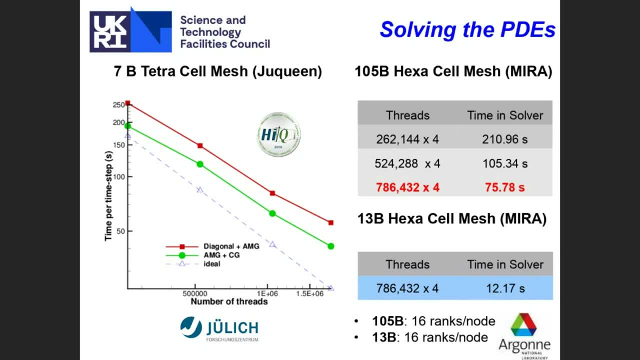 eight thousand is about three million, so that's that's the highest number. million, so that's that's the highest number. million, so that's that's the highest number of uh mpi tasks. of course that the of uh mpi tasks. of course that the of uh mpi tasks. of course that the code's been tested on. 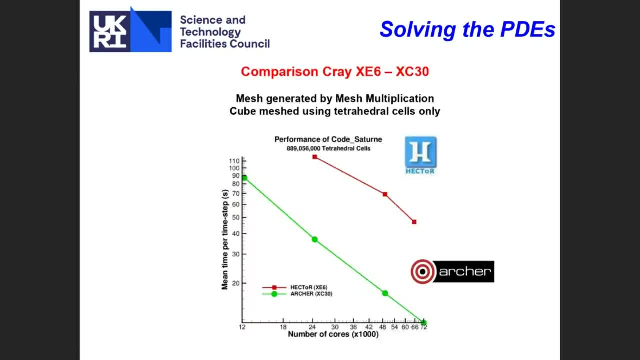 code's been tested on. code's been tested on, and that was already a few years back. now i i don't have the results on archer. now i i don't have the results on archer. now i i don't have the results on archer too, because 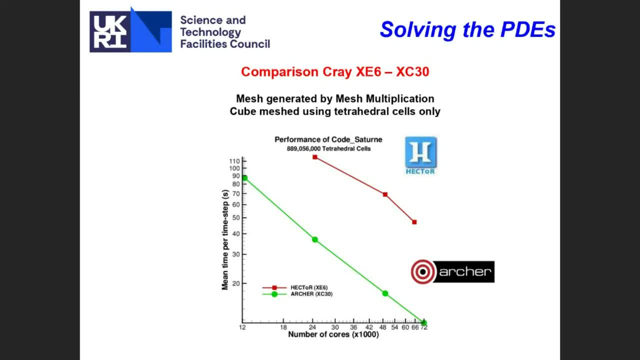 too, because, too, because we, i mean the- the machine is not fully. we i mean the the machine is not fully. we, i mean the the machine is not fully installed yet and we would like to have installed yet, and we would like to have installed yet and we would like to have the the, the. the results on the. on the. 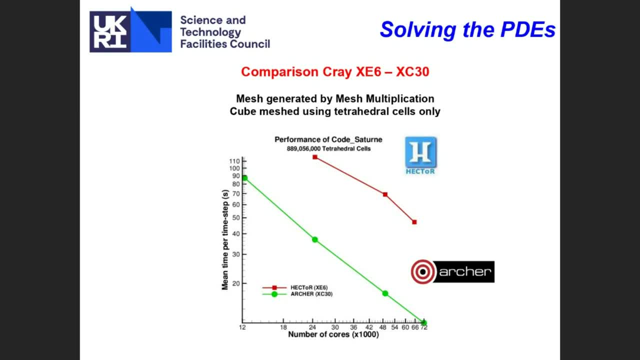 the, the results on the, on the on the full machine, but i mean full machine, but i mean full machine, but i mean this is a comparison between uh archer, this is a comparison between uh archer. this is a comparison between uh archer, which was uh just the commission and the. 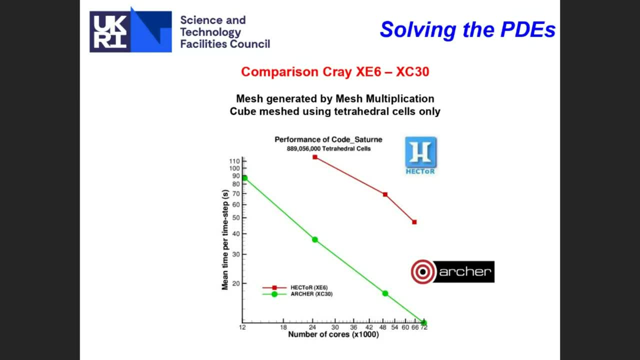 which was uh, just the commission, and the, which was uh, just the commission and the machine before. and we were going machine before and we were going machine before and we were going two to three times faster, two to three times faster, two to three times faster. now, on archer two, 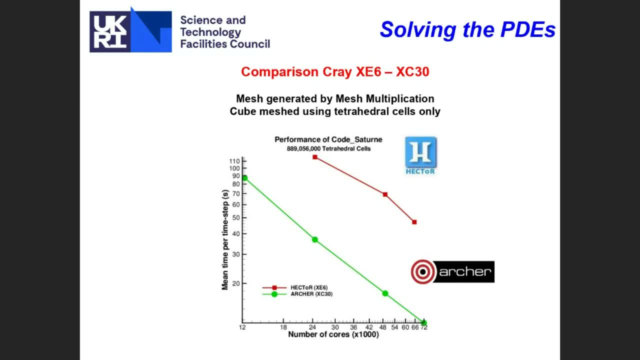 now on archer two. now on archer two, we run up to, we run up to, we run up to 32 or 64 nodes, 32 or 64 nodes, 32 or 64 nodes, no 256 nodes and we could see that. no 256 nodes and we could see that. 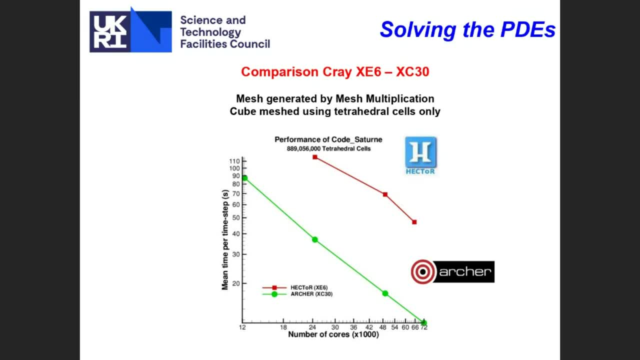 no 256 nodes, and we could see that, comparing to 256 nodes on archer, we comparing to 256 nodes on archer, we comparing to 256 nodes on archer, we were going about four times faster, which were going about four times faster, which were going about four times faster, which is a very good and 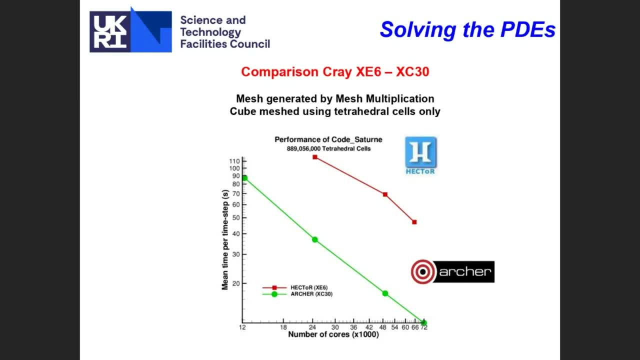 is a very good and is a very good, and and the time to solution has got the same and the time to solution has got the same and the time to solution has got the same pattern as this one, but i mean pattern as this one, but i mean. 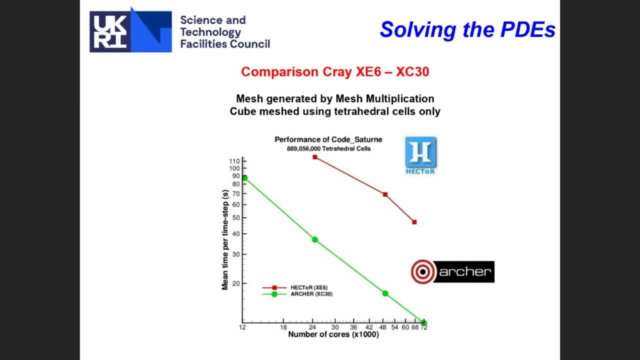 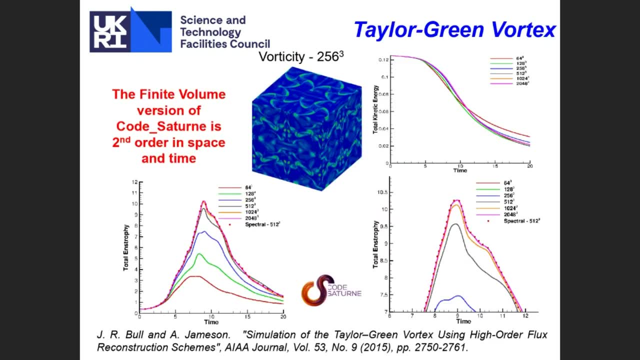 pattern as this one, but i mean: in a few months we get the. i mean in a few months we get the. i mean in a few months we get the. i mean the similar plots comparing uh to archer, the similar plots comparing uh to archer, the similar plots comparing uh to archer. nature too. 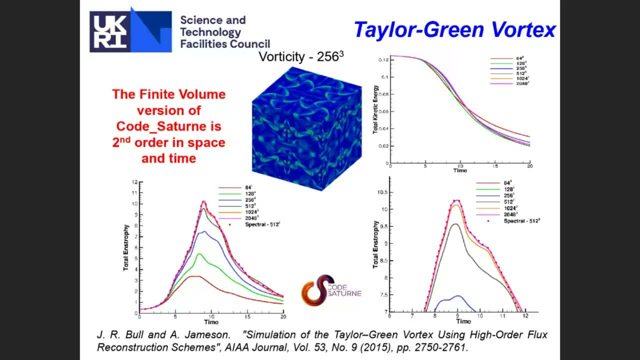 so i mean performance is important. but so i mean performance is important, but so i mean performance is important. but accuracy is also very important. so accuracy is also very important. so accuracy is also very important. so called saturn is called finite volume. called saturn is called finite volume. 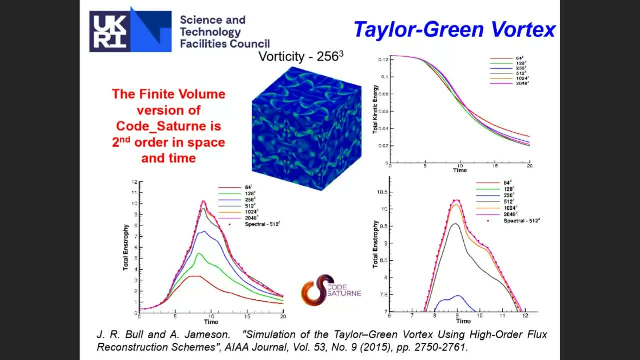 called saturn, is called finite volume, and and and and. the the best can be achieved with the, the the best can be achieved with the. the the best can be achieved with the secondary in space and time. secondary in space and time, secondary in space and time. so there's a test case called the. 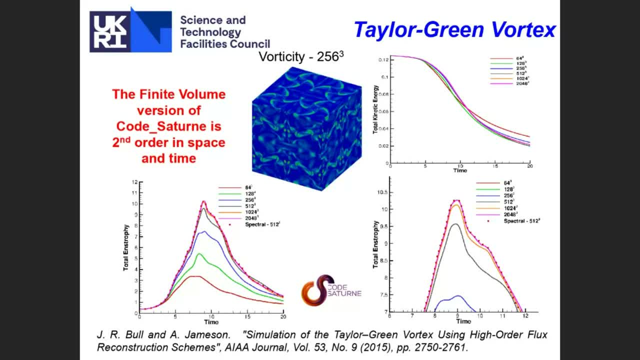 so there's a test case called the. so there's a test case called the. the terror green vortex test case, the terror green vortex test case, the terror green vortex test case, and some simulations have been run there and some simulations have been run there and some simulations have been run there up to 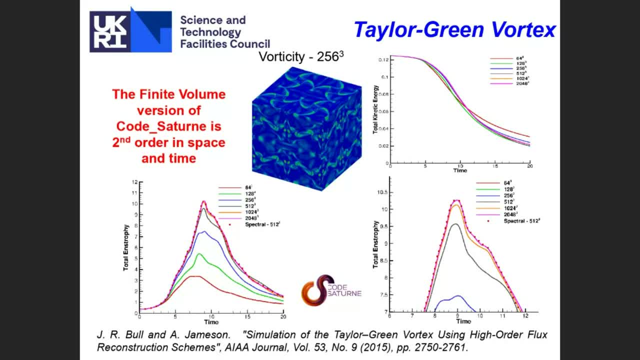 up to up to 2000 cube, so it's about 8 billion cells 2000 cube. so it's about 8 billion cells 2000 cube. so it's about 8 billion cells. and that's what is needed to, and that's what is needed to. 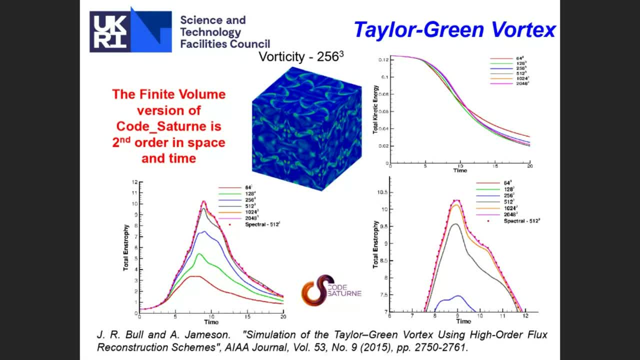 and that's what is needed to to recover spectral accuracy. so that's to recover spectral accuracy. so that's to recover spectral accuracy. so that's on the, on the, on the, the, the maximum on the right hand side, the, the maximum on the right hand side, the, the maximum on the right hand side, and this is also expected, given the. 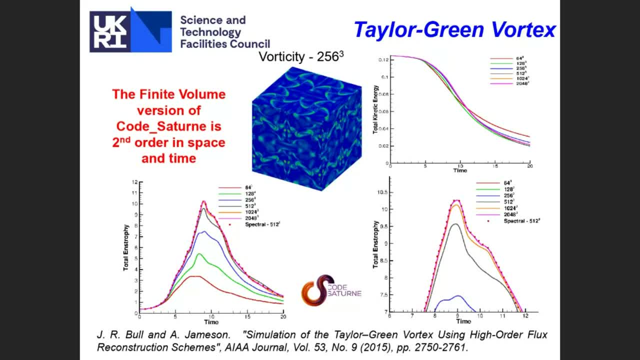 and this is also expected given the. and this is also expected given the. i mean the, the the best order of accuracy. i mean the, the the best order of accuracy. i mean the, the the best order of accuracy we can get. we can get, we can get in concert. but i mean, if you want to run, 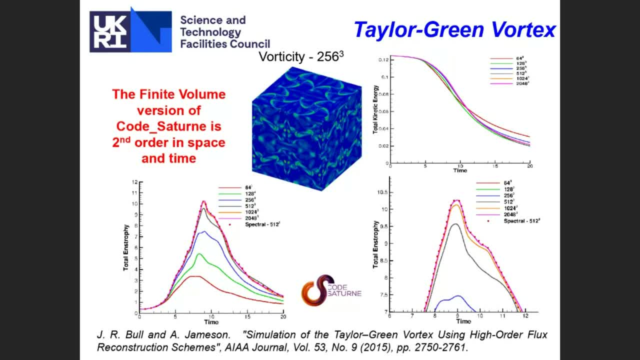 in concert. but i mean, if you want to run in concert, but i mean if you want to run simulation which are only with exide simulation, which are only with exide, simulation which are only with exide while cells and in a box, while cells and in a box. 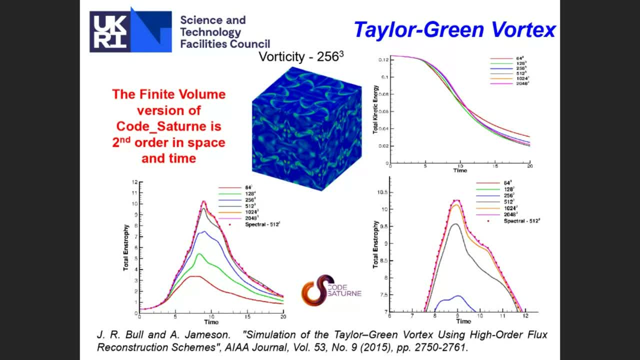 while cells and in a box. i mean construction might not be the best. i mean construction might not be the best. i mean construction might not be the best software to use. you should use a software to use. you should use a software to use. you should use a dns of software with a much, much higher. 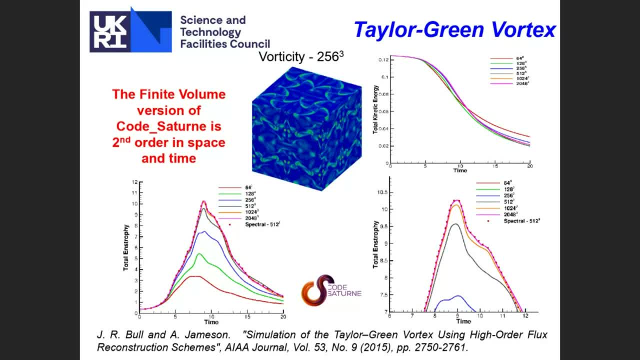 dns of software with a much, much higher dns of software with a much, much higher accuracy, accuracy, accuracy: now, if you are going for more complex, now, if you are going for more complex, now if you are going for more complex geometries, that will flow between geometries, that will flow between 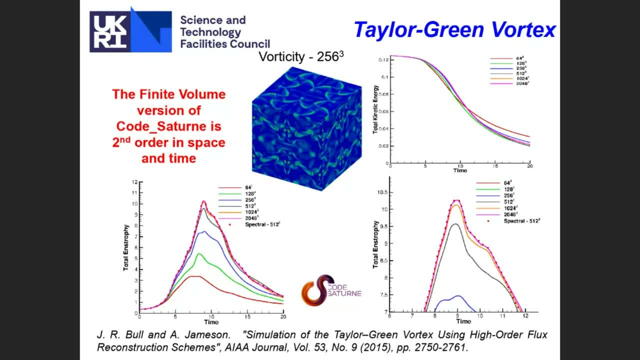 geometries that will flow between tube bundles saturn is a good one and tube bundles saturn is a good one. and tube bundles saturn is a good one. and and retain this second order. accuracy in: and retain this second order. accuracy in: and retain this second order accuracy in space and time. 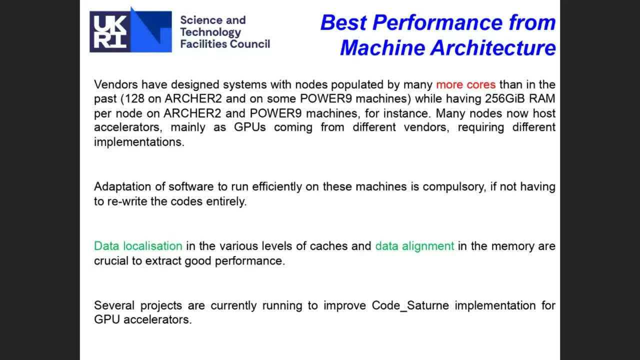 space and time, space and time. so now. another issue is that the so now. another issue is that the so now. another issue is that the, the architecture of the computers evolve. the architecture of the computers evolve. the architecture of the computers evolve all the time, all the time. 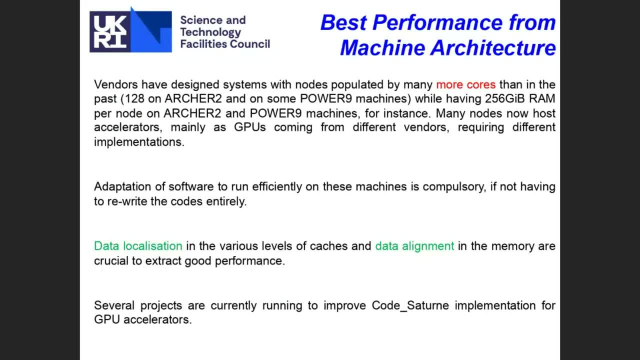 all the time. so, but a trend, so, but a trend, so, but a trend which is common to all this architecture is that it common to all this architecture is that it common to all this architecture is that it increased the number of cores, increased the number of cores. 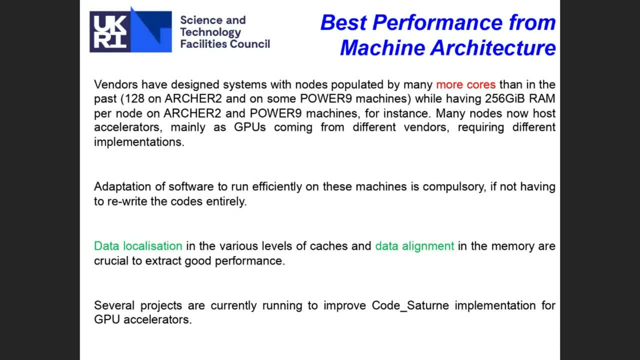 increased the number of cores per node at the point that a few years per node, at the point that a few years per node, at the point that, a few years back, back back, when you were bidding for time, you, you, when you were bidding for time, you, you. 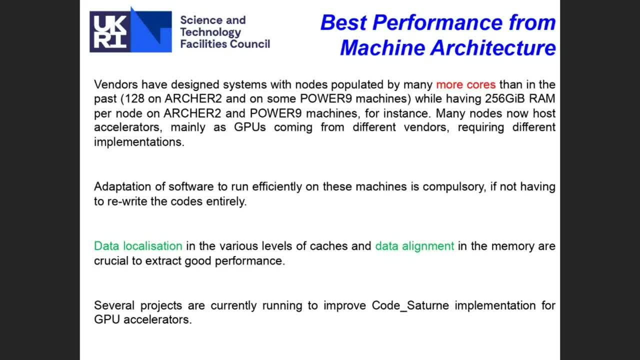 when you were bidding for time, you, you were asked for the number of cores. you were asked for the number of cores. you were asked for the number of cores. you were using and paid and you were paying, were using and paid, and you were paying, were using and paid and you were paying on that. now, you, you, you pay. 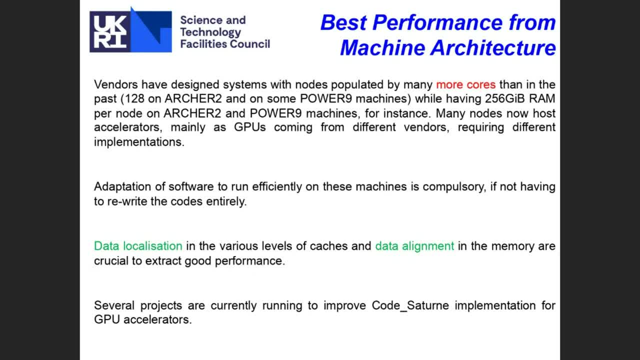 for the number of nodes you are using. for the number of nodes you are using. for the number of nodes you are using because the nodes can can, because the nodes can can, because the nodes can can. contain cpus accelerators. contain cpus accelerators. contain cpus accelerators, only cpus, a mix of both. 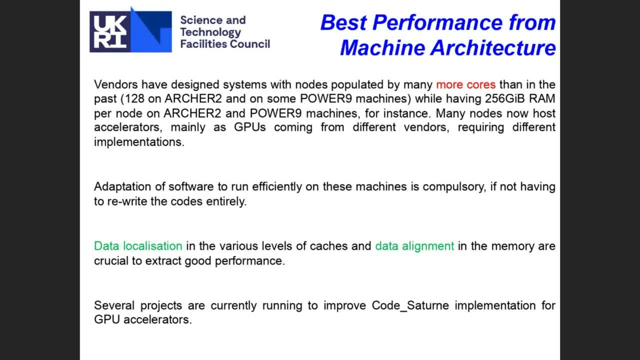 only cpus, a mix of both, only cpus, a mix of both, gpus so. but for instance, on archer 2, gpus so. but for instance on archer 2 gpus so. but for instance on archer 2, you've got 128 cores on. 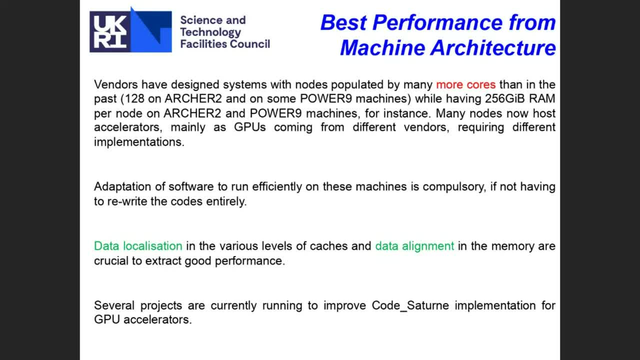 you've got 128 cores on. you've got 128 cores on per node, which is sufficient to run the per node, which is sufficient to run the per node, which is sufficient to run the relatively large simulation. we're going relatively large simulation. we're going relatively large simulation, we're going to. 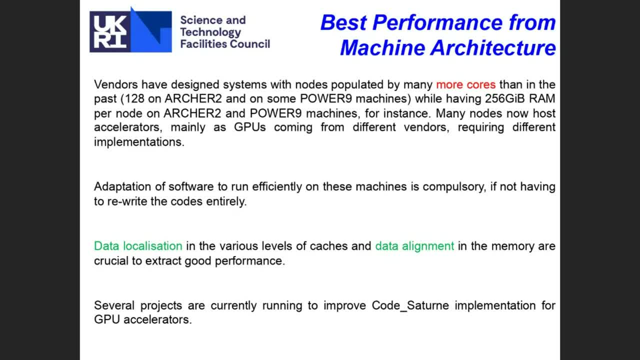 to to you are going to run later, and it's you are going to run later and it's you are going to run later, and it's also the same on, also the same on, also the same on on other actually architecture from other, on other actually architecture from other. 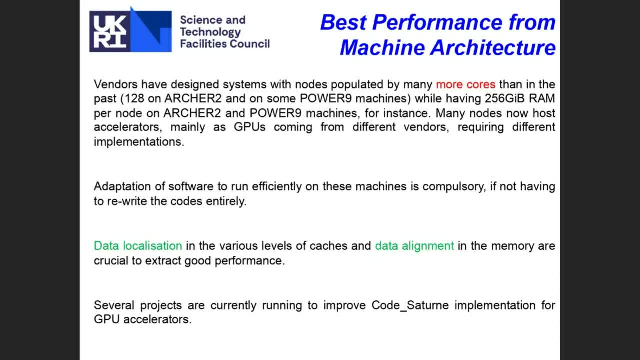 on other actually architecture from other vendors, vendors, vendors, and their trend is also to have quite a, and their trend is also to have quite a, and their trend is also to have quite a lot of ram, lot of ram, lot of ram. but you know there is, so you need to. 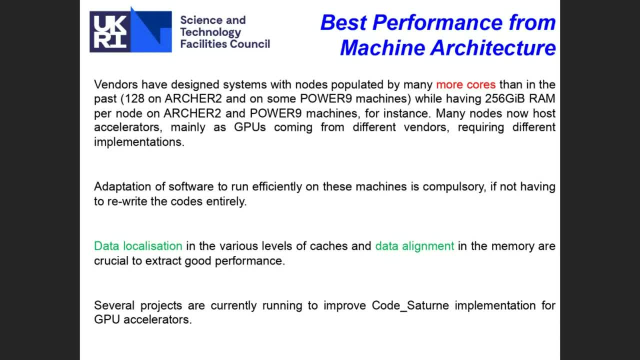 but you know there is, so you need to, but you know there is, so you need to prepare the code for this architecture, prepare the code for this architecture, prepare the code for this architecture, but also, but also, but also, things that you, you need to prepare it, things that you, you need to prepare it. 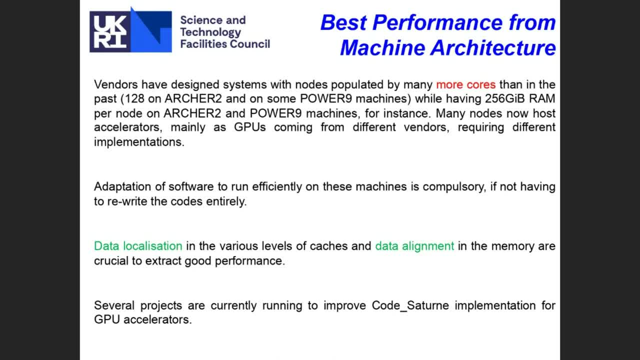 things that you, you need to prepare it for, for for accelerators. so in in saturn there are accelerators. so in in saturn there are accelerators. so in in saturn there are some efforts to, some efforts to, some efforts to to put on gpu accelerators. so a few. 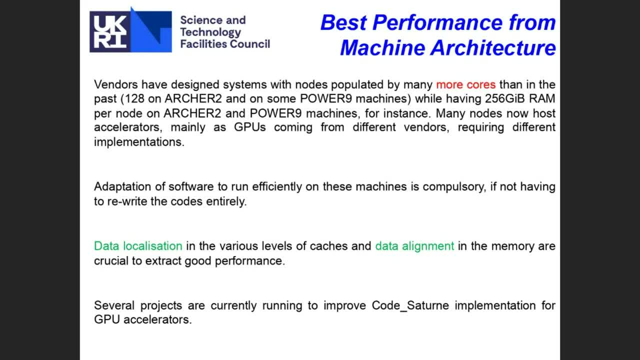 to put on gpu accelerators, so a few to put on gpu accelerators, so a few. years back, um years back, um years back um, a colleague for by bm, a colleague for by bm, a colleague for by bm port put it: a good chunk of the code. 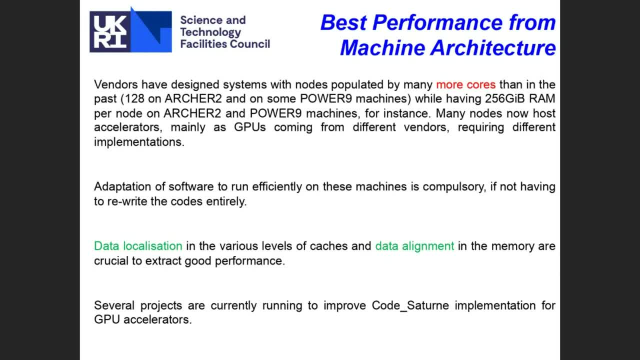 port put it a good chunk of the code. port put it a good chunk of the code there, there, there and for the for the solvers, and what and for the for the solvers and what and for the for the solvers and what. what has been worked on is accelerating. 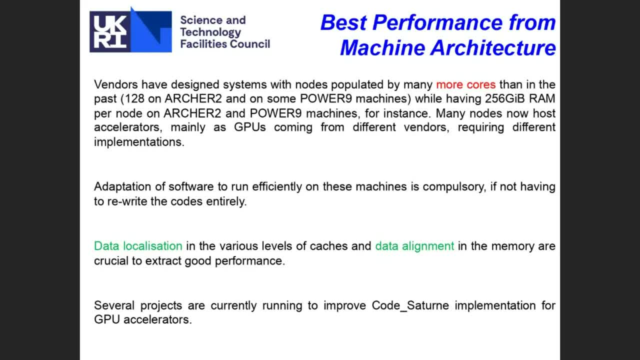 what has been worked on is accelerating. what has been worked on is accelerating the gradient reconstruction, as i, the gradient reconstruction, as i, the gradient reconstruction, as i mentioned before. so these are some results which were so. these are some results which were so. these are some results which were obtained on a summit. so that was a 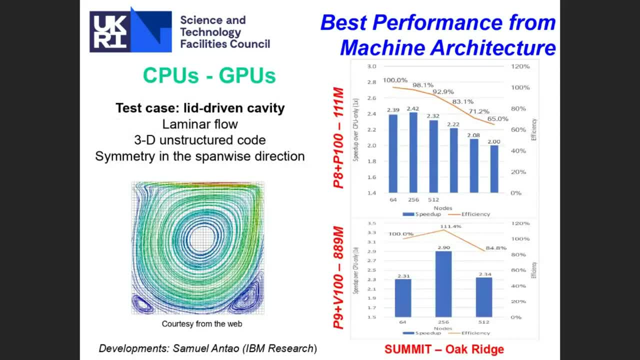 obtained on a summit, so that was a. obtained on a summit, so that was a second machine listed in the. in the top second machine listed in the. in the top second machine listed in the. in the top three machine: three machine. three machine and and and the. the code was tested up to 512. 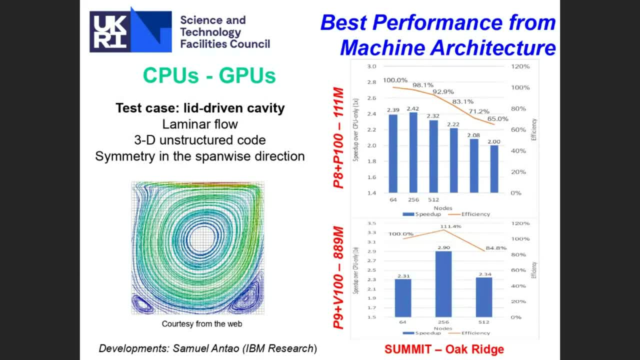 the? the code was tested up to 512. the- the code was tested up to 512. nodes of the machine. so you multiply by nodes of the machine. so you multiply by nodes of the machine, so you multiply by six, six, six to get the number of um. 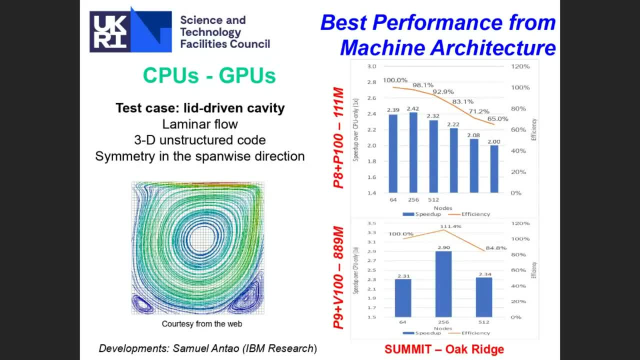 to get the number of um, to get the number of um of gpu which were, which were used, of gpu which were, which were used, of gpu which were, which were used. so it's about uh three, three thousand. so it's about uh three, three thousand. so it's about uh three, three thousand gpus which was. 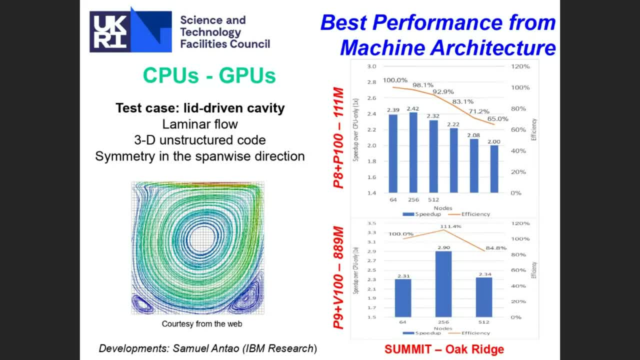 gpus, which was gpus, which was quite a lot and quite a lot and quite a lot, and the current comparison between cpu and the current comparison between cpu and the current comparison between cpu and gpu was giving a speed up about uh. gpu was giving a speed up about uh. 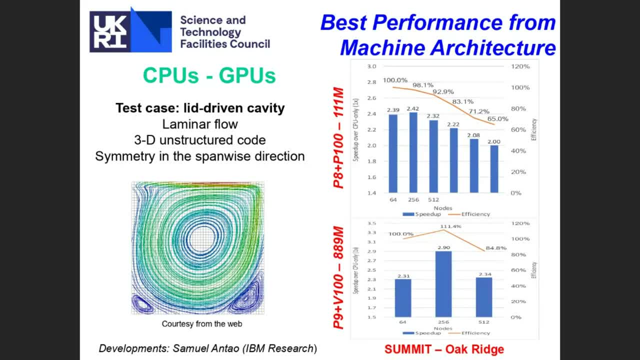 gpu was giving a speed up about uh between two to three, which is in the between two to three, which is in the between two to three, which is in the range of the other application being range of the other application being range of the other application being run on this software. 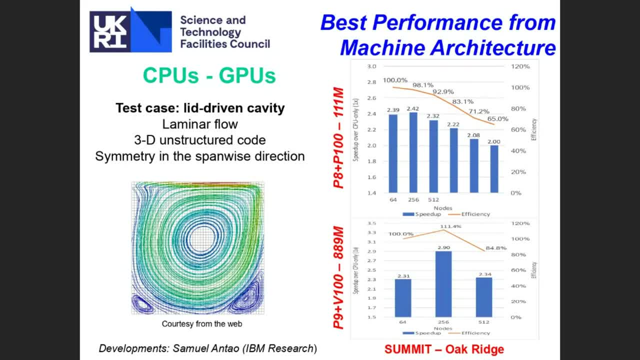 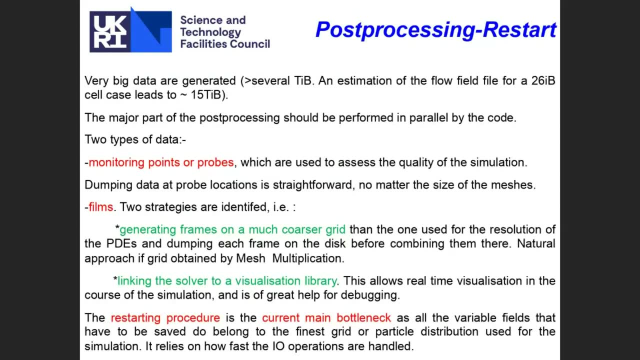 run on this software, run on this software, on, on on these machines. so now come the the the tricky bits. so now come the the the tricky bits. so now come the the the tricky bits. because because, because usually a a lot of time is invested in, usually a a lot of time is invested in. 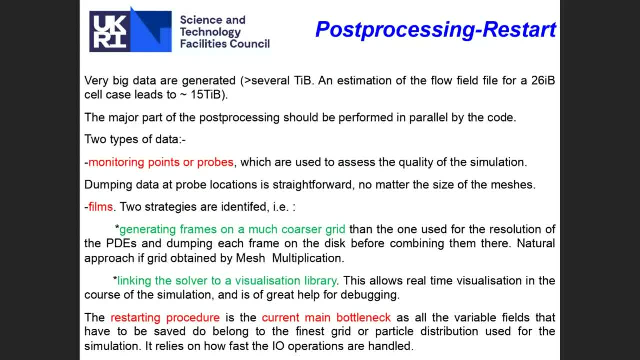 usually a a lot of time is invested in, in, in, in, in, in developing software and optimizing developing software and optimizing developing software and optimizing software, and a little bit less in software, and a little bit less in software and a little bit less in in ios, in ios. 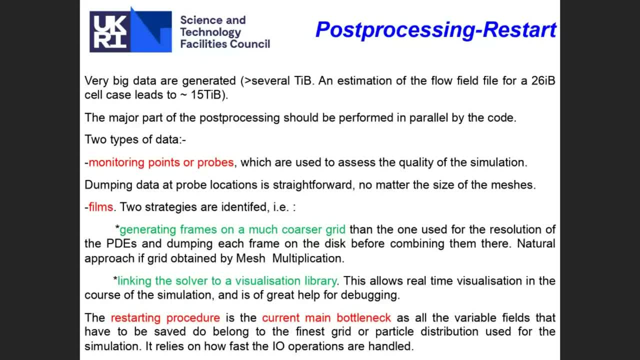 in ios. but but, but if we think about, if we think about, if we think about meshes of meshes of meshes of uh of billion, uh of billion, uh of billion, having billion, billion of cells, i mean having billion, billion of cells. i mean having billion billion of cells. i mean you. you easily end up with a. 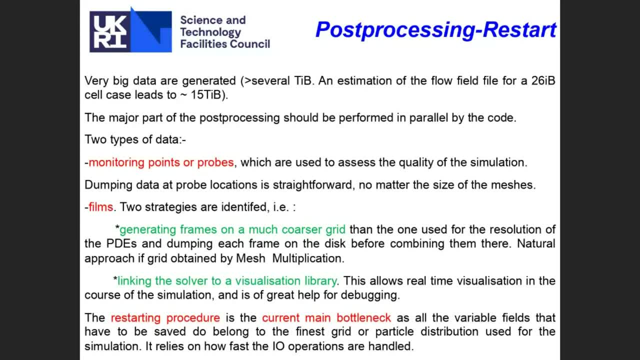 you, you easily end up with a. you, you easily end up with a: 10 to 20 terabytes of data. 10 to 20 terabytes of data, 10 to 20 terabytes of data, so so so, which is probably impossible to move, which is probably impossible to move. 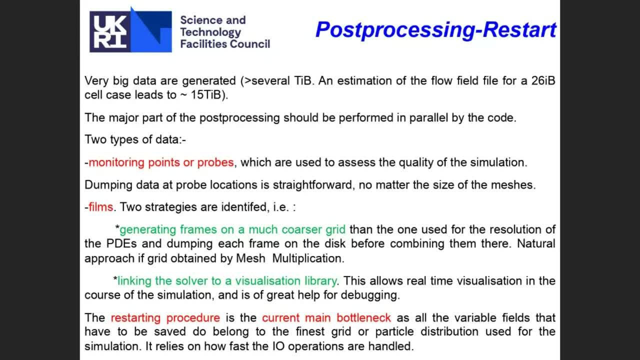 which is probably impossible to move around, basically around, basically around, basically. so, basically in concert, we've got several. so, basically in concert, we've got several. so, basically in concert, we've got several post-processing, post-processing, post-processing aspects. first, the monitoring points and aspects. first, the monitoring points and 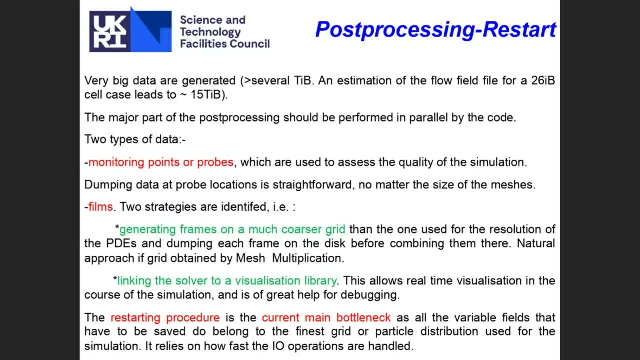 aspects. first, the monitoring points and the probes. so you've been using that in the probes. so you've been using that in the probes, so you've been using that in first tutorial. i think, first tutorial, i think, first tutorial. i think then, then, then you, you, you would like to be able to uh, to. 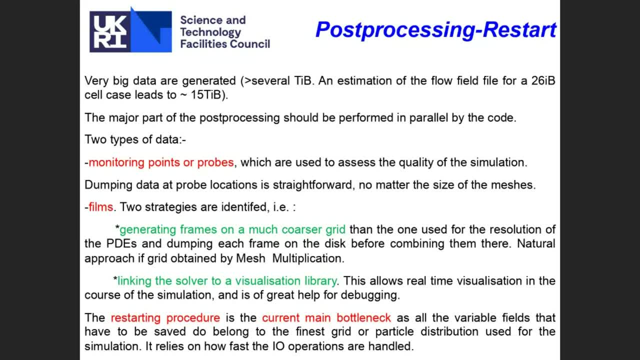 you, you, you would like to be able to uh to you, you, you would like to be able to uh to generate um, generate um, generate um films with you, with your data films, with you with your data films, with you with your data, and for for public engagement, for. 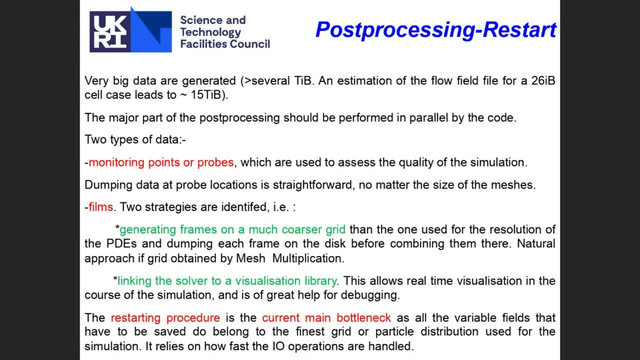 and for for public engagement, for and for for public engagement, for instance, instance, instance, so so. so it's uh very difficult to dump all the. it's uh very difficult to dump all the. it's uh very difficult to dump all the data on the on the disk. 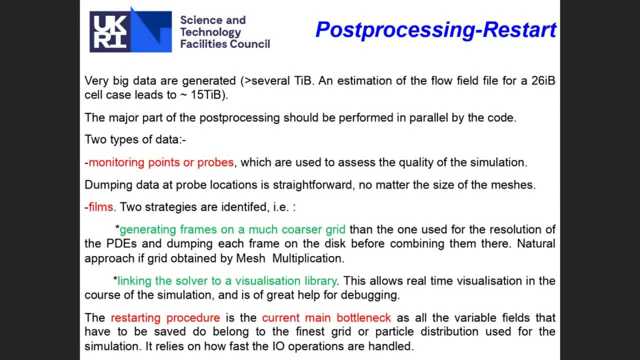 data on the on the disk. data on the on the disk, especially if you run, if you need about, especially if you run, if you need about, especially if you run, if you need about one thousand to two thousand five or ten, one thousand to two thousand five or ten. 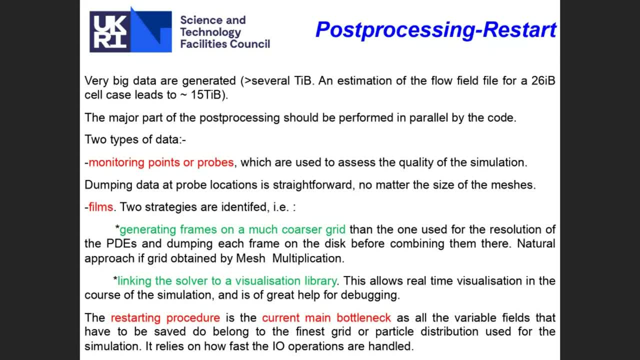 one thousand to two thousand, five or ten thousand instances, thousand instances, thousand instances. so the idea is to generate the frames. so the idea is to generate the frames. so the idea is to generate the frames either on a course, either on a course. either on a course, create and download. 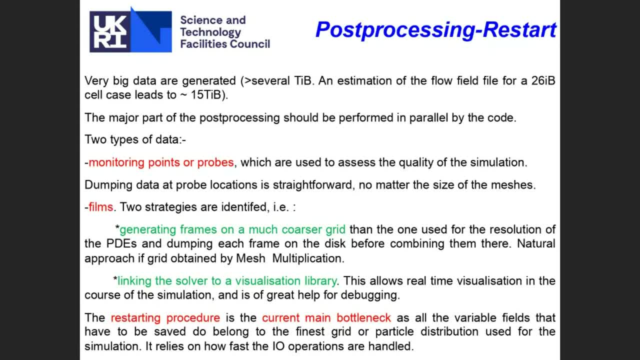 create and download. create and download. dump that on the disk or dump that on the disk or dump that on the disk or to to to present some results on the fly. present some results on the fly. present some results on the fly. so consumption is linked to a library. 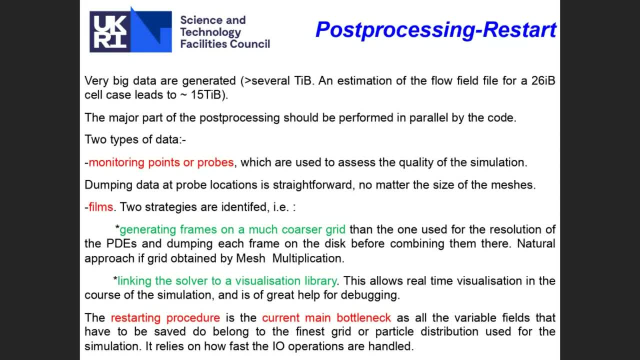 so consumption is linked to a library, so consumption is linked to a library called catalysts, which is also a called catalysts, which is also a called catalysts, which is also a part of a power view, part of a power view, part of a power view, and it's possible to dump png files, which 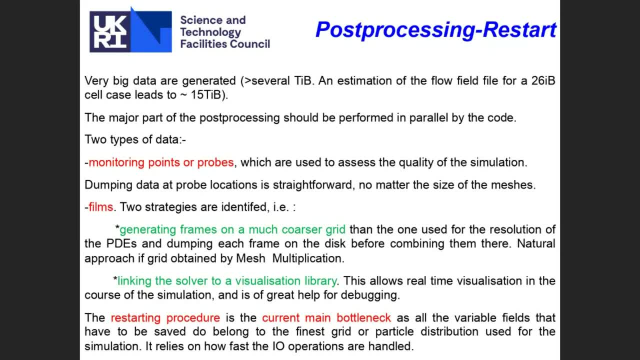 and it's possible to dump png files which- and it's possible to dump png files which are very very, are very very, are very very. i mean very small compared to a, i mean very small compared to a, i mean very small compared to a to a full uh. 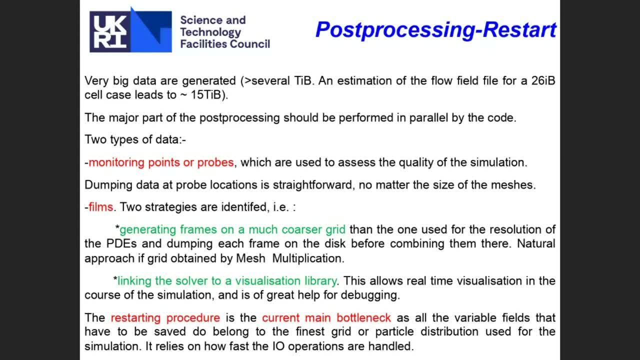 to a full uh. to a full uh. full post processing file. full post processing file. full post processing file. and then these png files are all just. and then these png files are all just. and then these png files are all just gathered and generated film. so maybe gathered and generated film. so maybe. 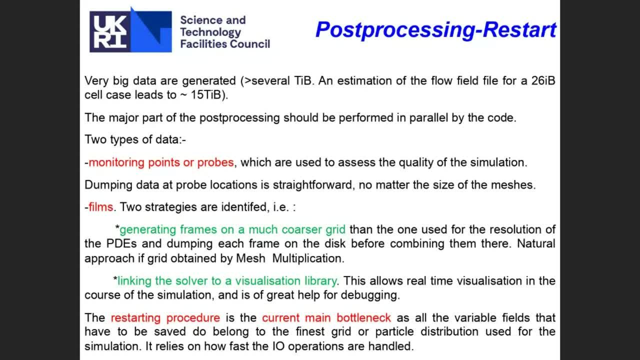 gathered and generated film. so maybe tomorrow, if, if we have time, i can show tomorrow, if, if we have time, i can show tomorrow, if, if we have time, i can show you a video that we you, a video that we you, a video that we we've been building, and so this is this. 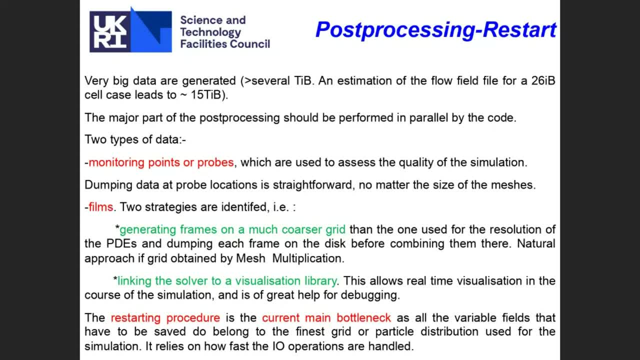 we've been building, and so this is this we've been building, and so this is this way i run, way, i run, way i run on a archer to 98 000 processors, on a archer to 98 000 processors, on a archer to 98 000 processors and doing um the, the plots only on the. 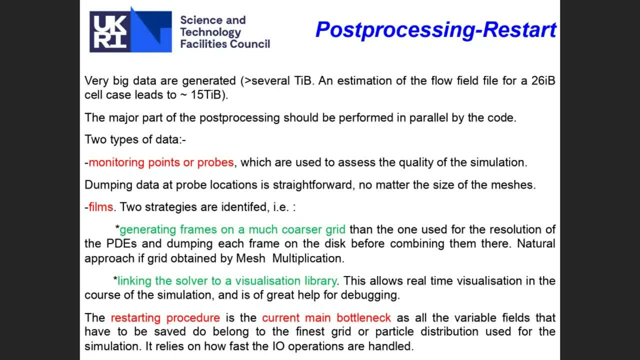 and doing um the, the plots only on the and doing um the, the plots only on the. fly, fly, fly. so, unfortunately, there's a massive. so unfortunately, there's a massive, so, unfortunately, there's a massive bottleneck. which bottleneck, which bottleneck which? which is a, the concert, the restart, or 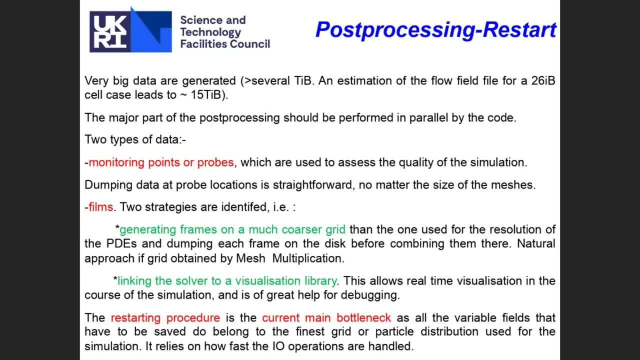 which is a the concert the restart, or which is a the concert the restart, or checkpoint, checkpoint, checkpoint, uh process, uh because they uh process, uh because they uh process, uh because they. there's no other way that we know, there's no other way that we know, there's no other way that we know um. 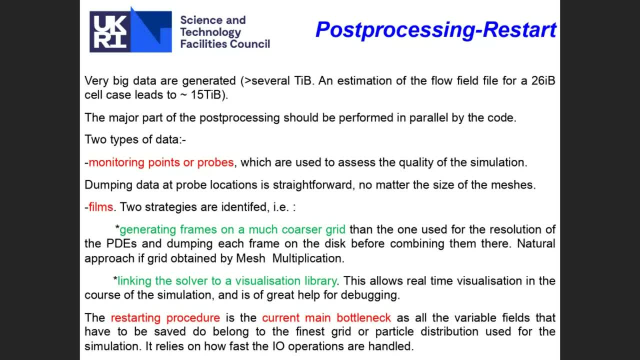 um, um, dumping the full information onto the dumping. the full information onto the dumping, the full information onto the disk, disk, disk. and if we would dump only a part of it, and if we would dump only a part of it, and if we would dump only a part of it, when we would restart the simulation, we 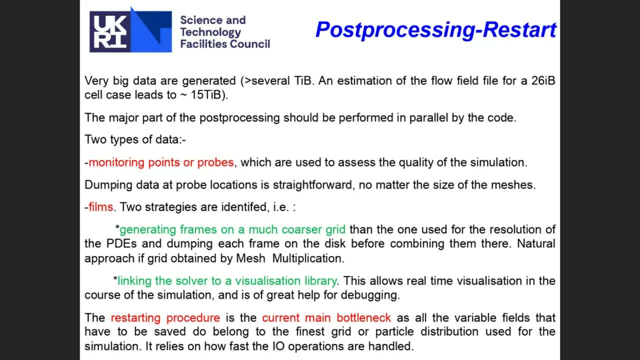 when we would restart the simulation, we, when we would restart the simulation, we would have a transient, would have a transient, would have a transient time, and we would actually lose all the time, and we would actually lose all the time and we would actually lose all the benefit of. 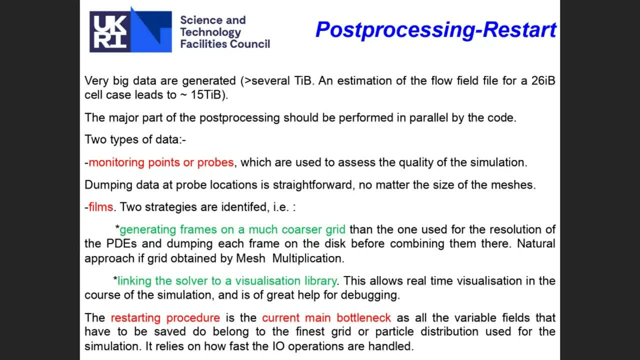 benefit of, benefit of, of, of, of saving less data. so we really need to dump saving less data. so we really need to dump saving less data. so we really need to dump that on the disk, that on the disk, that on the disk. so, in terms of uh. 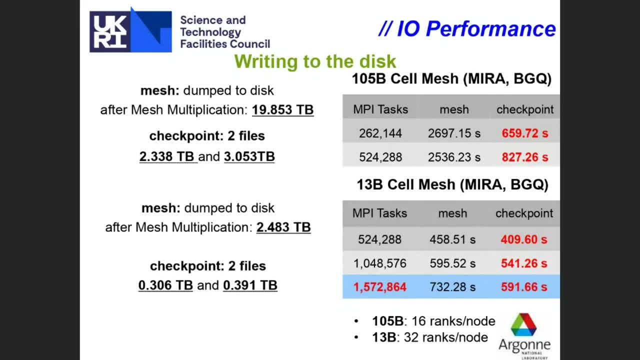 so in terms of uh, so in terms of uh and performance, so and performance, so and performance. so i mentioned that we we ran some tests on. i mentioned that we we ran some tests on. i mentioned that we we ran some tests on using the 105 billion. 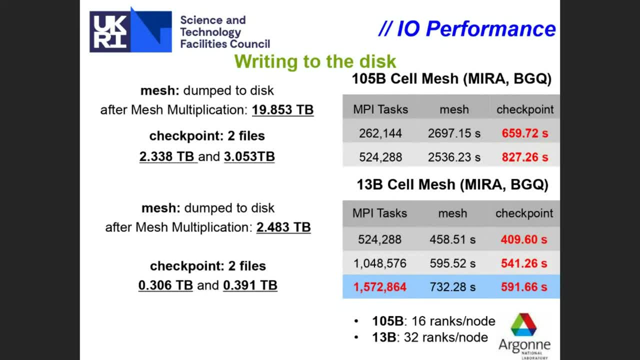 using the 105 billion, using the 105 billion cell mesh, cell mesh, cell mesh. so the mesh size was so the mesh size was, so the mesh size was about 20 terabytes, about 20 terabytes, about 20 terabytes. and the checkpoint files. there are two in 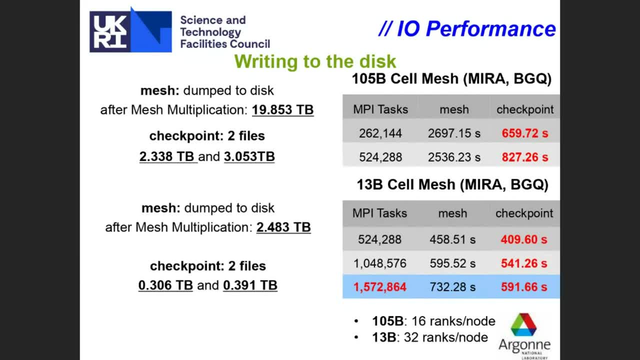 and the checkpoint files. there are two in and the checkpoint files there are two in saturn. so the main one saturn, so the main one saturn, so the main one corresponds to a vw, corresponds to a vw, corresponds to a vw, uvwp, uvwp, uvwp. and the second one 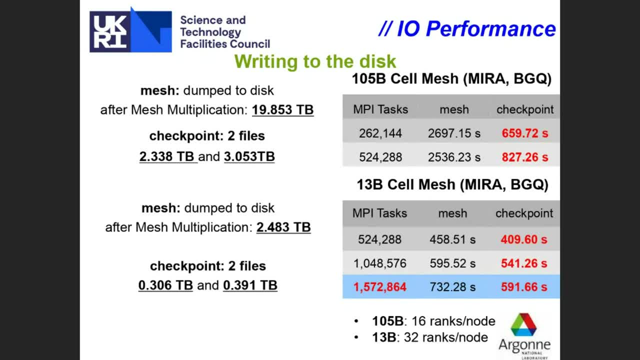 and the second one usually with the extra physics, usually with the extra physics, usually with the extra physics. so so so the? the simulation will run on a. the? the simulation will run on a. the? the simulation will run on a quarter of a million and a half a million. 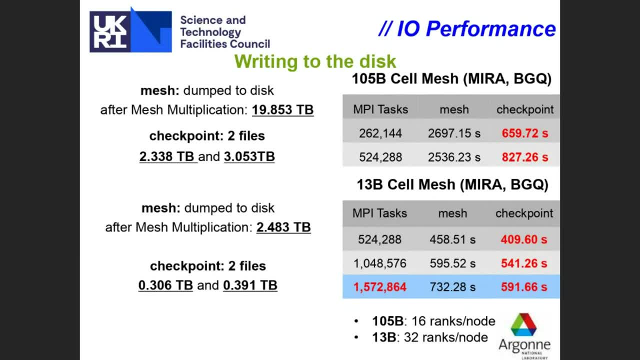 quarter of a million and a half a million. quarter of a million and a half a million mpi tasks and dumping. the mesh was mpi tasks and dumping. the mesh was mpi tasks and dumping. the mesh was taking about. i think it's about 40 taking about. i think it's about 40. 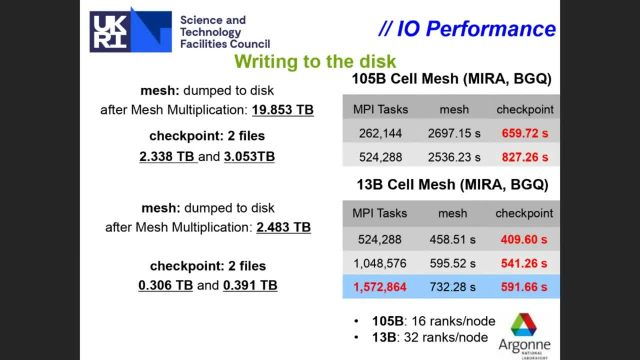 taking about. i think it's about 40 minutes, minutes, minutes. and if you remember that mesh and if you remember that mesh and if you remember that mesh, multiplication was only eight seconds, multiplication was only eight seconds, multiplication was only eight seconds, you can easily see that it's better to. 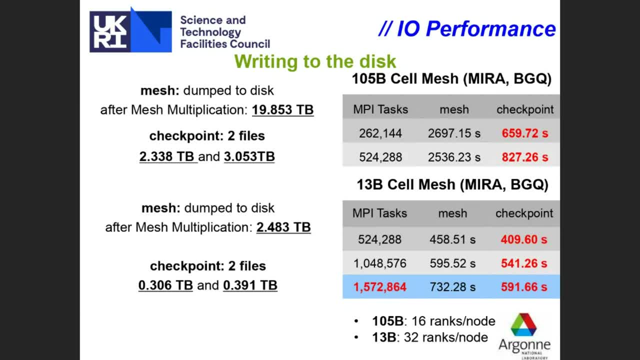 you can easily see that it's better to. you can easily see that it's better to keep everything on the fly, but in there, keep everything on the fly, but in there. keep everything on the fly, but in there. i mean that was just an exercise to. i mean that was just an exercise to. 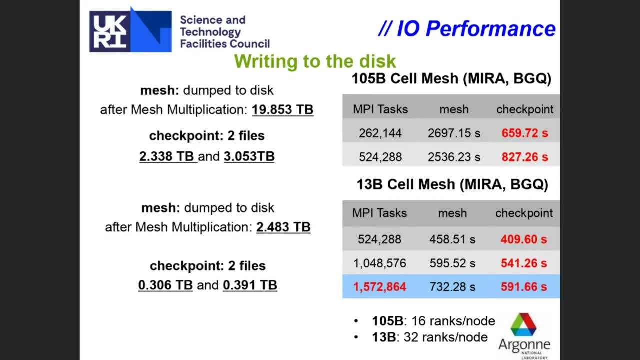 i mean that was just an exercise to to to to write the. the measure of the to to to to write the. the measure of the to to to to write the. the measure of the disk, disk disk, and from the checkpoint, i mean this is, and from the checkpoint, i mean this is. 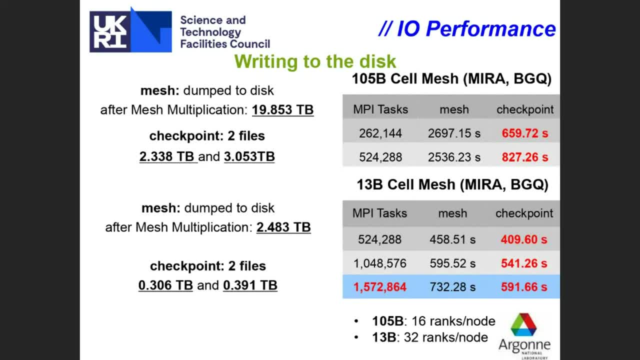 and from the checkpoint, i mean this is compulsory, so it takes compulsory, so it takes compulsory, so it takes 11, 11 to 11, 11 to 11, 11 to basically about 25 minutes, basically about 25 minutes, basically about 25 minutes in total. 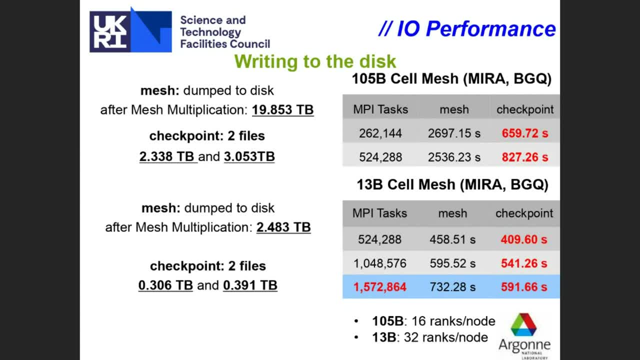 so i mean, and this has been run also on, so i mean, and this has been run also on, so i mean, and this has been run also on: tested on the. tested on the. tested on the on the full machine using uh. on the full machine using uh. 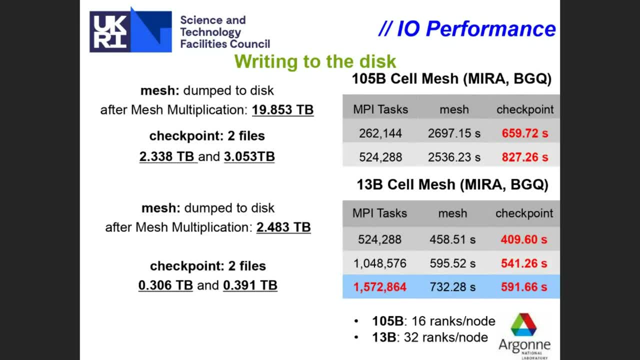 on the full machine using uh 32 ranks per node in the case of the 32 ranks per node, in the case of the 32 ranks per node, in the case of the 13 billion cells: 13 billion cells, 13 billion cells. but okay, this is difficult, but this is. 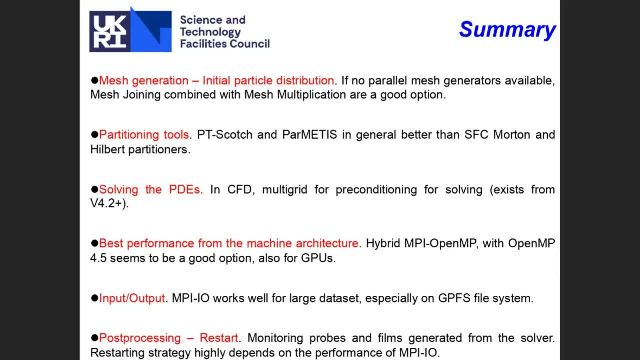 but okay, this is difficult, but this is. but okay, this is difficult, but this is doable, let's put it that way, doable, let's put it that way, doable, let's put it that way. so in a in summary, so in a in summary, so in a in summary, just want to say that for the mesh. 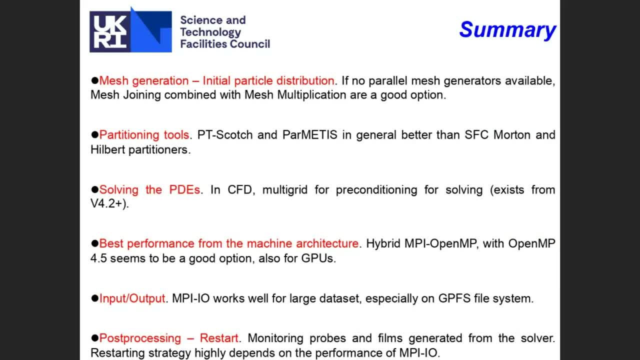 just want to say that for the mesh, just want to say that for the mesh. generation partitioning tool- solving pdes. generation partitioning tool: solving pdes. generation partitioning tool, solving pdes, and, and. and. we, we've got tools in the code that. we, we've got tools in the code that. 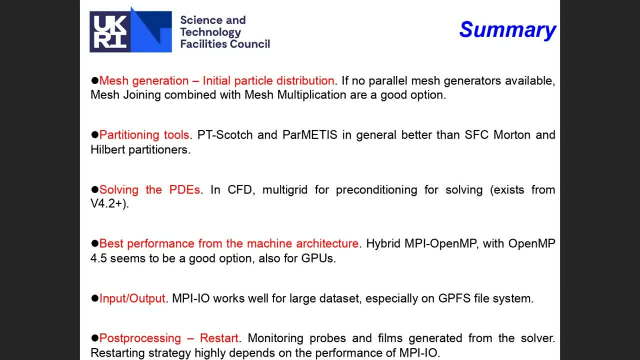 we. we've got tools in the code that can be used and have been used at, can be used and have been used at, can be used and have been used at, at, at, at, at a very large scale, at a very large scale, at a very large scale. so this 100 billion test case, i think 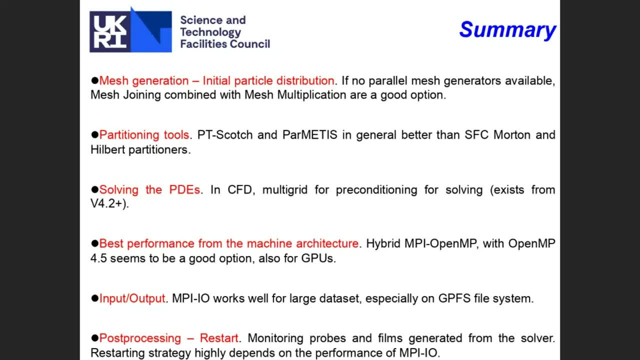 so this 100 billion test case, i think. so this 100 billion test case, i think in, in in. normal production runs are about normal production runs are about normal production runs are about a max between uh, a max between uh, a max between uh 100 million to half a billion. really. 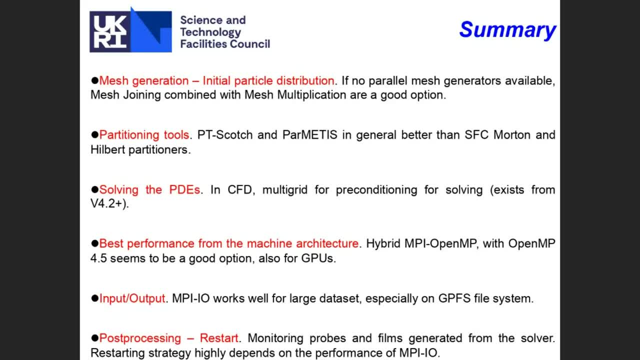 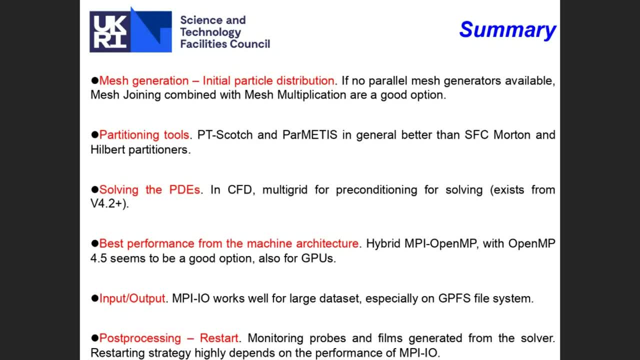 for the best performance uh. for the best performance uh. depending on the machine architecture, so depending on the machine architecture, so depending on the machine architecture. so this is depends, this is ongoing, this is depends. this is ongoing. this is depends, this is ongoing, obviously because new architectures are. 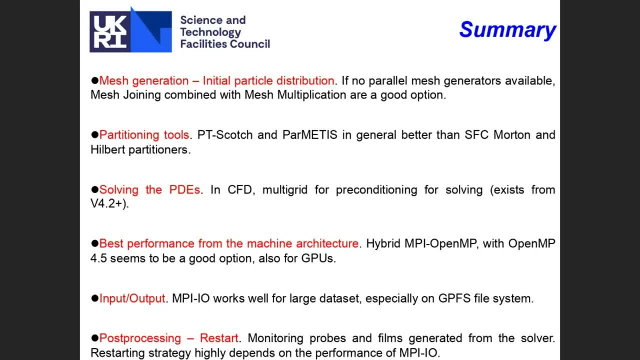 obviously because new architectures are. obviously because new architectures are always coming up, always coming up, always coming up. there's also an issue when you go to gpus. there's also an issue when you go to gpus. there's also an issue when you go to gpus is that each vendors get their own. 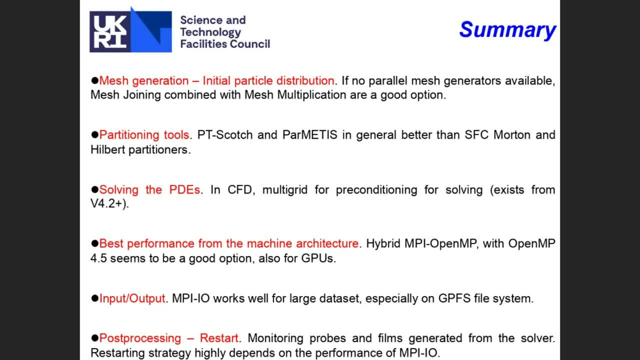 is that each vendors get their own? is that each vendors get their own own, own own modeling uh, modeling, uh, modeling uh. no all, no all, no all. programming uh tool for that. so programming uh tool for that. so programming uh tool for that. so. so amd's got a different one than nvidia. 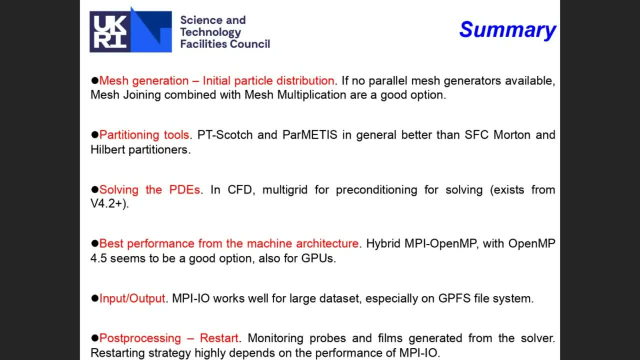 so amd's got a different one than nvidia, so amd's got a different one than nvidia. and intel as well. so so we need to adapt, and intel as well. so so we need to adapt, and intel as well. so so we need to adapt the code in a way that it gets. 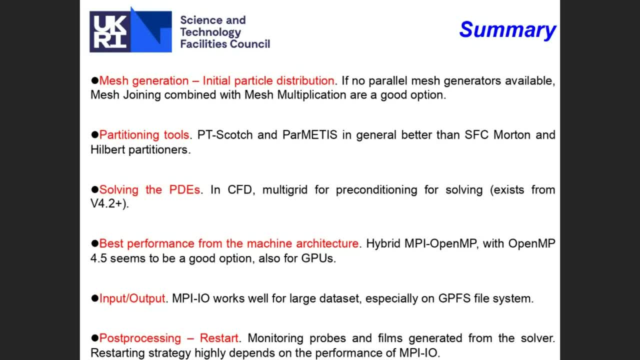 the code in a way that it gets the code, in a way that it gets portable, so you might lose some of the portable, so you might lose some of the portable, so you might lose some of the and all the and all the and all the gain, or you might lose a little bit of. 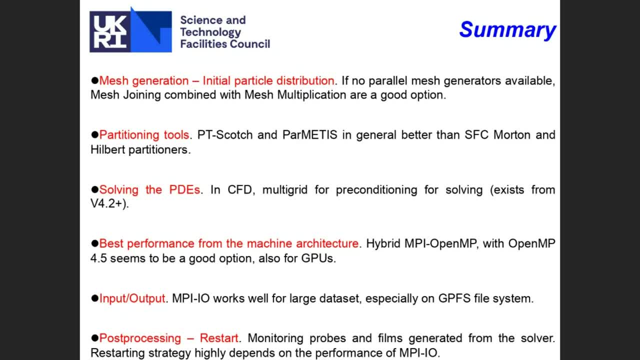 gain, or you might lose a little bit of gain, or you might lose a little bit of performance. performance, performance if you use a more general tool. but these if you use a more general tool. but these if you use a more general tool. but these are options which are actually very 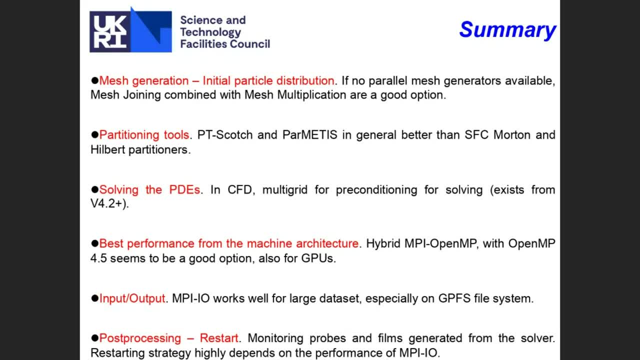 are options which are actually very, are options which are actually very difficult, to difficult, to difficult, to to predict and to account for, so at to predict and to account for, so at to predict and to account for so at at that time, at that time, at that time, uh, open mp 4.5 and maybe five. 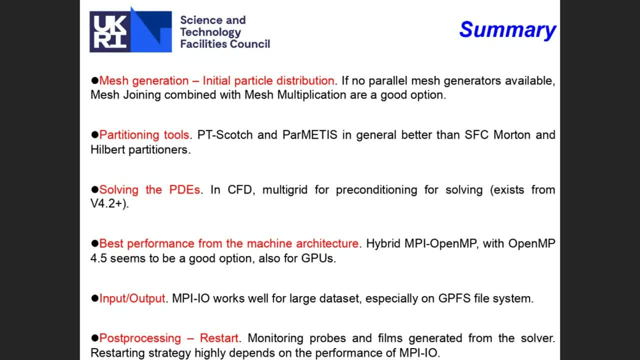 uh open mp 4.5 and maybe five. uh open mp 4.5 and maybe five. look like a good option for gpus, but look like a good option for gpus. but look like a good option for gpus. but open scc is another one. 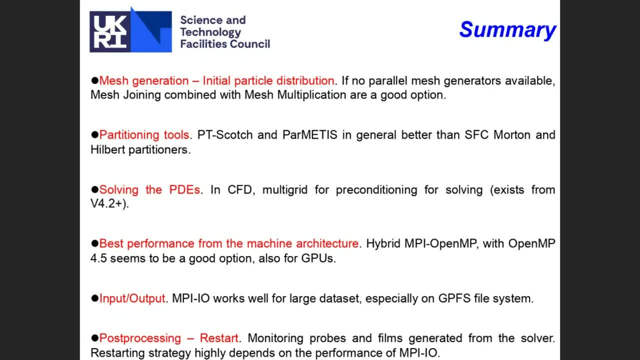 open scc is another one. open scc is another one. so we don't know yet in which direction. so we don't know yet in which direction. so we don't know yet in which direction it's going to go. it's going to go, it's going to go. and for the ios, so they work fine on. 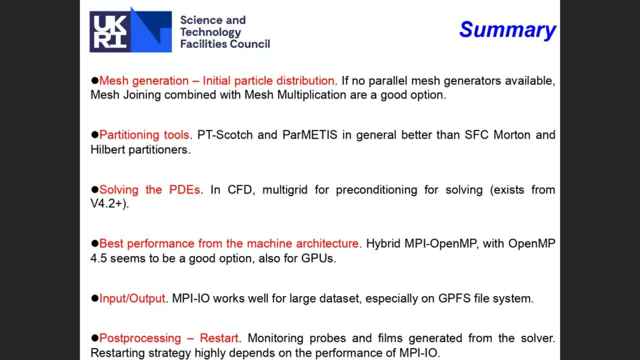 and for the ios, so they work fine on and for the ios, so they work fine on the gpfs system. so the gpfs system, so the gpfs system, so the old system luster which is used and the old system luster which is used, and. 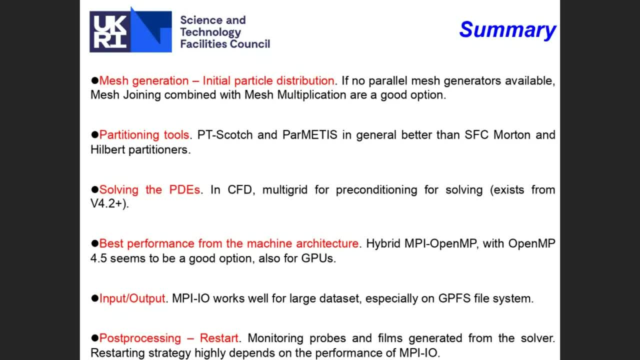 the old system, luster which is used, and an archer tool has been tested as well. an archer tool has been tested as well. an archer tool has been tested as well. and it, and it, and it. it works fine, but you need it, requires a. 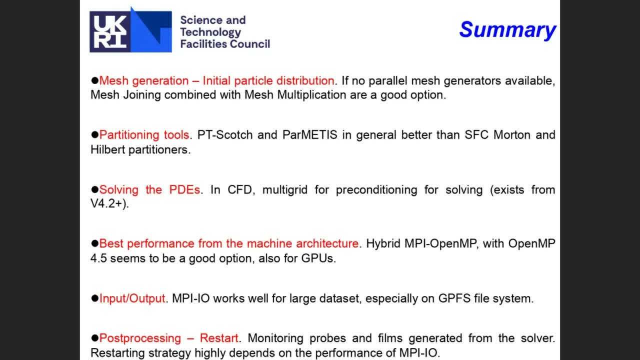 it works fine, but you need it requires a. it works fine, but you need it requires a little bit more, little bit more, little bit more. some settings, uh, some settings, uh, some settings, uh, working on on striping when you when. working on on striping when you when. 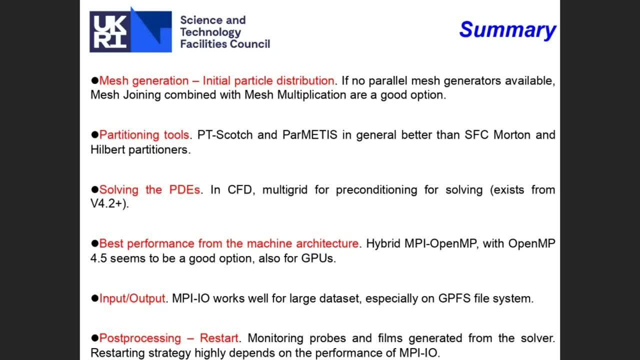 working on on striping, when you, when you, when you write on, read from the disk. you, when you, when you write on, read from the disk. you, when you, when you write on, read from the disk. and really the main bottlenecks, and really the main bottlenecks. 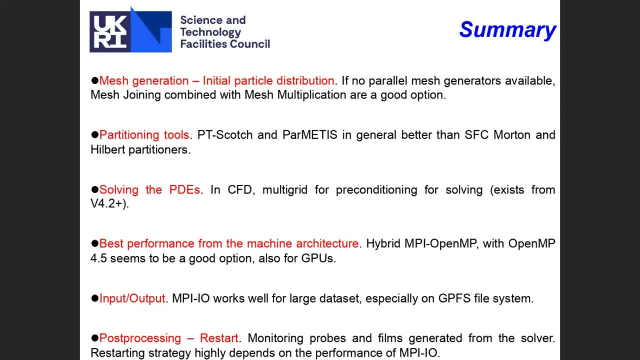 and really the main bottlenecks, is a is a restart on checkpointing for. is a is a restart on checkpointing for. is a is a restart on checkpointing for fire uh files, but this is not only for fire uh files, but this is not only for. 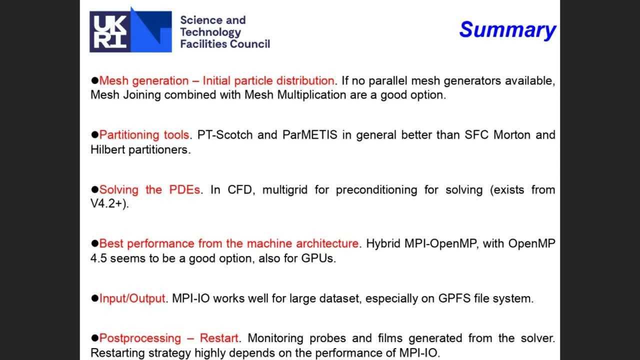 fire uh files. but this is not only for art for for concertion, it's for all the art for for concertion. it's for all the art for for concertion, it's for all the cfd codes, cfd codes, cfd codes. and finally, i want you just to show a. 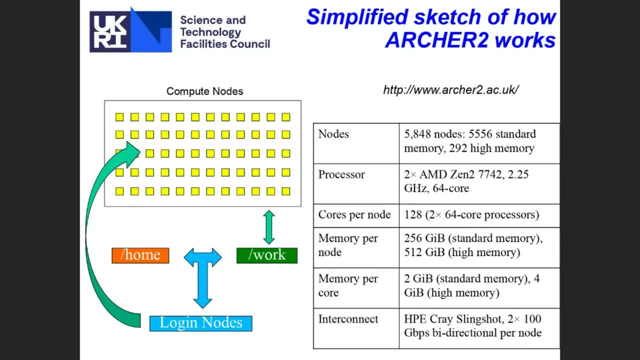 and finally, i want you just to show a and finally, i want you just to show a very simple, simplified sketch of how very simple, simplified sketch of how very simple, simplified sketch of how archer 2 works. so, on the the right hand, archer 2 works. so on the the right hand. 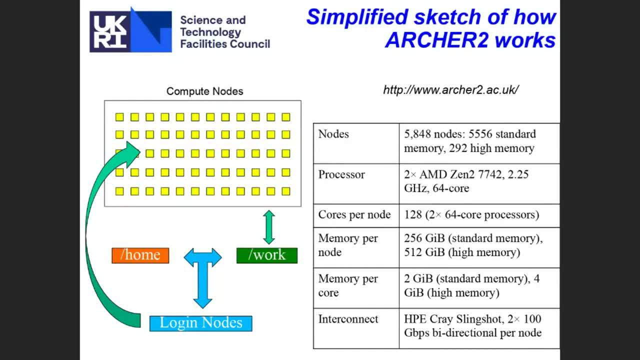 archer 2 works. so on the the right hand side you get the feature. so this is side. you get the feature, so this is side. you get the feature. so this is copied from the. copied from the. copied from the from the archer 2 websites. 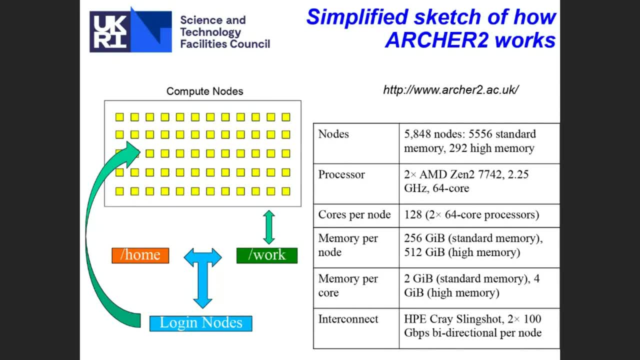 from the archer 2 websites. from the archer 2 websites, so so. so this corresponds to the code to the. this corresponds to the code to the. this corresponds to the code to the: to the machine when it's going to be a full. to the machine when it's going to be a full. 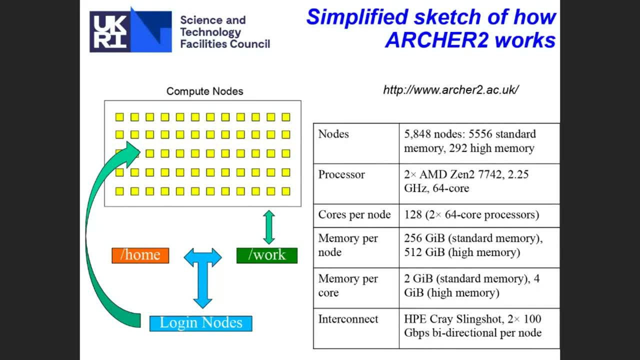 to the machine when it's going to be a full capacity, capacity, capacity, so so. so now, if i'm correct, you get about now, if i'm correct, you get about now, if i'm correct, you get about one-fifth or one-sixth of the machine. 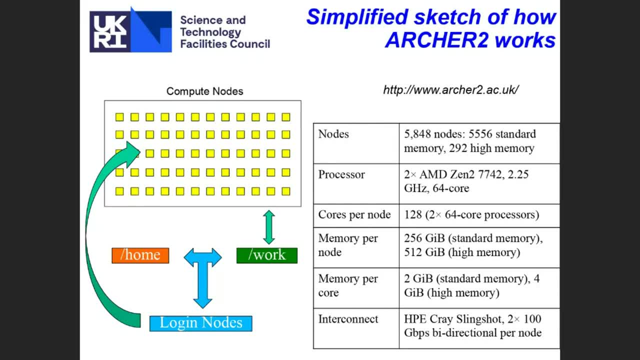 one-fifth or one-sixth of the machine, one-fifth or one-sixth of the machine. so you got four cabinets, so you got four cabinets. so you got four cabinets instead of the 23 which are going to be, instead of the 23 which are going to be. 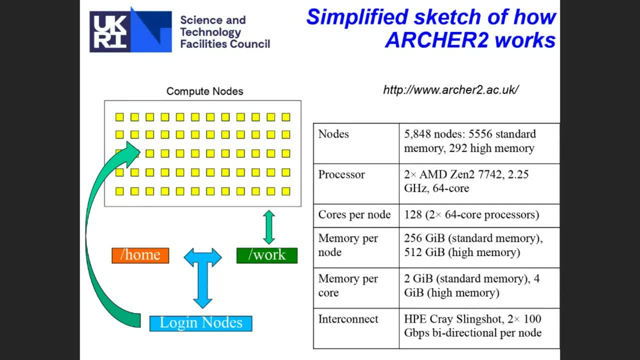 instead of the 23 which are going to be uh completely installed. so this makes a uh completely installed. so this makes a uh completely installed. so this makes a machine which is already very machine, which is already very machine, which is already very, very quick, but is going to be uh reaching i. 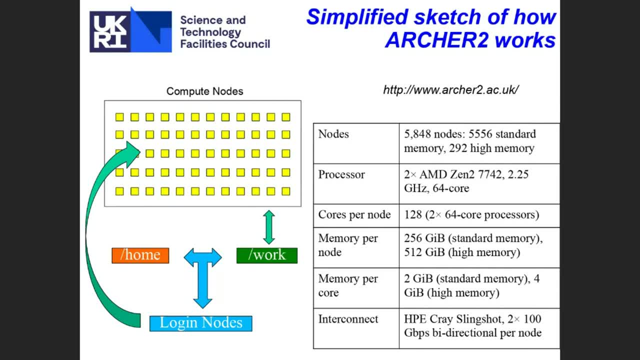 very quick, but is going to be uh reaching i very quick, but is going to be uh reaching, i think, 28 petaflops, maximum, which i mean, which is going to maximum, which i mean, which is going to maximum, which i mean, which is going to give them a very good rank in the top. 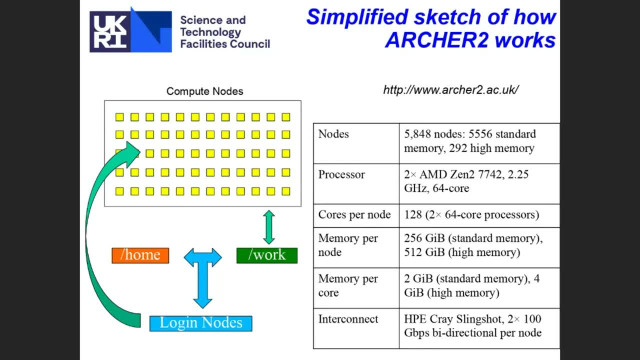 give them a very good rank in the top, give them a very good rank in the top 500 of the supercomputer, so of the supercomputer, so of the supercomputer. so basically, when you log on the machine, basically when you log on the machine, basically when you log on the machine, you go for the logging nodes and from 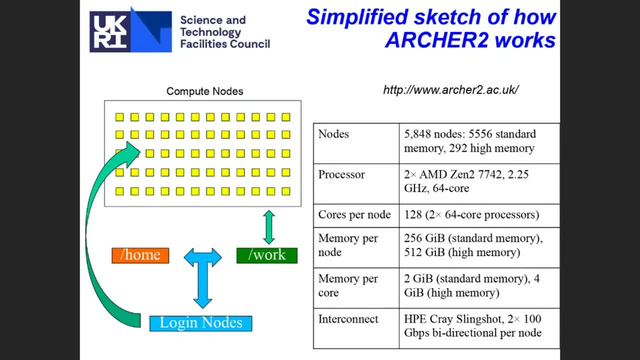 you go for the logging nodes and from you go for the logging nodes and from the logging nodes you've got access to the logging nodes. you've got access to the logging nodes. you've got access to the home to the work directory. the home to the work directory. 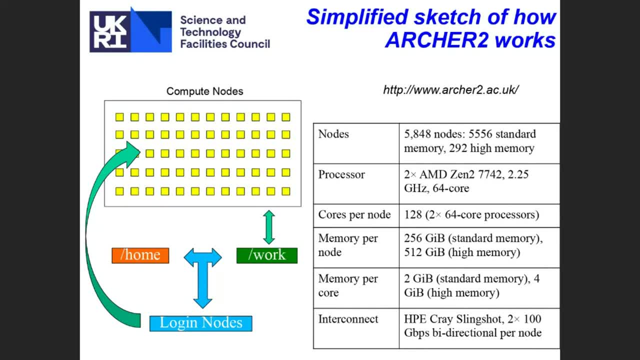 the home to the work directory. so what we have done is that we have. so what we have done is that we have. so what we have done is that we have created the what is called a soft link, created the what is called a soft link, created the what is called a soft link here under the home directory, so that 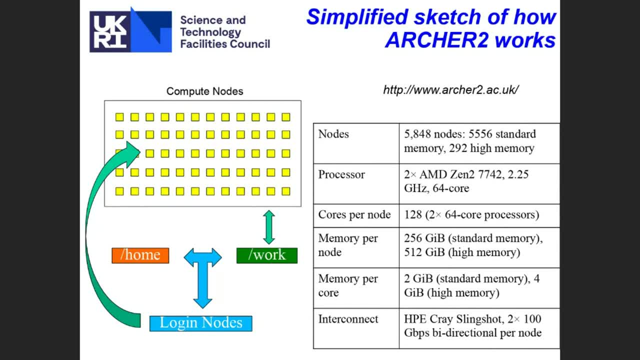 here under the home directory, so that here under the home directory, so that you can use the work directory. but you can use the work directory, but you can use the work directory, but be aware that, oh, you cannot submit some. be aware that, oh, you cannot submit some. 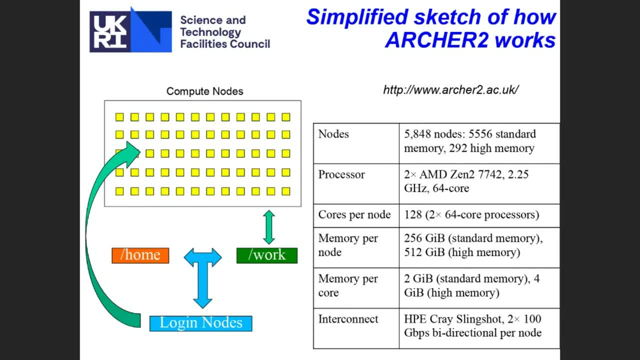 be aware that, oh, you cannot submit some simulation or jobs if you are not in the simulation or jobs, if you are not in the simulation or jobs, if you are not in the work directory, work directory, work directory. so be sure that you run all your. so be sure that you run all your. 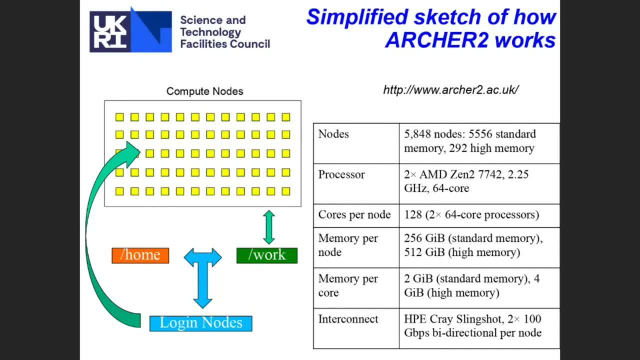 so be sure that you run all your simulation from the work directory. when simulation from the work directory, when simulation from the work directory, when you log on a nature 2, you log on a nature 2, you log on a nature 2 and from the work directories as uh. 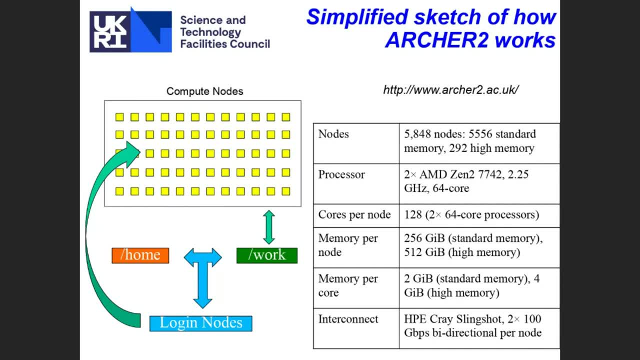 and from the work directories, as uh, and from the work directories as uh. i mean they, they have access to the. i mean they, they have access to the. i mean they, they have access to the compute node. so you don't see them. so compute node, so you don't see them. so 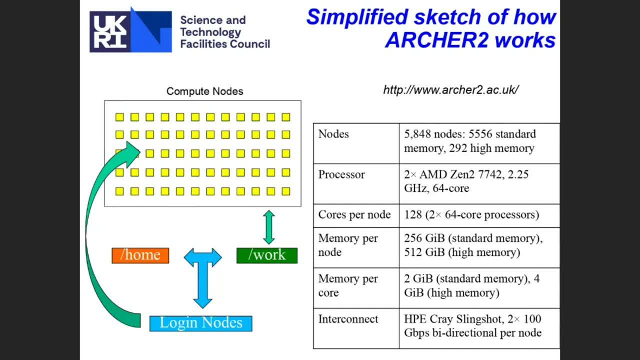 compute node, so you don't see them. so this is hidden, this is hidden. this is hidden through the, the, the queuing system, and through the, the, the queuing system, and through the, the, the queuing system, and and the submission system basically, and the submission system basically. 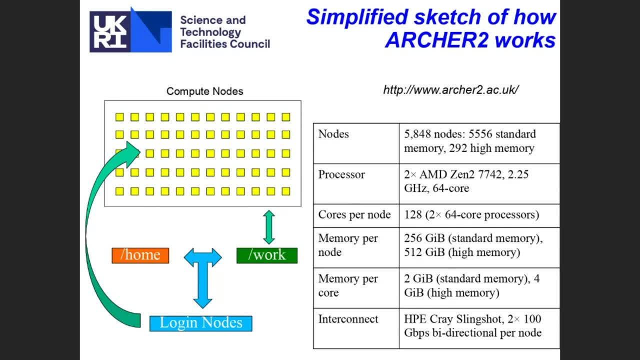 and the submission system, basically, but the simulation are running parallel, but the simulation are running parallel, but the simulation are running parallel on the compute node. so in your case it's on the compute node. so in your case it's on the compute node. so in your case it's going to be on one node. 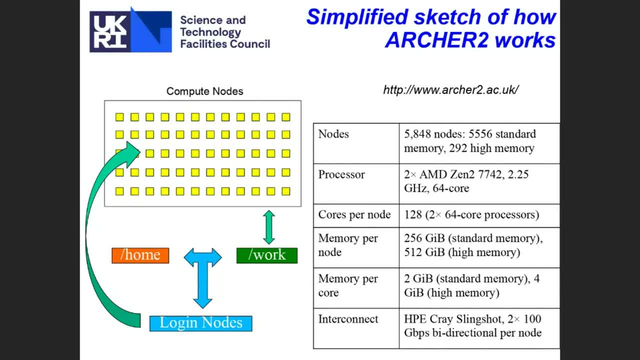 going to be on one node, going to be on one node and with which going to have 128 and with which going to have 128 and with which going to have 128, mpr tasks, mpr tasks, mpr tasks and, at the end of the simulation, you, you. 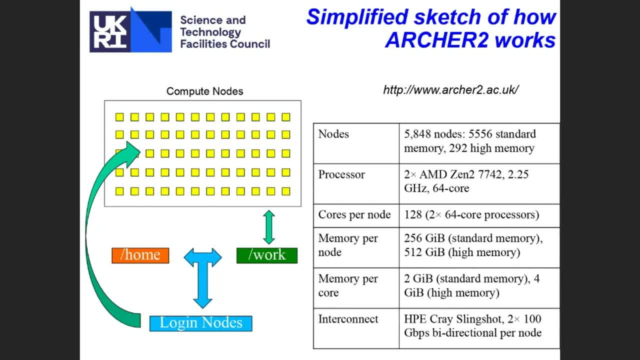 and at the end of the simulation, you, you, and at the end of the simulation, you, you, recover all your results, recover all your results, recover all your results, still under the work directory, still under the work directory, still under the work directory. so, so, so, just for me. so, if you have any questions, 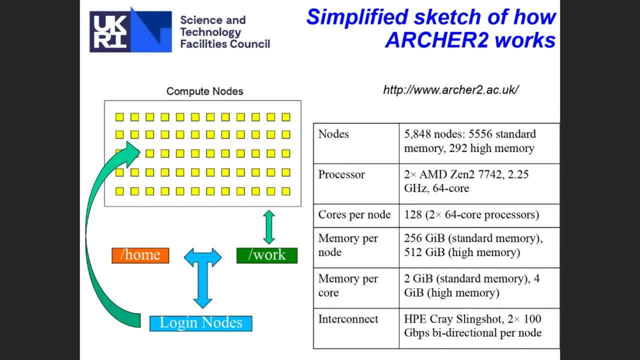 just for me. so if you have any questions, just for me. so if you have any questions, just don't hesitate, or just don't hesitate, or just don't hesitate, or write them in the chat and i can answer. write them in the chat and i can answer. 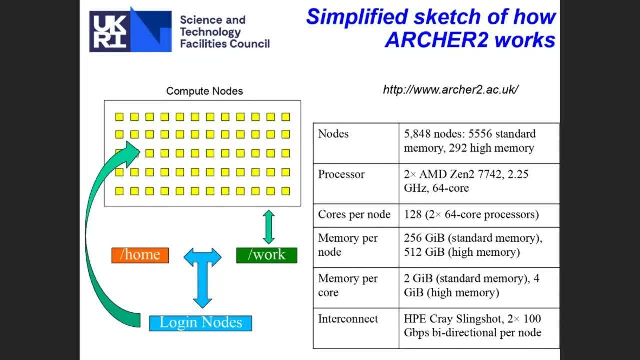 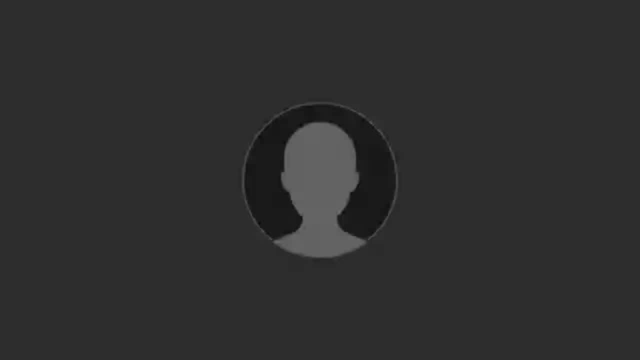 write them in the chat and i can answer what you are going for the next, what you are going for the next, what you are going for the next tutorial, i guess. thank you, feel free to speak and just ask the. feel free to speak and just ask the. 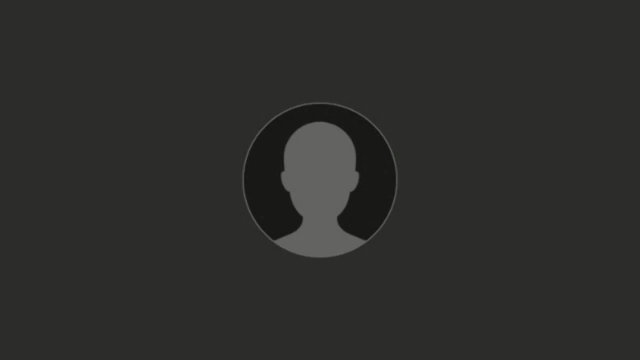 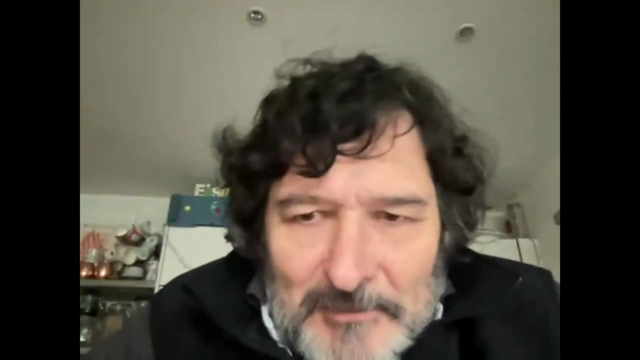 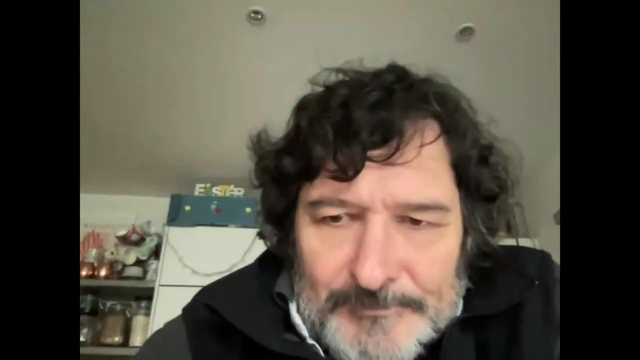 feel free to speak and just ask the. well, if you want, okay, so maybe the questions are going to okay. so maybe the questions are going to okay, so maybe the questions are going to come later. come later, come later during the tutorial. so during the tutorial, so during the tutorial. so let's move to the 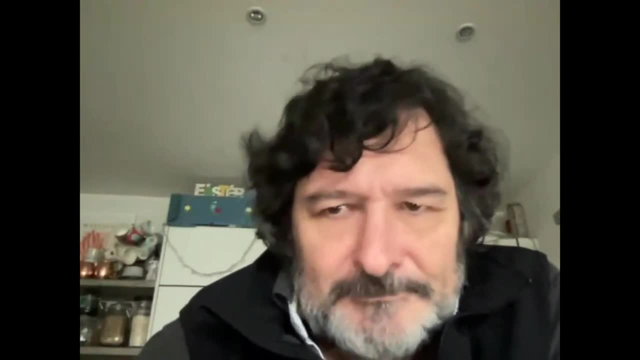 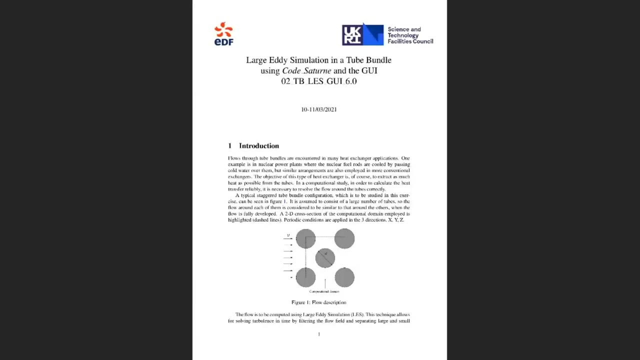 let's move to the, let's move to the next one, which is next one, which is next one, which is this one. so this, this is the- still the flow in a tube bundle, but now still the flow in a tube bundle, but now still the flow in a tube bundle, but now we are going to use 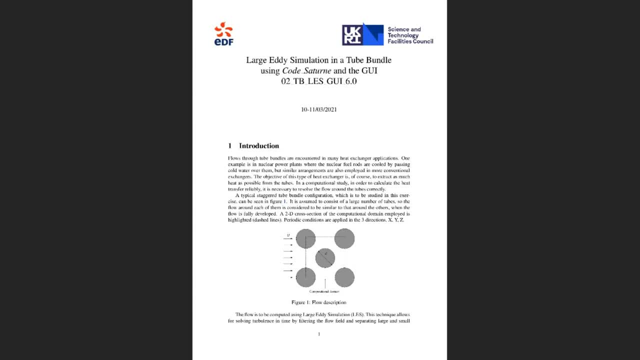 we are going to use, we are going to use advanced turbulence modeling for it. so so, so this technique is called larger, this technique is called larger. this technique is called larger: dissemination, dissemination, dissemination. so the mesh is also going to be much, so the mesh is also going to be much. 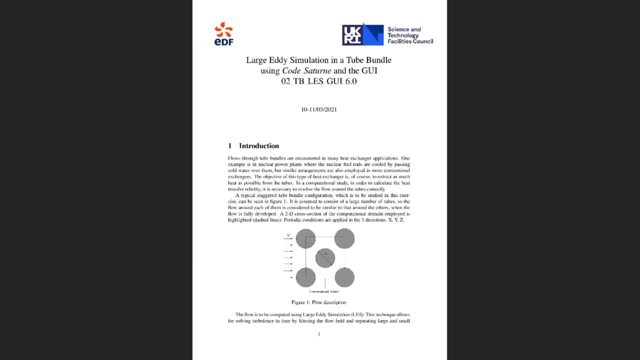 so the mesh is also going to be much bigger. it's going to have a 3.5 million bigger. it's going to have a 3.5 million bigger. it's going to have a 3.5 million. uh, uh, uh. cells is going to be fully 3d. 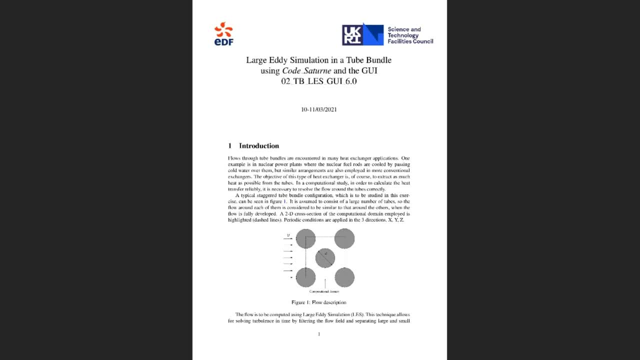 cells is going to be fully 3d, cells is going to be fully 3d, and the objective of this tutorial is, and the objective of this tutorial is, and the objective of this tutorial is for you to, for you to, for you to, to set up the whole case. 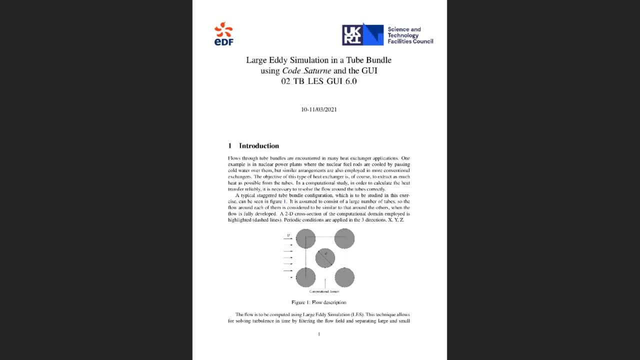 to set up the whole case. to set up the whole case on the, on the, on the local or virtual machine, local or virtual machine, local or virtual machine. so that's explained in the tutorial, so that's explained in the tutorial, so that's explained in the tutorial. and then 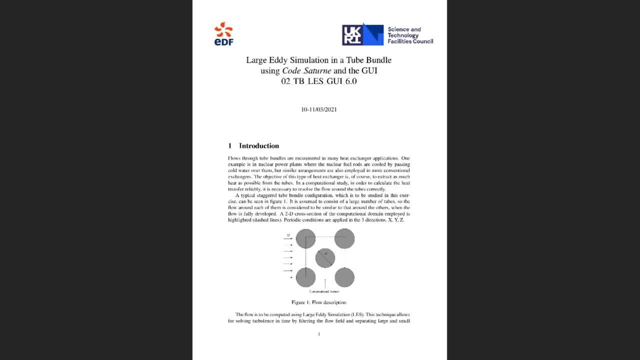 and then, and then, when you're ready to copy file across, when you're ready to copy file across, when you're ready to copy file across on archer, on archer, on archer, and then, then, and then, then, and then, then, use a submission script to submit a. 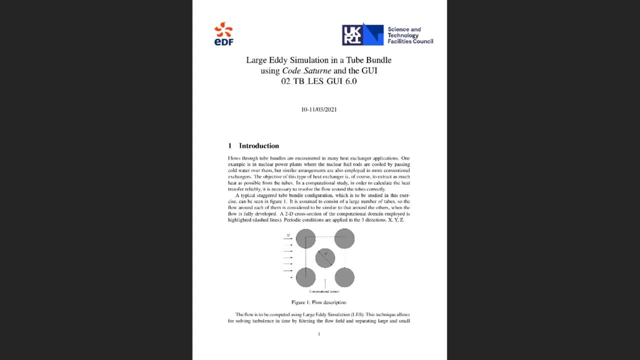 use a submission script to submit a. use a submission script to submit a job. so yeah, a mix of archer and archer job. so yeah, a mix of archer and archer job. so yeah, a mix of archer and archer too, but it should be actually all the. 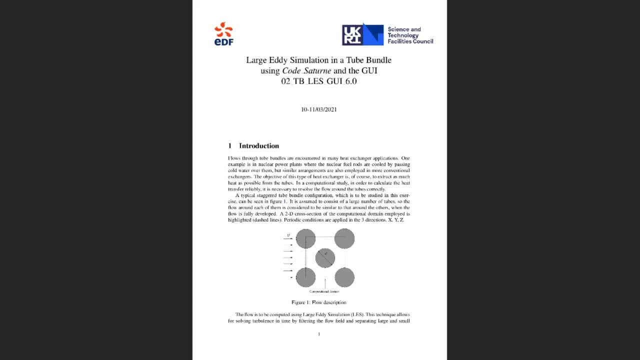 too, but it should be actually all the too, but it should be actually all the time, time, time, and so so to submit the job on archer, and so so to submit the job on archer, and so so to submit the job on archer, too, too. 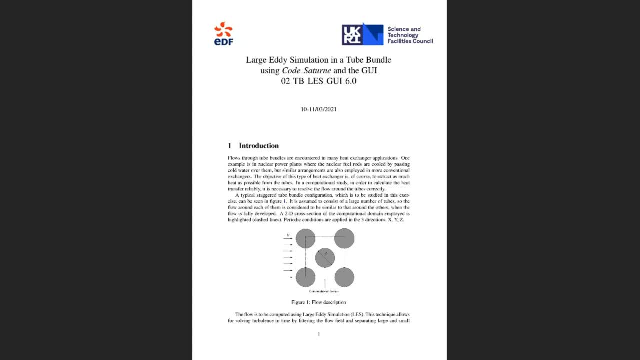 too, and and then the simulation should run, and, and then the simulation should run, and, and then the simulation should run for about 10 to 11 hours, for about 10 to 11 hours, for about 10 to 11 hours overnight, and tomorrow you're. 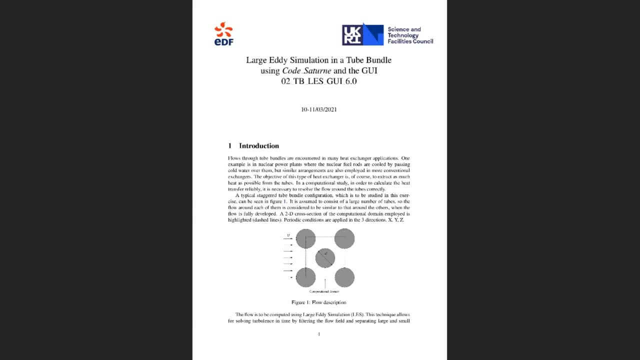 overnight and tomorrow you're overnight and tomorrow you're you're going to uh, you're going to uh, you're going to uh, to post process these results, so to post process these results, so to post process these results. so i think it's time for you to 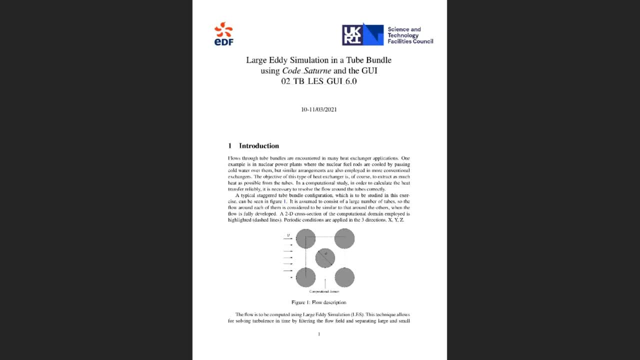 i think it's time for you to. i think it's time for you to to have a look at this one. okay, it seems like okay, it seems like okay. it seems like: um, let's, let's, let's. only two people that haven't been able to get the SSH key. For the rest, there's a step. 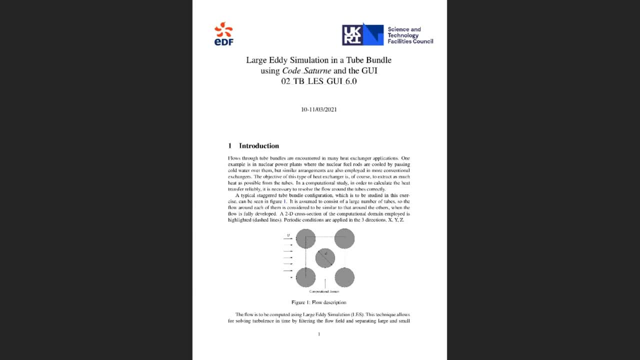 that you need to do after you generate that key and you log in first to Archer. So I'm gonna show you what you need to do. You can do that now, or you can do that whenever you are in the tutorial logging into Archer. I'm gonna share. 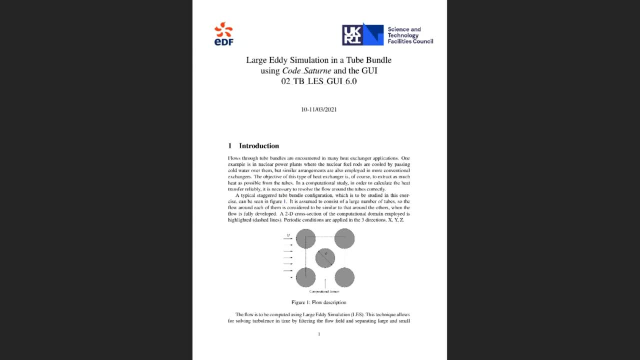 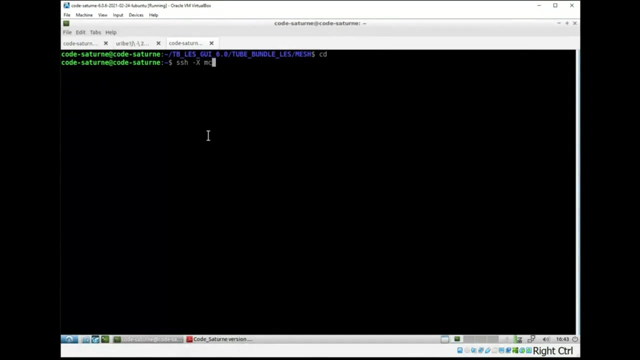 my screen so you can see what you need to do. So when you're in a terminal- whatever it is the terminal you are working on, whether it's the virtual machine or your own local machine- once you have uploaded the SSH key, you need to log in with username. that was. 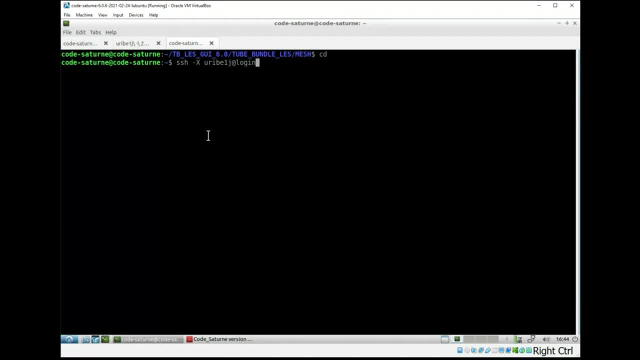 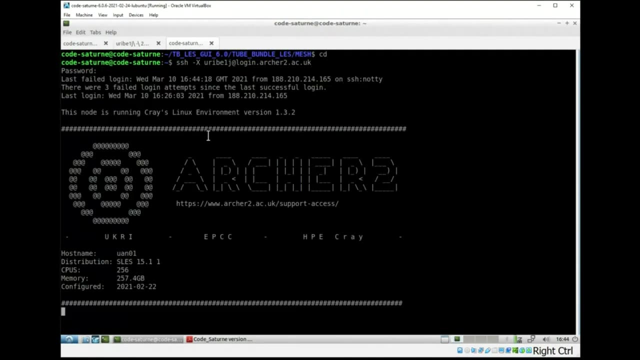 the one that you set up when you create the save account, and the name of the machine, which is Archer2, and you should be able to see the SSH key. But if anyone has a problem doing that, please let us know as soon as possible. 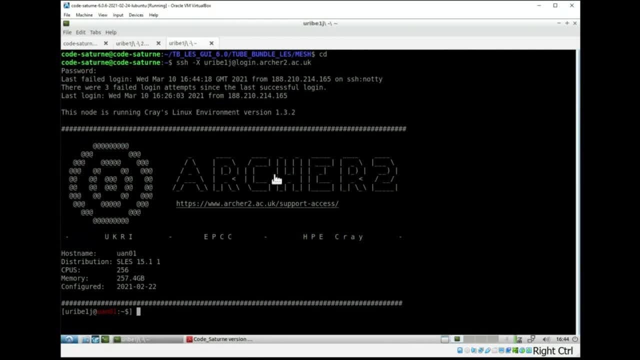 because there might be an issue with your authentication. So, before you can do anything, you're gonna need to copy a file that will set up your account the first time. This only needs to be done one time, okay. So what you need to do is copy from work and our group for this tutorial, which is TA019.. 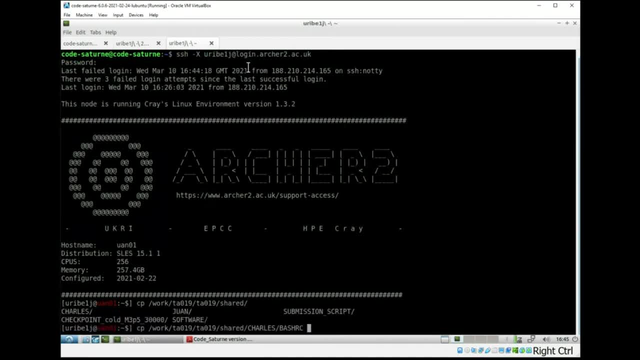 And then you're gonna find here a file called bash-rc. okay, This is a shell file that will set up your environment so that you can run Saturn correctly in Archer The first time that you log in. you just copy that into your home directory. 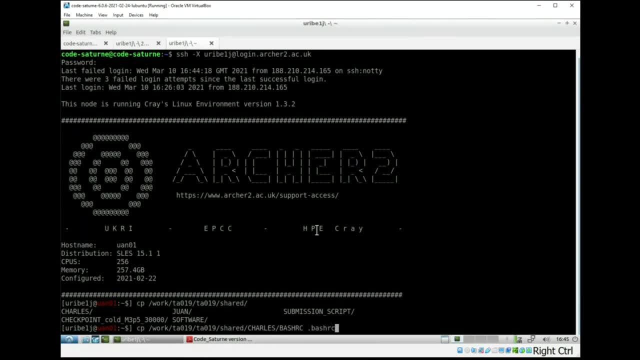 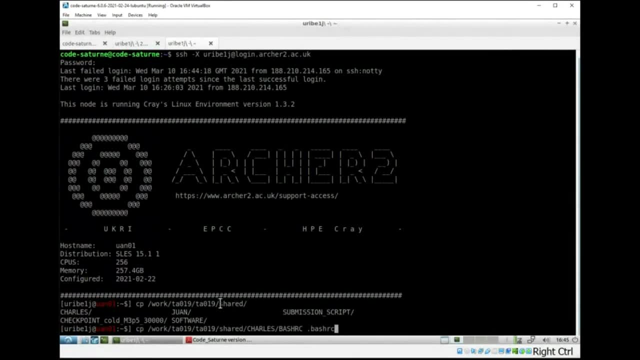 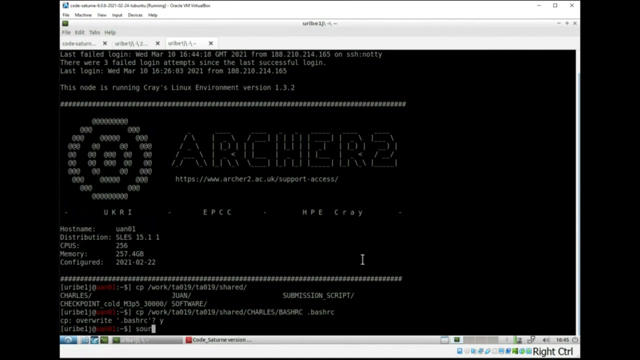 and rename it as bash-rc. okay, So this instruction will copy the file that we have for you. You will also have access to this shell directory, because you're part of the same group in your home directory. Okay, Um, once you've done that. 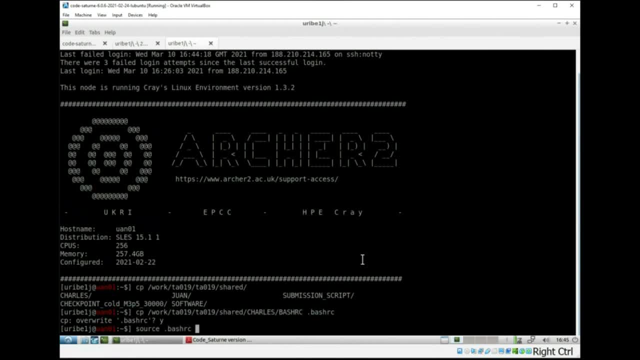 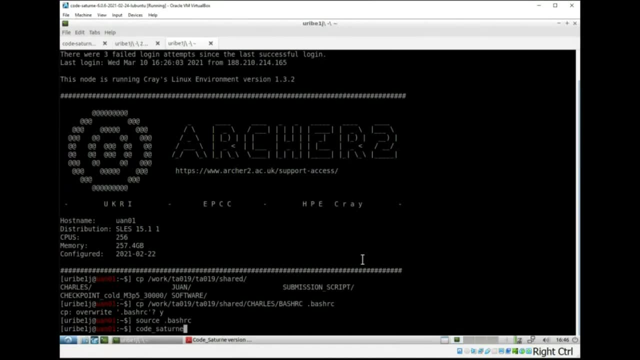 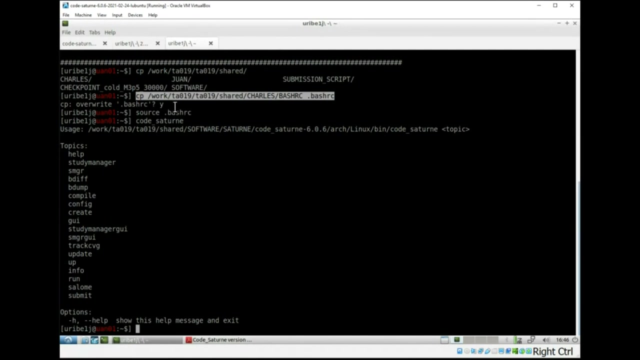 you can just source the same file And after that you should have the command code Saturn available for you. okay, So this only needs to be done the first time that you log in. So I'm gonna leave those two commands that one. 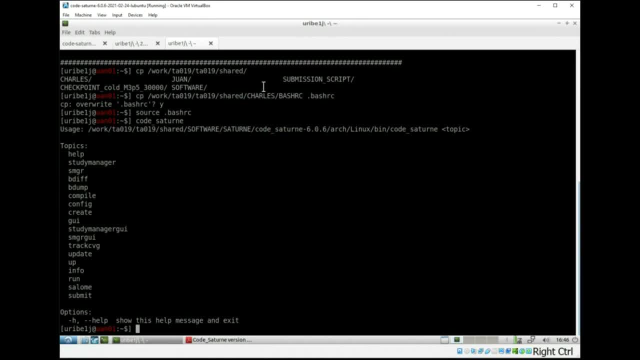 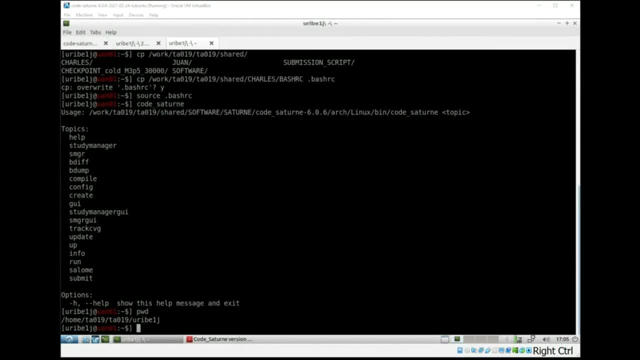 and that one there, And if you have any problems, let me know. Okay, just to explain a little bit of what's going on, because it's a bit of confusion: The bash-rc file that I gave you that you copy. 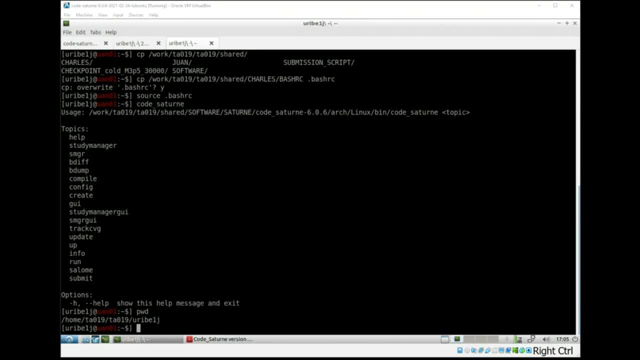 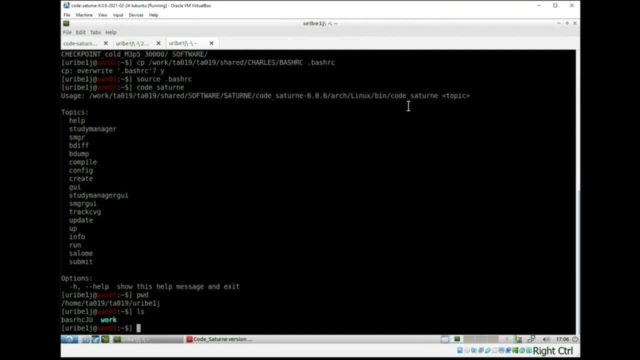 creates a link in your home directory to your work directory so that you don't have to put the whole path every time that you want to copy things from your local machine to the remote machine. So once you source the file, you should have. 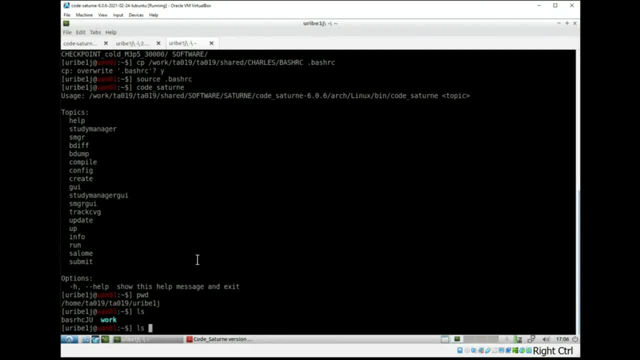 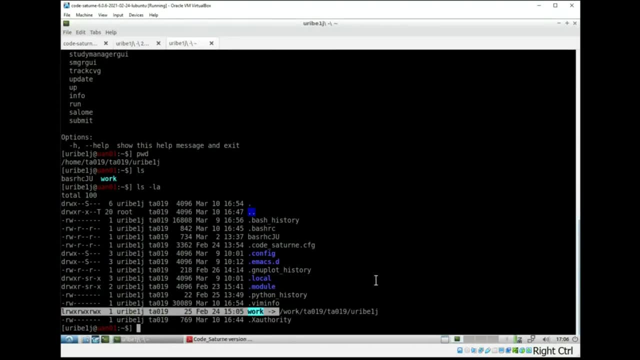 this link here in your home, which is, if you look at this, which is the, And for now, it's books, if you, if you look at that, it's pointing to in my. this is my username, obviously, but for each one of you will be your different username, so this path is equivalent to. 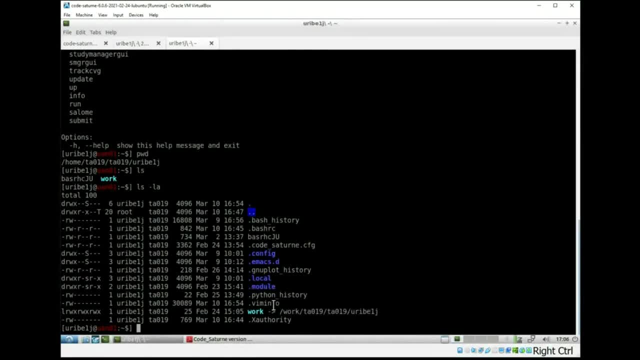 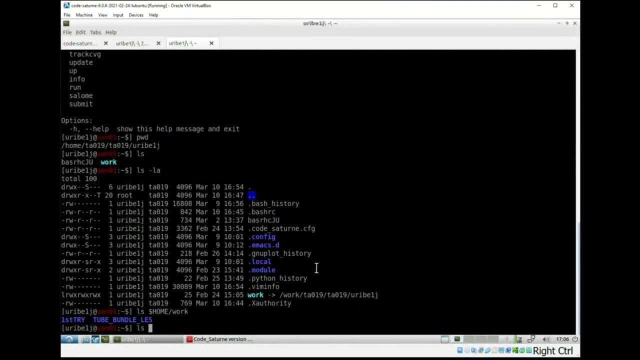 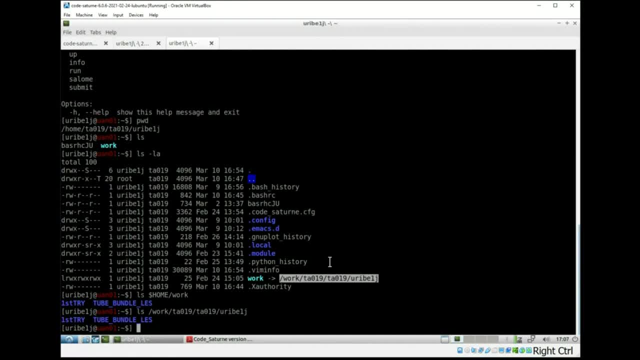 you'll see later, when you have to copy the mesh and you have to copy your subroutines and you have to copy your xml file. you don't have to put a very long path, it's just short, so i'm going to show you how to do that. 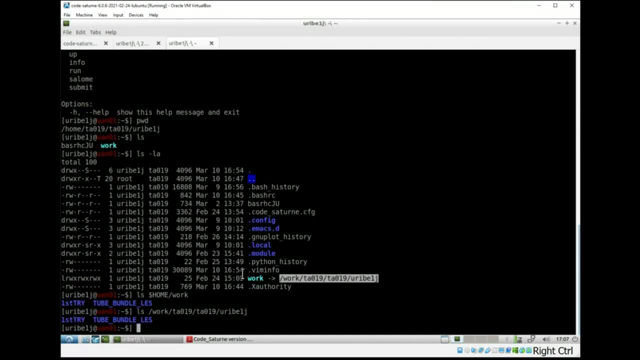 okay, um, yeah, it's just that my the work link it points to the project c01 instead of ta019 and that's why it didn't let me access it. i don't know if it was created before or something, but that's the problem. uh, okay, let me check. 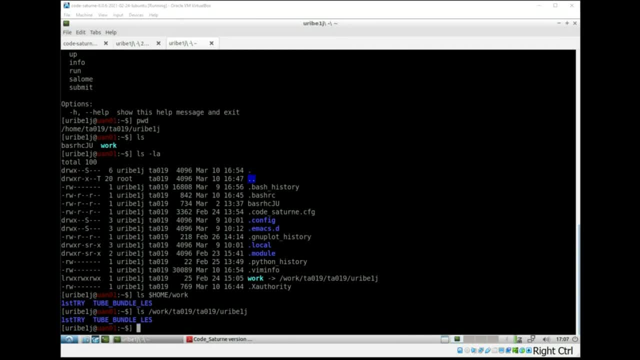 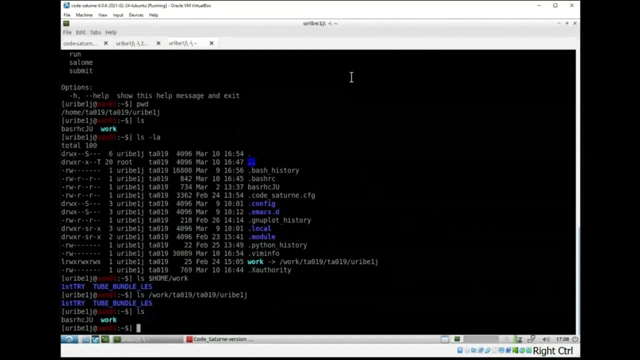 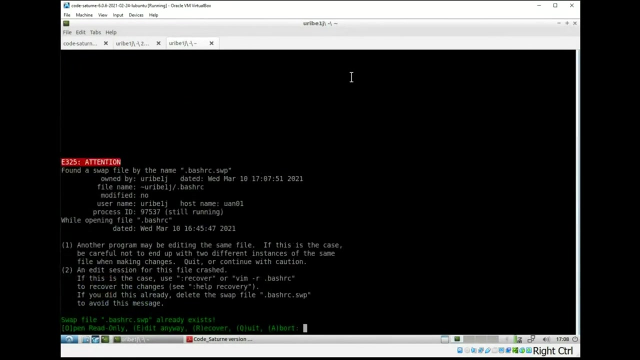 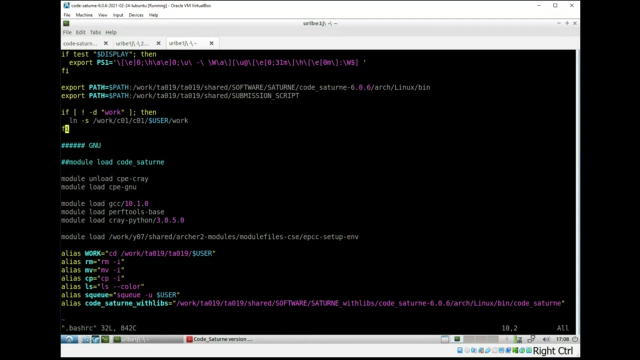 i'll change this in the brush. i'll see, um. i think my patch. i've seen this. maybe not. ah, yes, sorry, um, i need to do it again. all right, okay, i know u don't know how to do this. yeah, you're right, this should be okay. can you just log out or log in again? 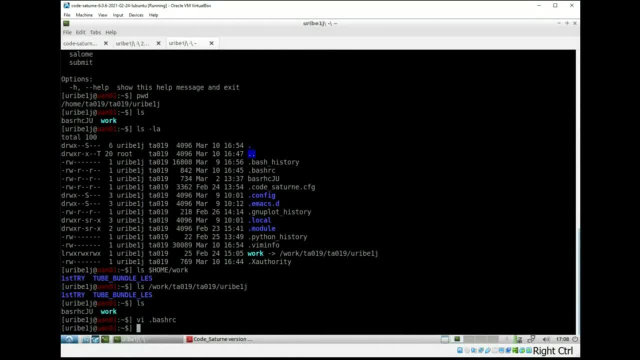 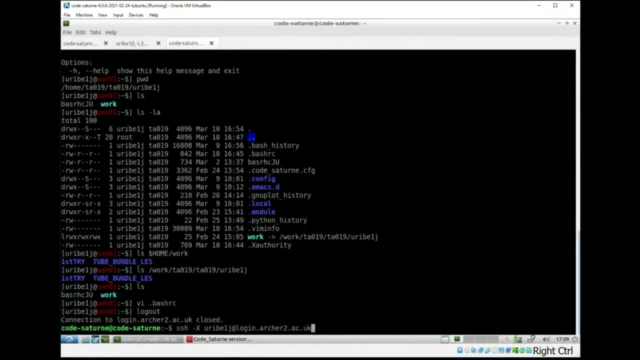 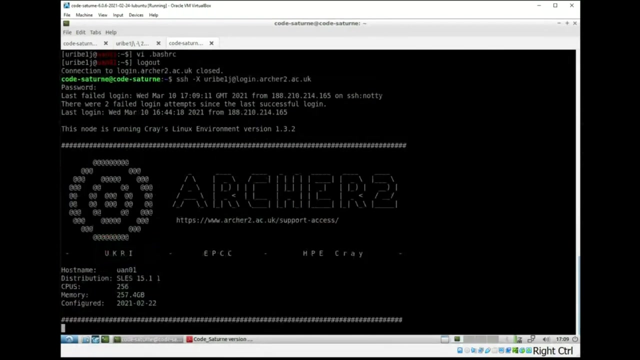 i just changed it. uh, one i just changed. So can you log out on the green again? to Archer: Yeah, I'll do that. You need to copy it again and source it again. Okay, Yes, I don't know, You might need to remove the existing link actually. 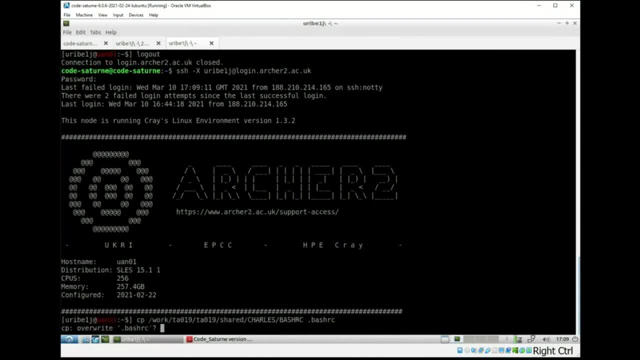 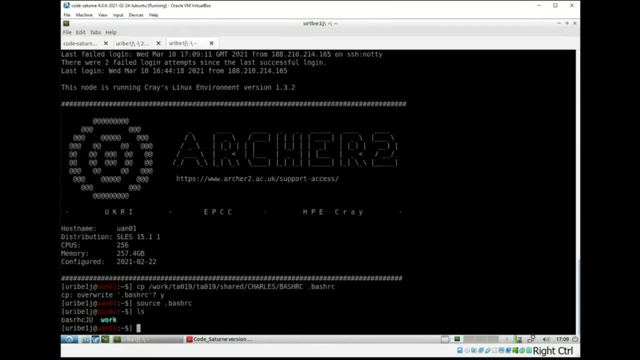 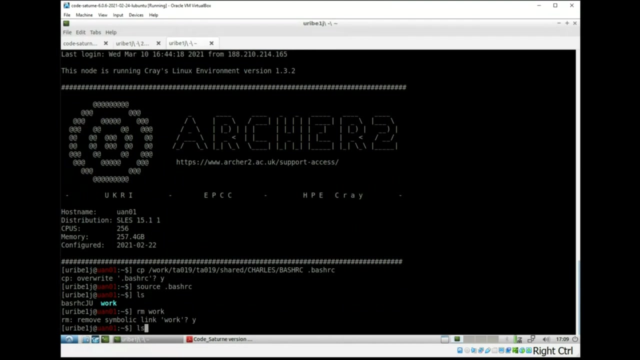 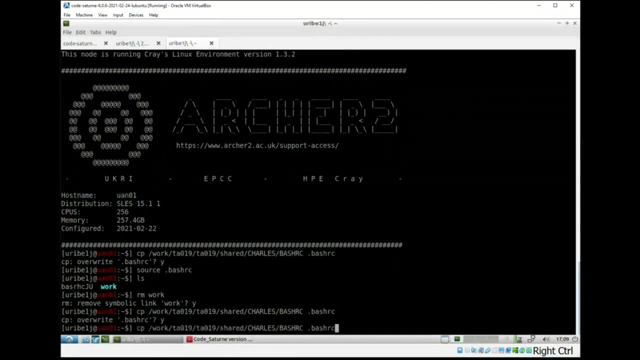 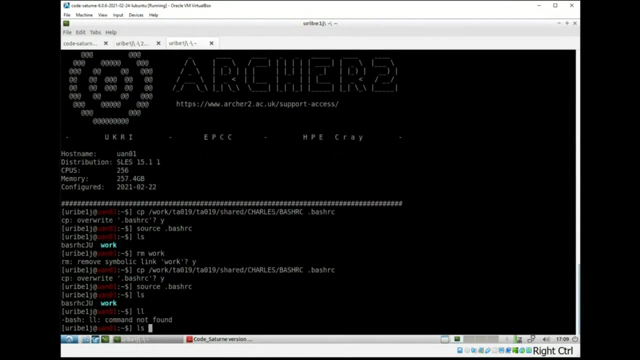 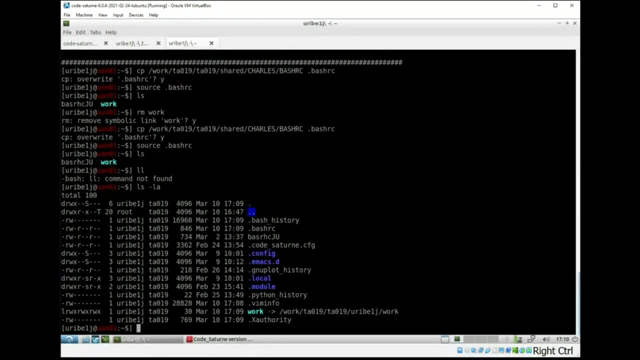 Because if I do this And if you had, yeah, It's better if you do that before you do that. No, that's wrong, That's wrong. No, no, no, Do it again, Do it again, Just delete. 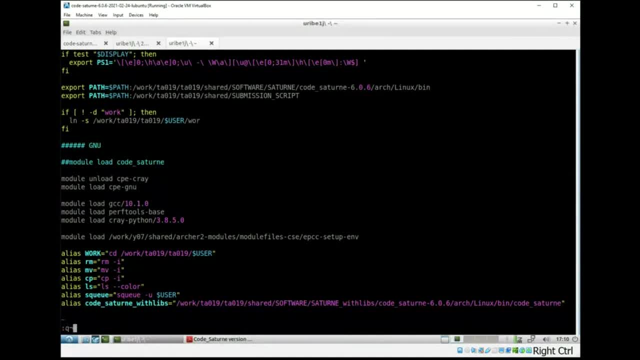 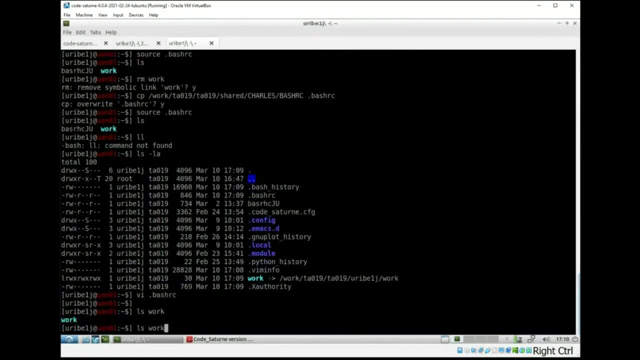 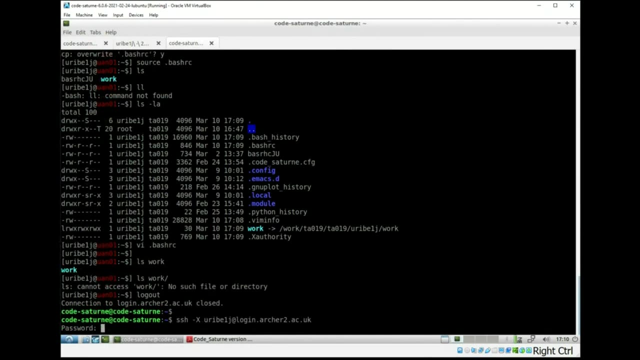 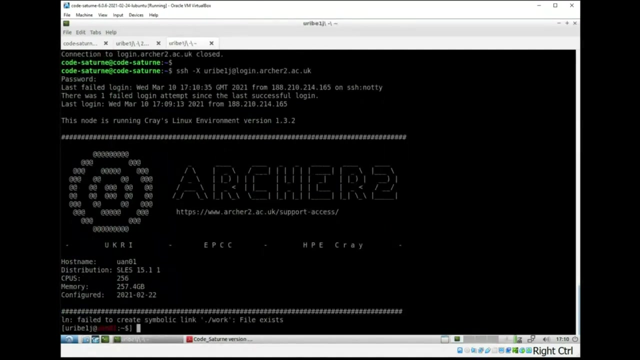 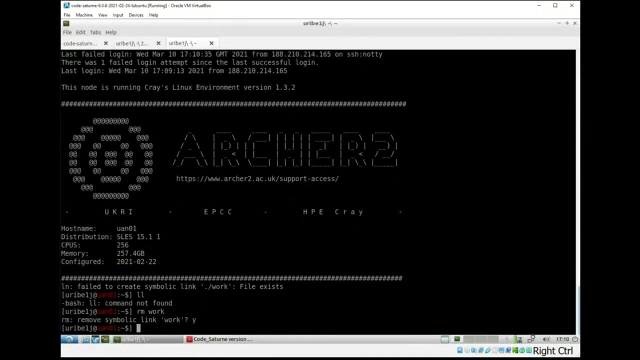 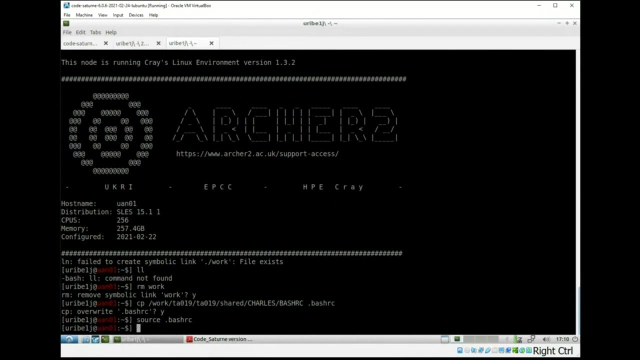 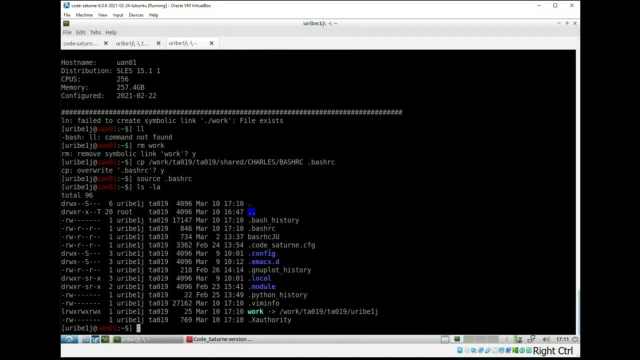 It happens that for the course I had to prepare for another account- this C01 account- for other people, So when I copied the BashRC I mean I missed that bit. Okay, just to clarify If you're in your home directory when you log in to Arche. if you type ls-la like this: 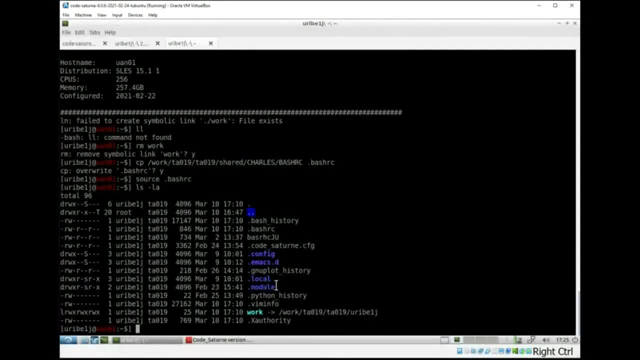 you should see the link for your work directory and it should have TA019.. If it has 0, it should be 0.. So C01 or C03, that's wrong. So if it doesn't have TA019, you should remove that link. then copy the BashRC file again. 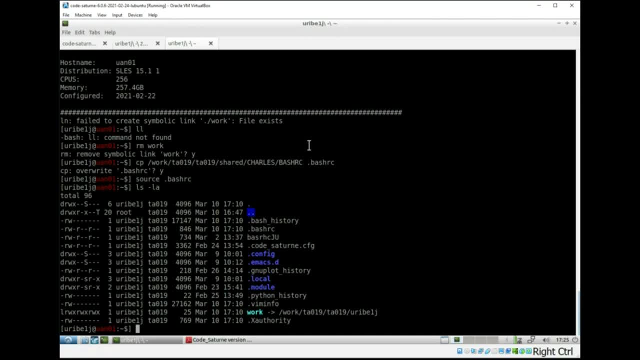 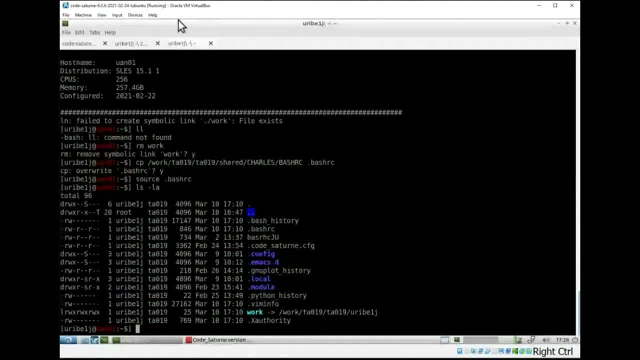 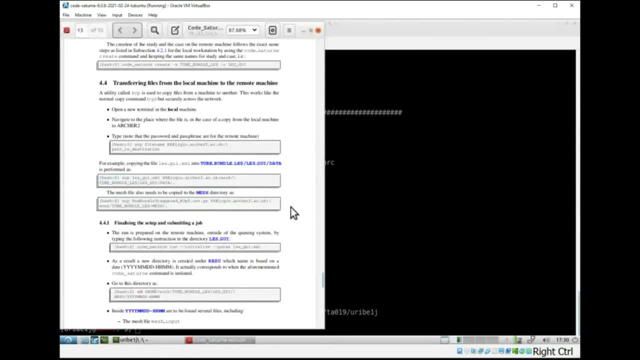 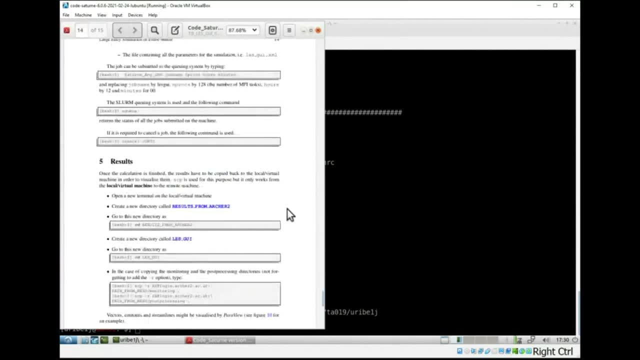 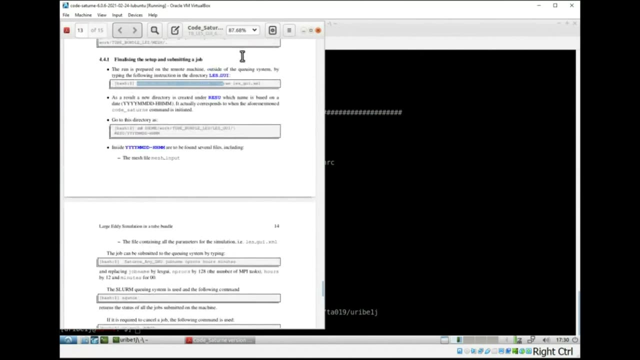 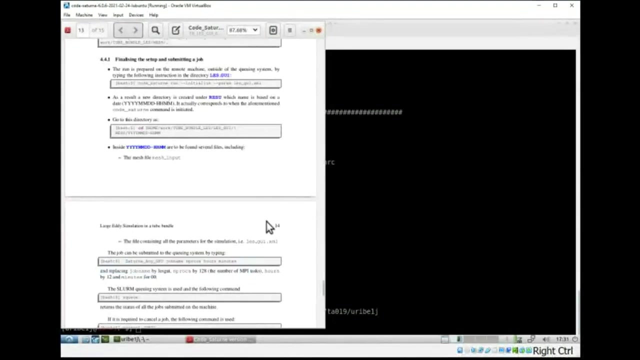 So when you do the initialize, it's not really running yet. It's after you submit the case that it starts to run. So when you do this bit it goes really fast, but when you do this bit it just stays there until the end. 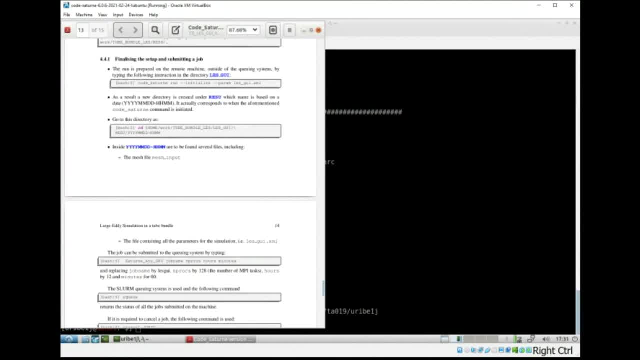 And this is related to what I was saying before- that the encode-shuttle and everything is separated. So what you do when you initialize is create the directory where it's going to run. it's reading the mesh file, it's creating that intermediate file between the preprocessor. 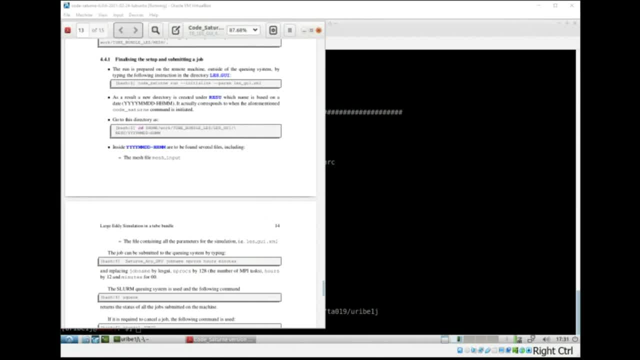 and the kernel and it's letting everything there ready for running when you submit it. So it's because here in Archer you don't have a graphical interface that would do that for you. You have to do it in these two stages. And to add on what Rohan said, this first part, the run initialize, is run serial. 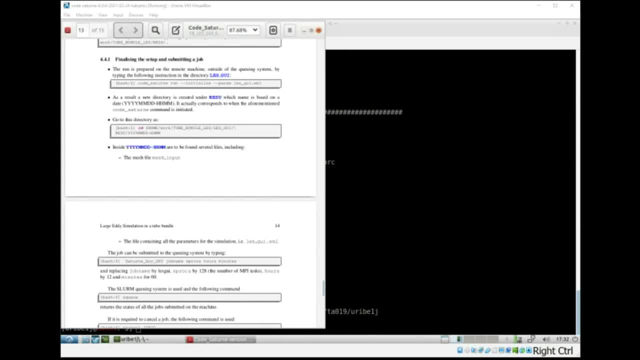 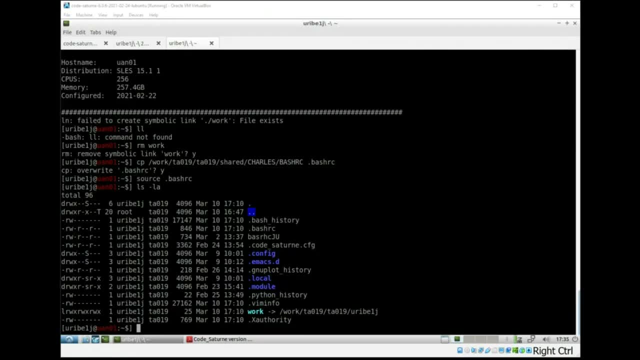 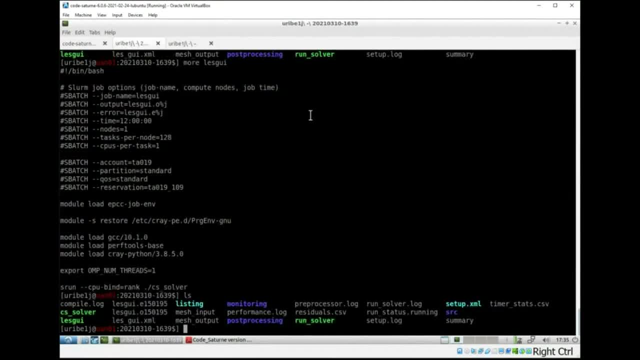 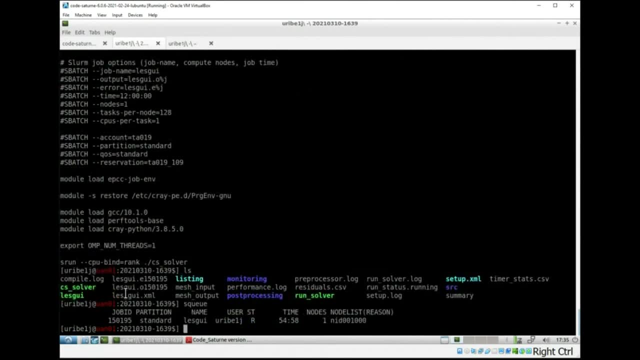 So the job is working. If you're going to your working directory and you type sq, you should see something like this, And the key thing here is the R, which means running. Okay, It tells you which node is running, for how long, etcetera. 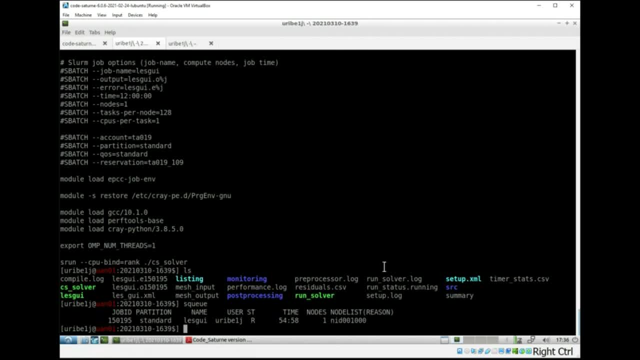 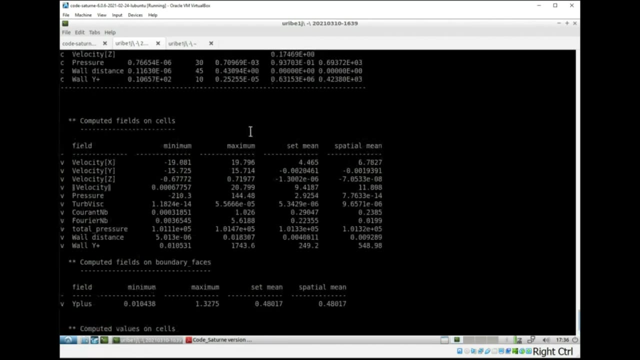 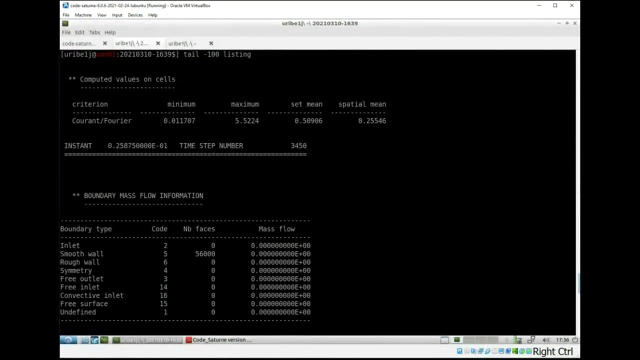 But at the same time, while this is running, it's also writing. it's also writing this cronsolverlog file, or listing file, which is the same thing you can- you can always check what's being written there. so this is the kind of information that you will get, and 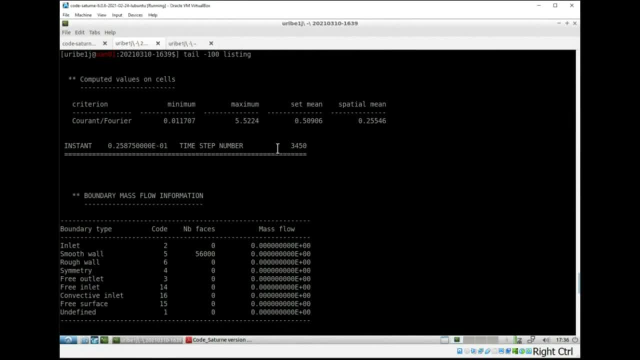 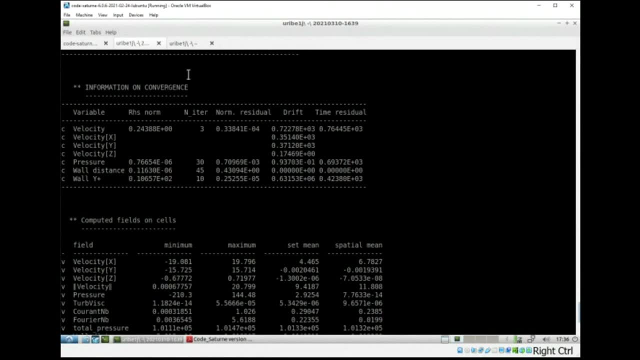 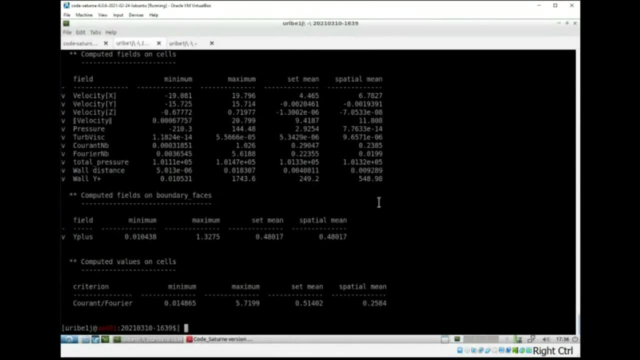 and at each time step. well, we're writing here between five time steps, but you have there, for each variable, the number of iterations, the residuals, the minimum, maximum, etc. all right, so for all those that have the job running, and now the only thing left is to wait. 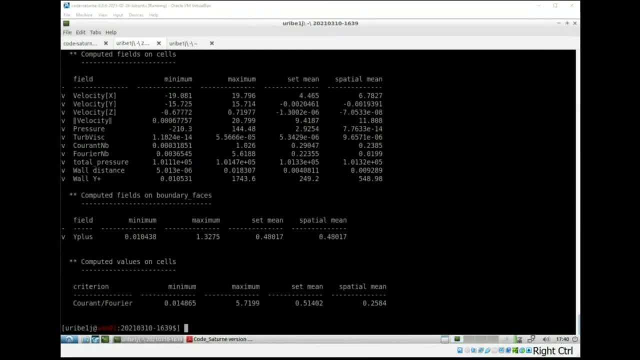 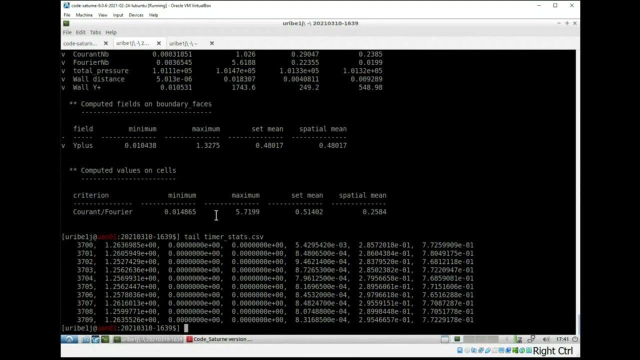 so it should run for about 10 hours and the idea is that we come back tomorrow and and we the results. i would encourage you to wait until you start seeing that the job is running. so if you type, for example, this timer, statistics is collecting statistics for each iteration. so the first column, this is the 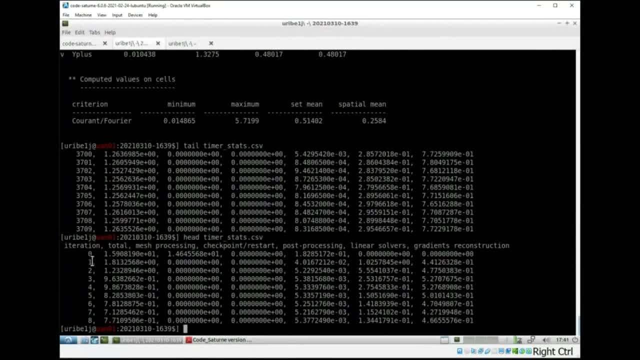 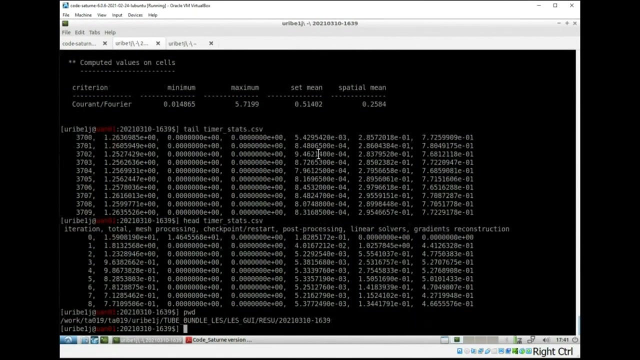 the number of iterations. so after you start you see that it's actually running and there is doing some iterations means that everything should be okay and you can happily go okay yourself. um, in your in your execution data that is also is here in your directory. so in my case it's this date, but you should have your own. 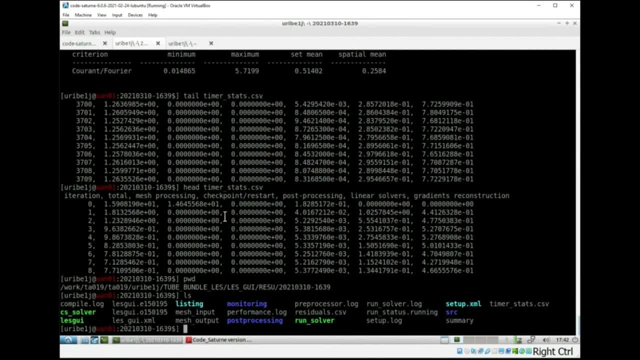 there's a file called statisticscsv- this one so- that gives you every iteration the total time seconds that it took and it splits it into all of these, uh, different stages of the iteration. So, as you can see, mesh preprocessing is only done at the first iteration and then zero. 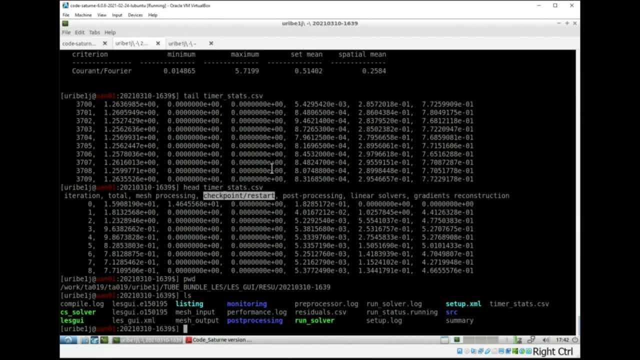 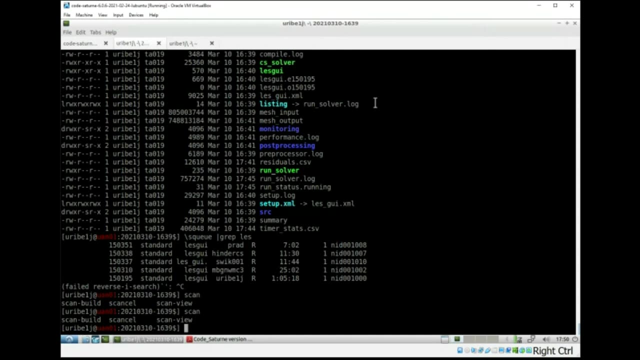 And the same for the checkpoint and restart. that's going to be done every 50 iterations or something. Another good way to check that everything is OK is looking at these two files, LESGYE and O, and then this number is going to be the number of the job that has the output and the error of what you would normally see in your terminal graphical interface. 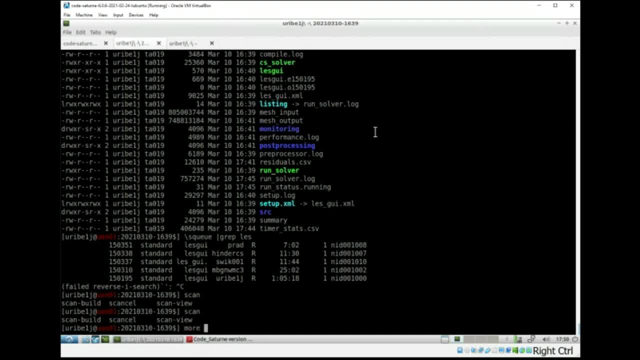 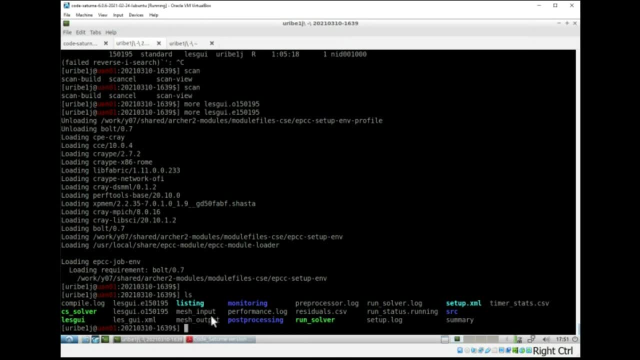 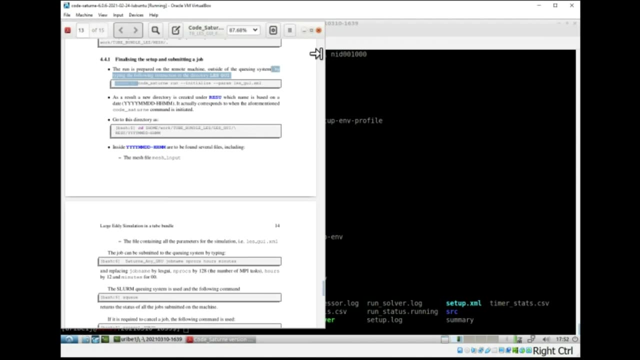 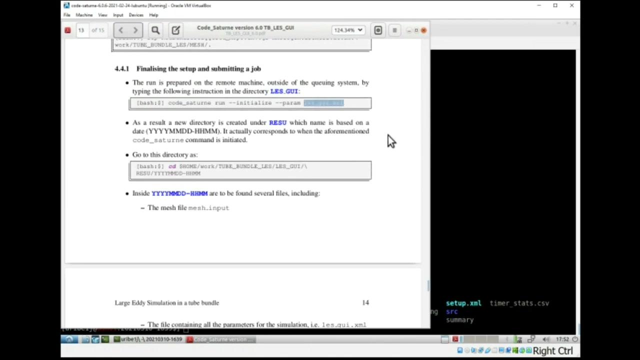 So if I show you mine, The problem is, I'll show you here. The problem is that there's three problems. There are two things. When you do the initialize this instruction, can you see it Here? this is the name of the data file that you copied from your GUI in your local machine. 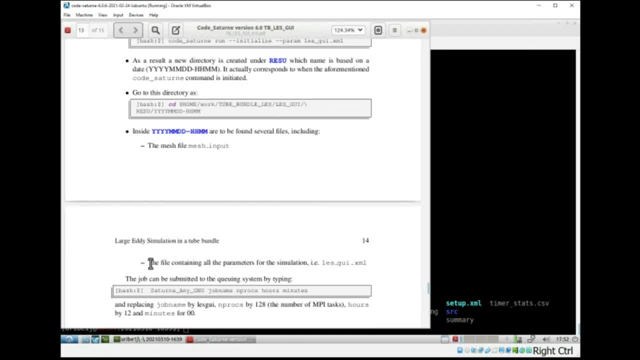 But then when you submit the job with this command here, SaturniGNU, this job name, it should be LESGYEE, Without the underscore and without the dot. So I mean, for some reason that wasn't what you had, but I don't know if it was because you submitted this one or 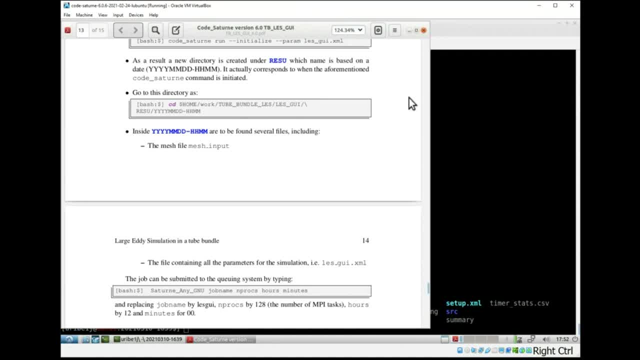 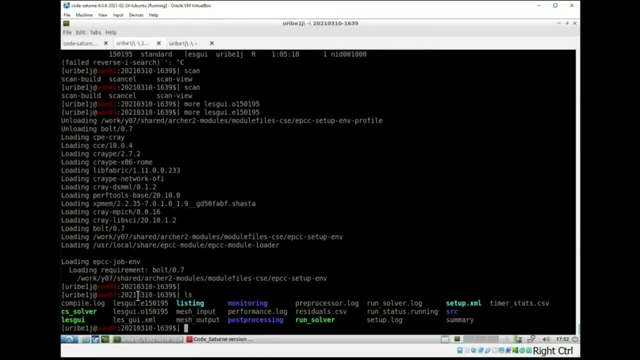 Yeah, I submitted the XML thing literally on the job name. I put that down as the XML thing, So it probably means that it overwrote this file, Because what that command does is create this file. The name that you put is a different file. 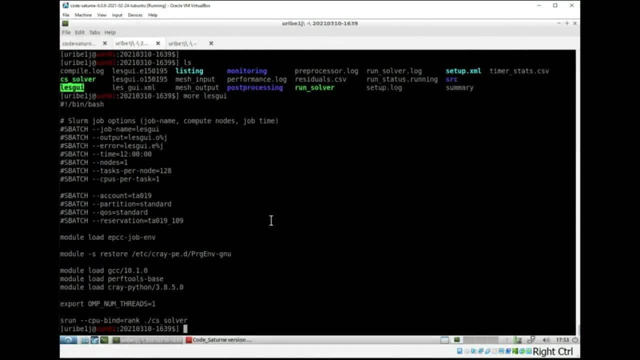 So you need both. You need the XML file and this new name file. So if you put the XML file in the submission script, it means that you overwrote the XML file. So if you look at your XML file, it should have all of this. 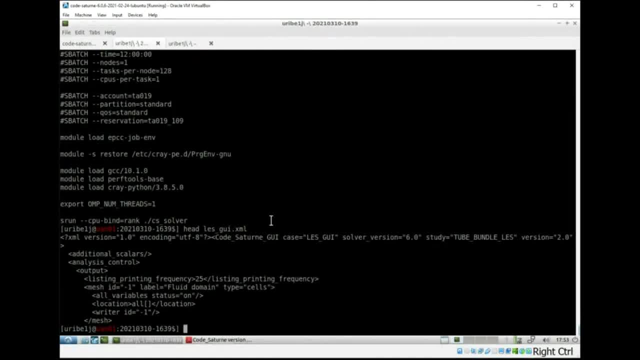 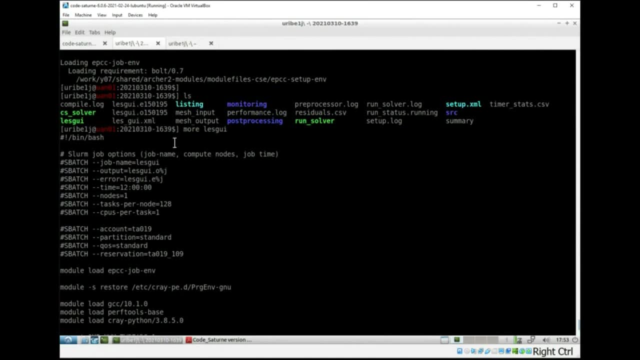 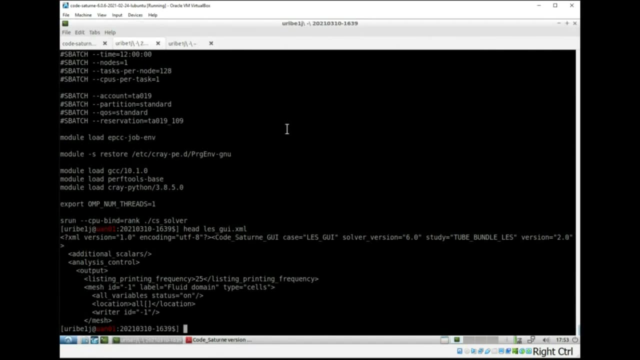 XML tags and stuff, Whereas the other one should have, like, shell commands. Did you do another initialize? Yeah, After you cancel the job. Okay, That should work. Yeah, I've got the statistics as per the one that you displayed. 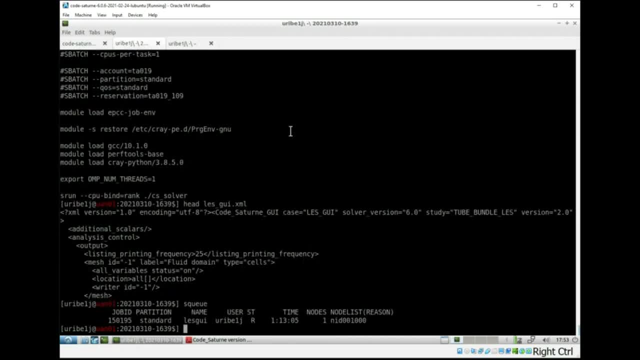 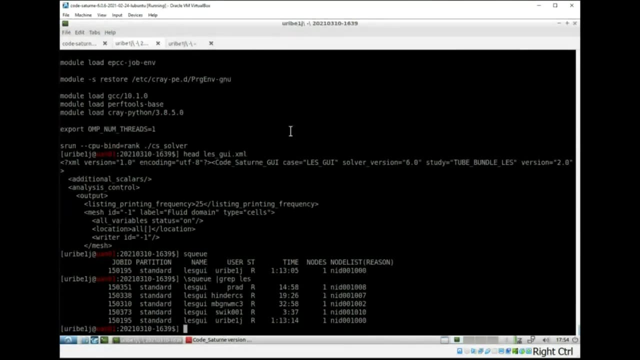 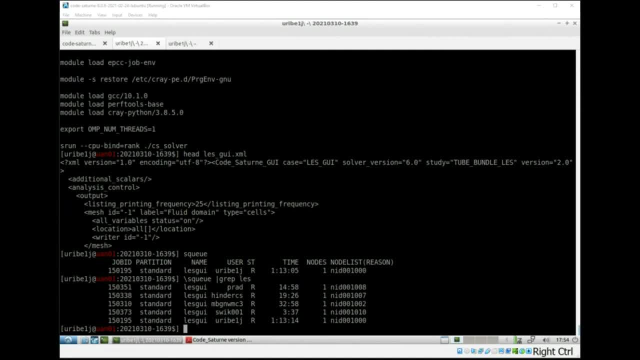 Okay, Okay, Okay. Who is he asking? Hello, how are you doing? I'm good, Thank you. I'll leave the علog to XANG then. Sorry, Apologies, All right, So do we just log off, or are we okay? 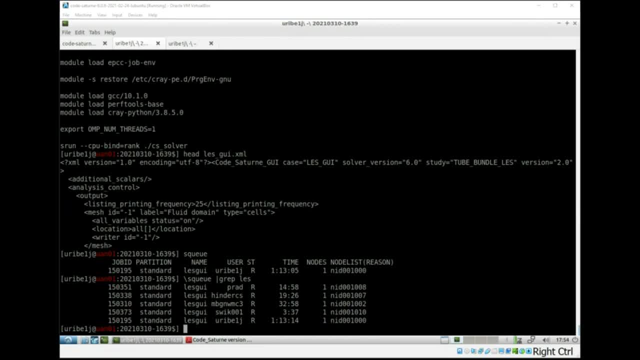 Yeah, yeah, you're done for today. Thank you for having us. Thanks, guys. Thank you. We'll talk tomorrow and in that case, that's great. Okay, Please, Bye, bye, As William is asking. so is there anybody who you had before that you moved your? 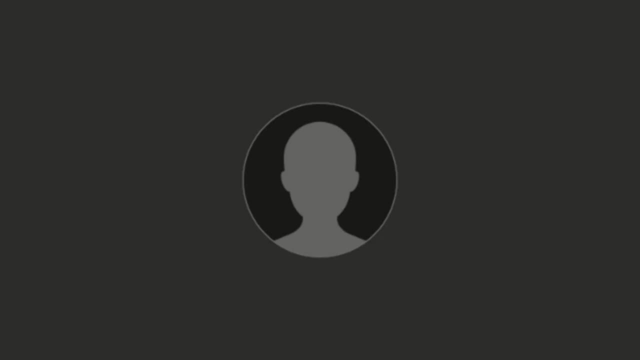 Red X signature. so is there anybody else having issues or is everything smooth going smoothly okay? so i mean, what i think is, uh, what you did when you created the xml file on the local machine. you basically went to look for a mesh which was not set or written or under the mesh directory. 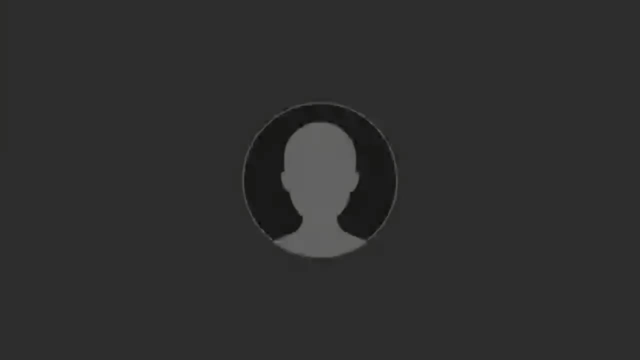 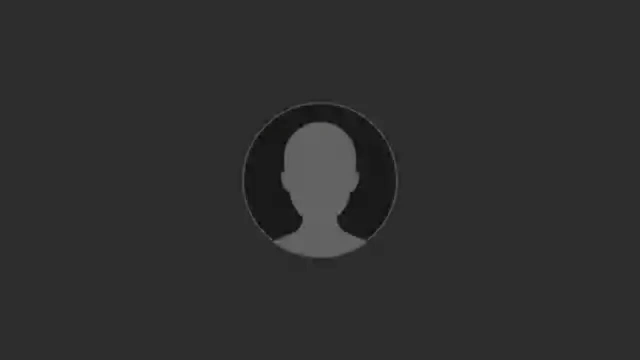 the to road bundle and the gz, but it has got the full, uh, the, the global path. that's what i think is happening. yes, so can we manually override the part in the excellent thing? well, if you give me a second, i try to find which keyword correspond to the mesh in the xml file. 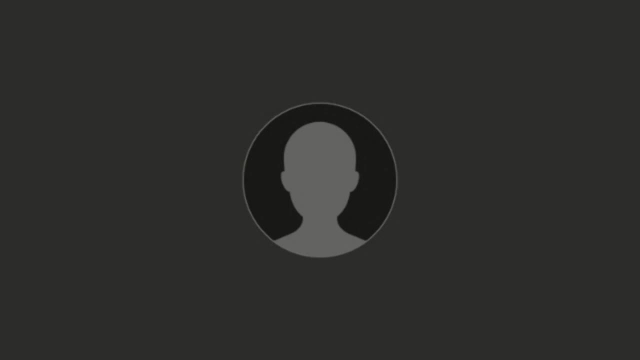 and i just send you the link. i mean, i just send you what, what to do, okay, so you could get very much. you could go to watcher 2 and the data, edit this xml file and there's just something to uh to change. but i need to find the exact syntax, okay, yes, all right, thanks, excellent. 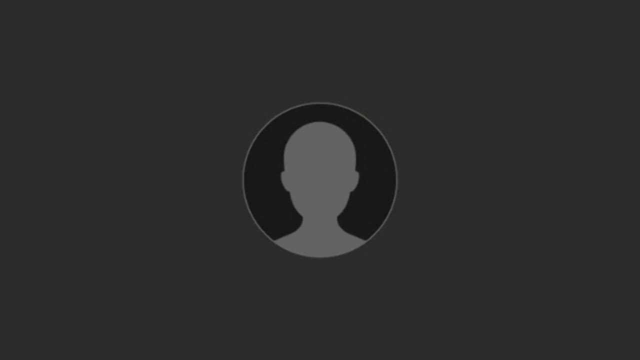 okay, can you? can you edit your xml file? and uh, on archer, uh two, sorry, in the data directory- i just found it- the path is stated to be the same. uh, slash form and so on. i need to change it, so okay, so mesh space name. that gives you. 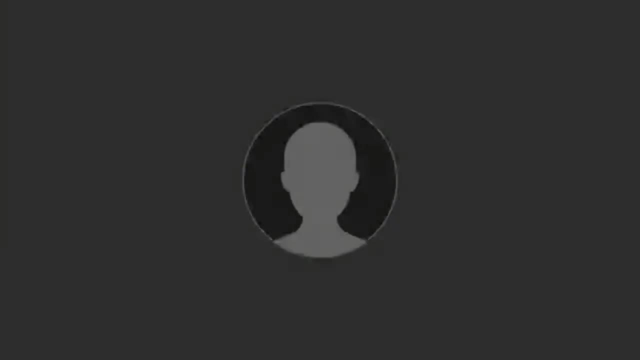 slash form and everything. yes, yes, uh, so basically i'll change it to my workday. no, no, no, no, no, no, no. you just delete everything apart from the name of the file, okay, you just delete, slash home everything and you just keep road bundle staggered on everything, okay.